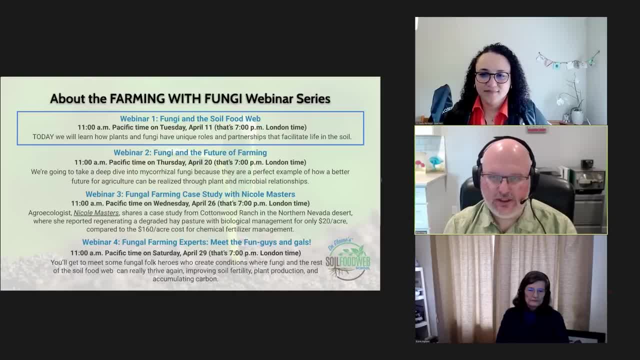 April 20th. This is where we're going to take a deep dive into mycorrhizae fungi, And then webinar three- Fungal Farming Case Study- with Nicole Masters. And then webinar four, which is going to be Fungal Farming Experts- Meet the Fun Guys and Gals, and that's going to be on April. 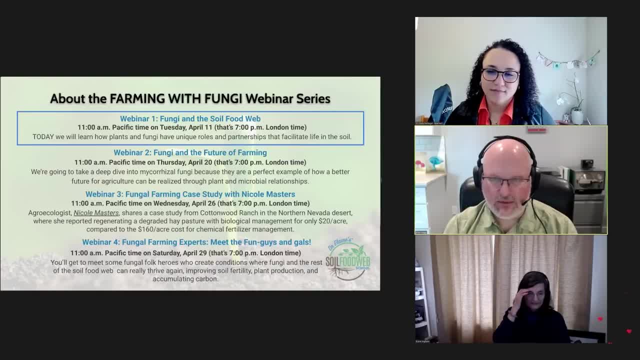 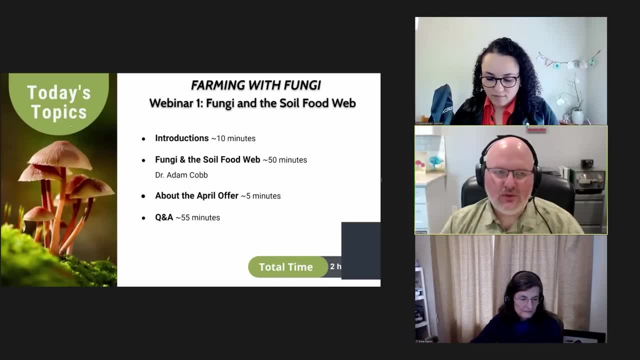 Saturday, April 29th. So we've got, I think, just a great April webinar series. I mean, I love fungi, so this is fantastic that we have it focused on. All right, let's get into who our panelists are for today. So, Elaine, you want to introduce yourself? 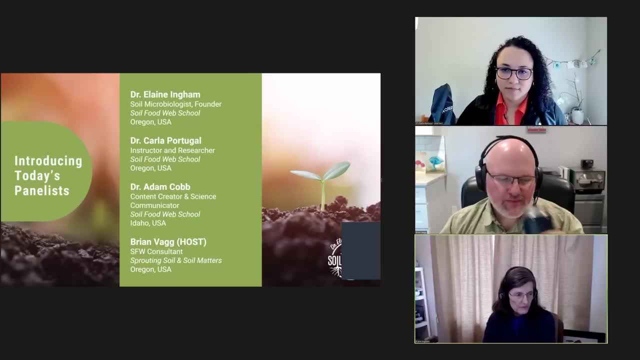 So I am the president of the Soil Food Web School. I also have a small consulting company called Soil Food Web Inc. So don't get the two of them. just you know, get them wrong. Don't keep them separate. They are different places. So get hold of me wherever you want. I started the Soil Food Web back in gosh. it's been since 1996.. Before that we had the Soil Microbial Biomass Service at the Oregon State University, But when I left the university started out on my own 1996.. That's when the changes happened, And so working on all kinds 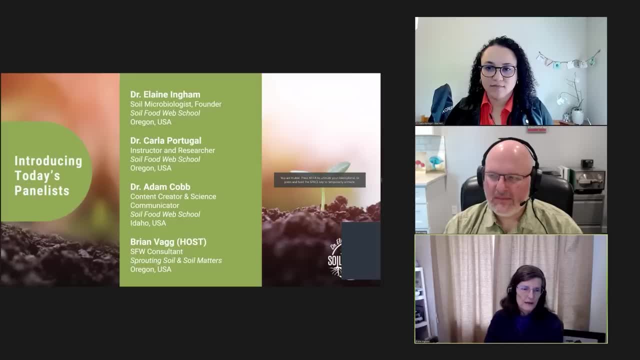 of projects all over the world, And so I've been working on all kinds of projects all over the world. It's fun having some time here to talk to everyone around the world about what they've been finding. Great Thanks, Elaine. Dr Carla Portugal. 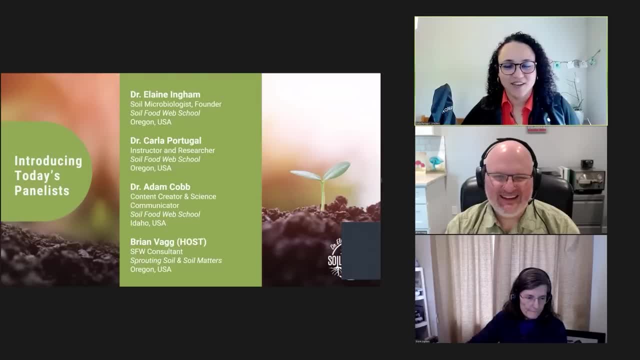 Hey, it's an honor to be here again talking about fungi, and it's always full of details. I'm excited for this presentation today. I'm an instructor and researcher at Dr Elaine's Soil Food Web School and I have the pleasure to work with this amazing crew. It's awesome to see that. 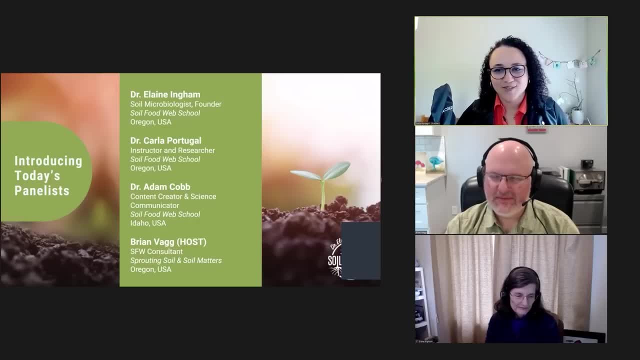 every webinar, we have more and more folks join us. So thank you all for being here, helping us change the system, changing the world. Great Thanks, Carla. Alright. Dr Adam Kamm- All right, Thanks for that opportunity, Brian. You all may have seen me on previous webinars. 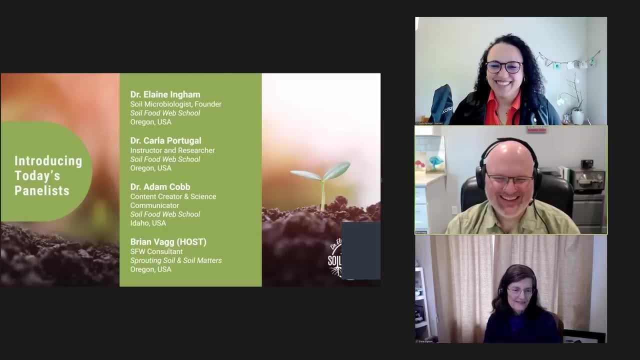 and you won't see me today on this webinar. webinar because apparently Brian, the internet, did not want two bald guys in this room. I guess not right too much shine. I get it exactly so, but I'm excited to bring the slide deck that I put together there's. they're very visual and since Brian is driving that deck, you all will get to. 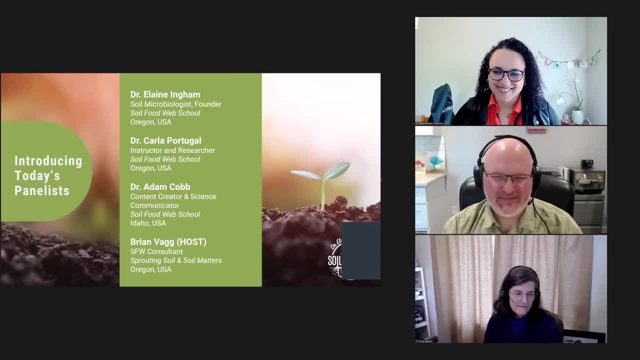 see it. you just won't get to see me today. I'm calling in from Idaho, where I don't want to make anybody jealous, but spring is in the air, the trees smell different, things are budding, things are blooming, and I could not be happier for for saying goodbye to winter. I hear you, I'm on the 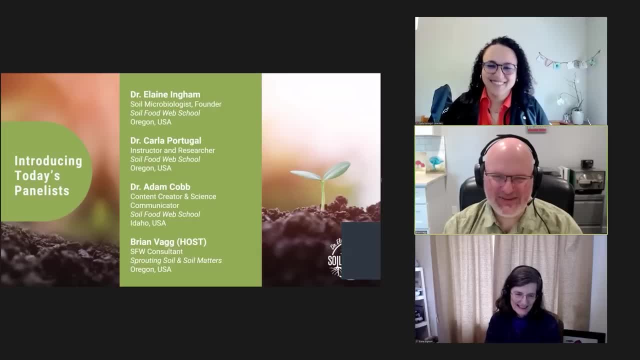 Oregon coast. it hasn't sprung in here yet, it's just been rainy and wet, so, okay, well, I'm Brian, I'm your host for today. I'm a soil food web consultant. I really have two businesses. I have sprouting soil, which is a consulting business, and then I've combined forces with Akisha and Casey. 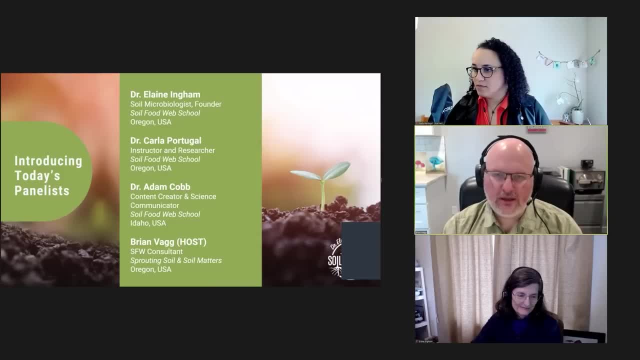 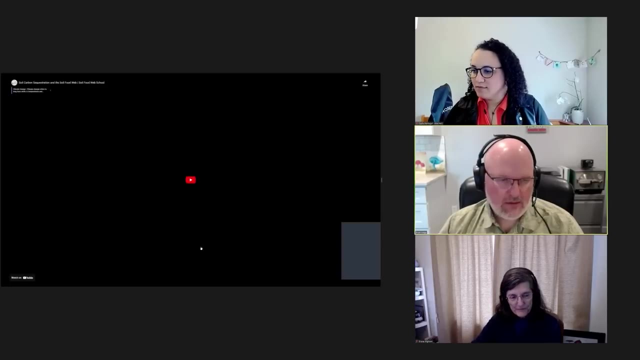 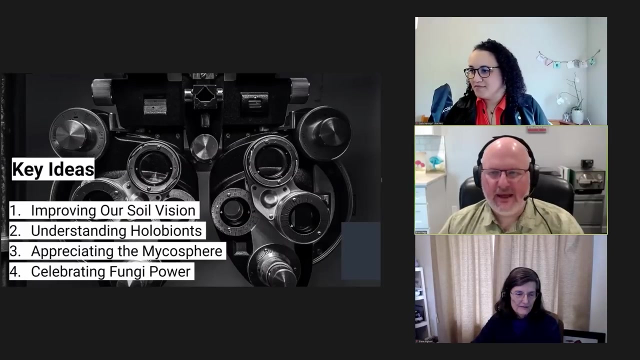 Ernst, who some of you may be familiar with, and we've created a larger consulting group called soil matters, and I'm based out of Oregon, USA. all right, without further ado, let's go ahead and jump right into your presentation, Adam. actually we're gonna skip this video and go. sorry folks, there we go, Adam. 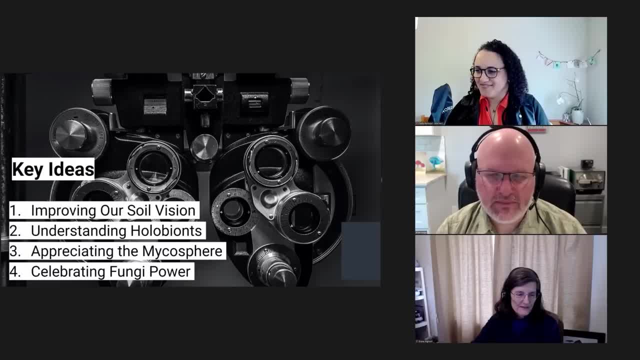 take it away. hey, there we go. now, Brian, you're gonna have to let me know if my audio quality changes drastically or something. and I can repeat myself, because again, this is a phone call and, Adam, your auto quality is perfect. it's really really good, excellent, that's good to. 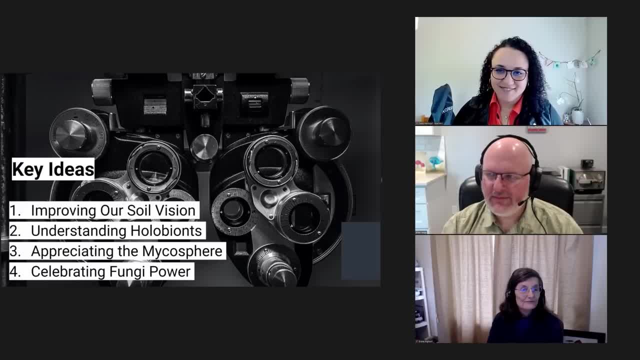 hear- and Carla and Elaine and Brian- all of you- this is, this represents teamwork, so you know any of these ideas it's because of being in this place for a year and a half, so I want you all to to jump in and add things to my talk as we're going along. and, Brian, since you're driving, you can just tell. 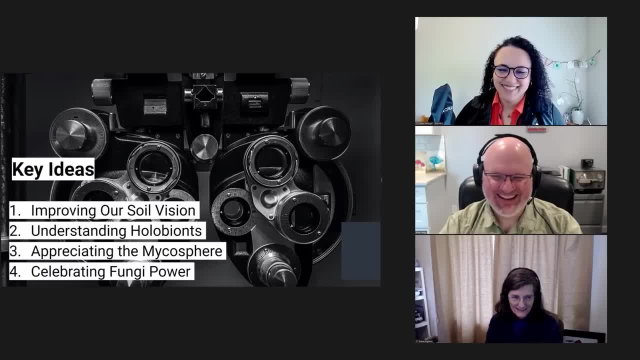 me to shut up and let these amazing, brilliant women add what they want to add, or you can add what you want to add. we're not afraid of adding our opinions here at this group at all. so I know it's a great quality for sure. so, um, this time I, I did. 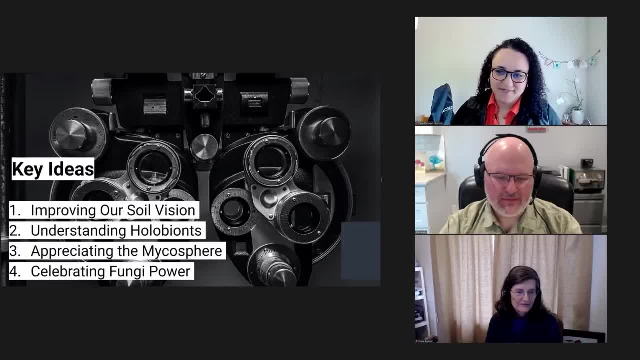 something a little different and I actually wanted to list sort of the the four key points of this talk or key ideas. um, and I just want to mention, you know, I started with saying improving our soil vision- because my personal story is one across the last 15 years where I have just reached for every opportunity that I could. 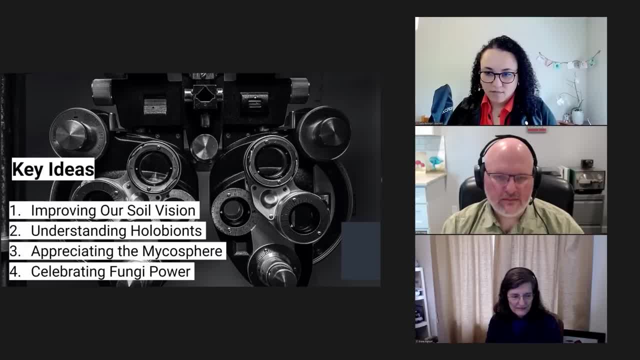 think of to improve the accuracy of my soil eyes. right, it's like going to an optometrist and saying, is this better or this? is this better or this? and every piece of information, every opportunity to have a conversation with the people in this place, um it. what I want to do is see the soil story. 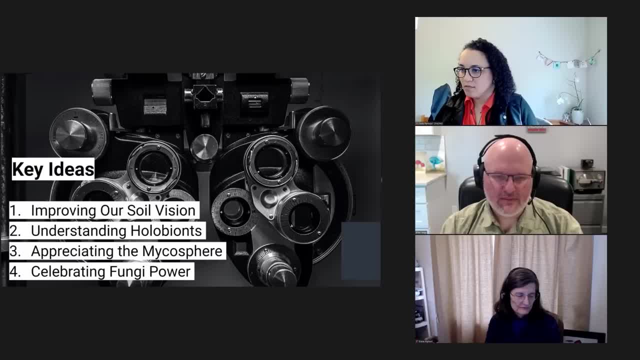 bring, or translate, some of my lessons to this group. To do that, I want to spend some time today focusing on the concept of what's a holobiont. I want to bring that because I think it's not only the exciting thing that's made our planet, it's really the planet belongs to the. 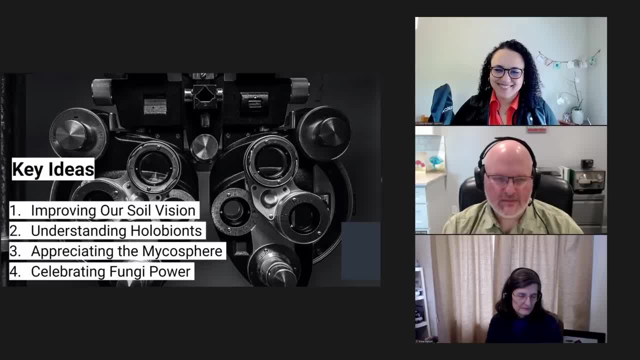 holobionts and we're just passengers in my opinion. But it's also the future of agriculture, which we'll get into more next time. And then I want to focus in on what I call the micosphere, or what many people call the micosphere right, And define that and explain. 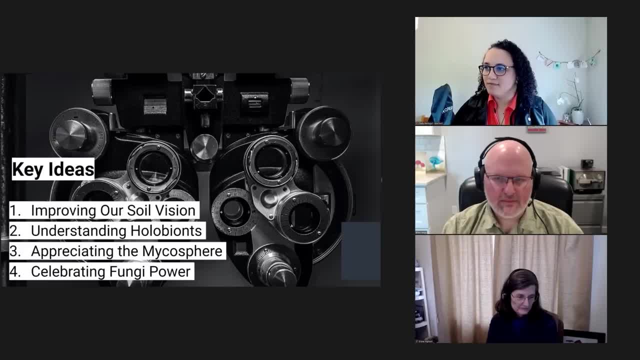 how fungi play this unique role, but this role in an ecosystem with all these other beautiful relationships in the soil food web. And then I do want to spend some time just celebrating fungi power. They are one of my favorites and I think that appreciating them and I think that 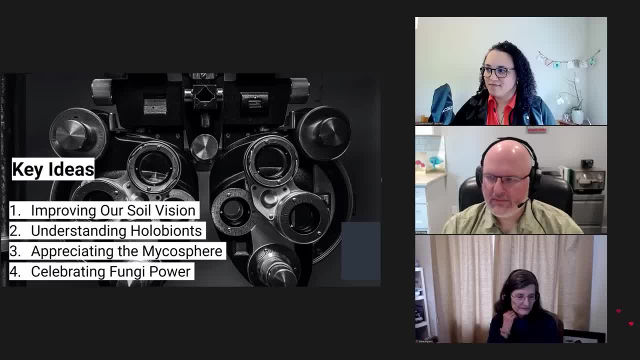 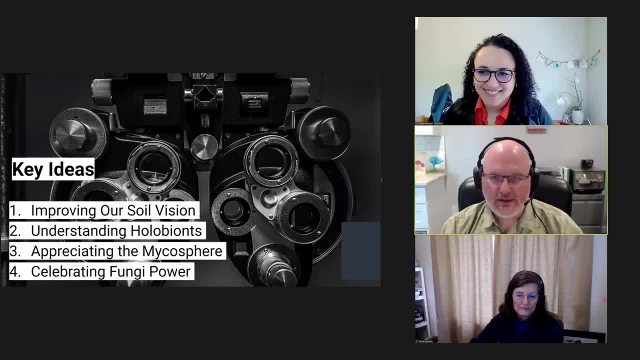 analogy of the soil vision, And you know, it's to say from my own experience, that as my knowledge base is increased, plus my the tools I have available to me have become available, that my vision or acuity of understanding really what's happening in the soil is definitely increased. 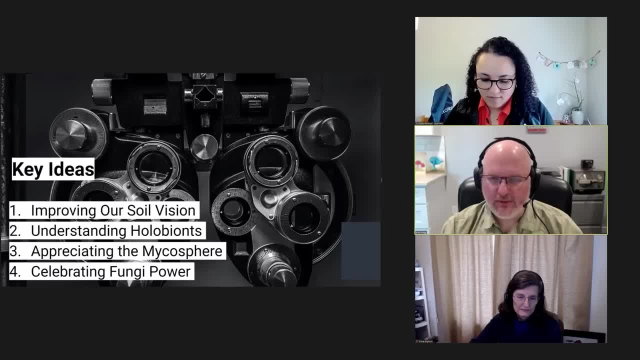 And it continues to. So the analogy really stuck home for me Right on. Some people call soil black box. They use that metaphor because as much as humans are peering into it, as much as we have developed across, especially the last 100 years, the science, 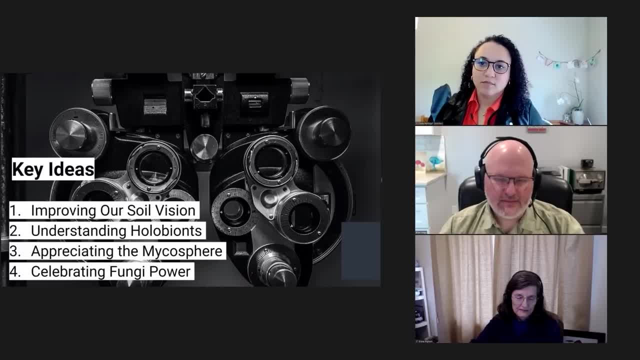 and the tools. we still have to remind ourselves to be humble, because there's so much of it that we don't understand yet. But together, this community is trying to illuminate into that black box, And I think that's a really good point. And I think that's a really good point. 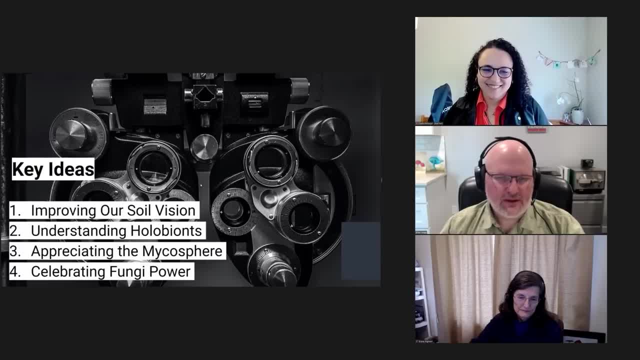 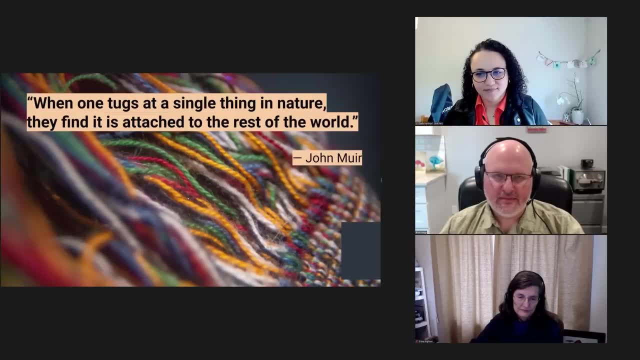 But together, this community is trying to illuminate into that black box, And I think that's a really good point, And I think that's a really good point, And I think that's a really good point. Great, Next slide. Yeah, this is just one of my favorite quotes and I think it's really appropriate to discuss. 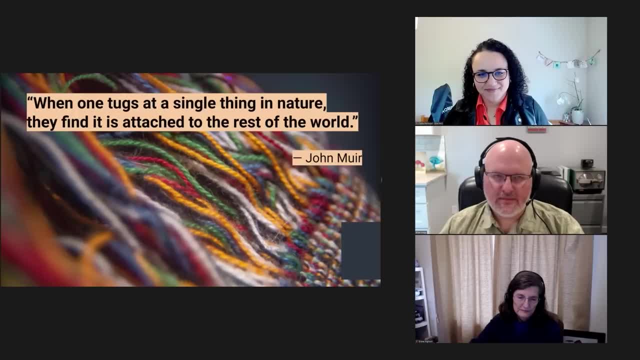 fungi that if we start tugging at one thing in nature, we'll find that thing attached to everything else Right. And fungi are such a critical component of the tapestry because their connection right. they connect things that normally wouldn't be able to even communicate or share resources or have a 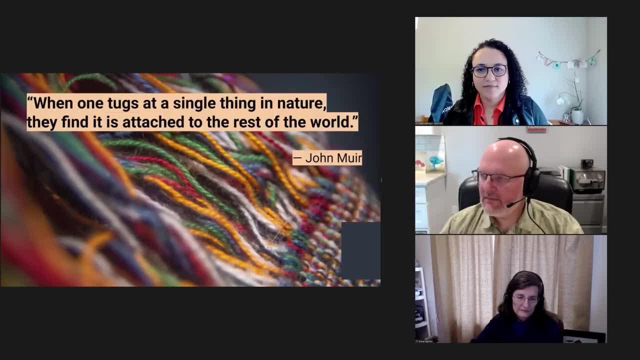 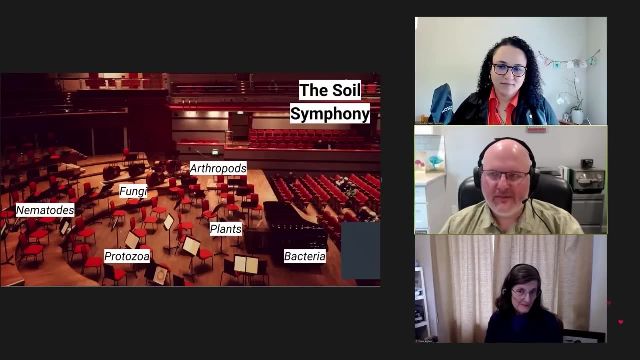 relationship. They're like I don't know. it's sort of like they facilitate the dating app of the microbial world, right, Help people link up Next slide. Yeah, sure, Okay. I worked on this with Dr Lane. We had a lot of fun and talked about how we need to get a cartoonist in here. 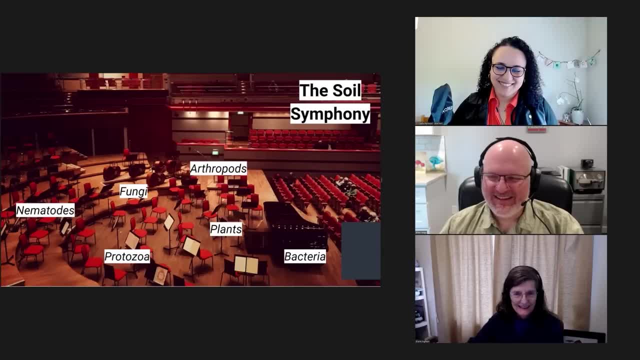 and really make this a cartoon in the long run. But you know she shared during our last soil summit a talk about this, the symphony in the soil right, the way that things are brought together, And please note that the plants we've put there kind of at the conductor's spot. 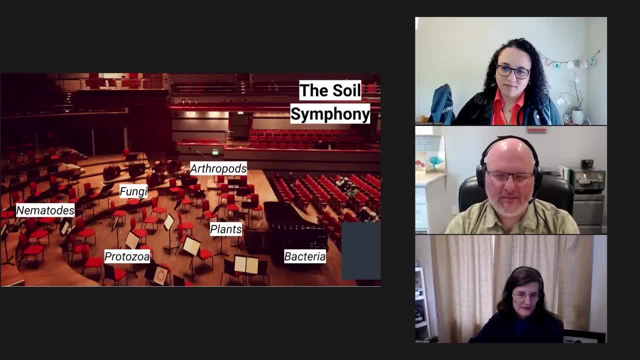 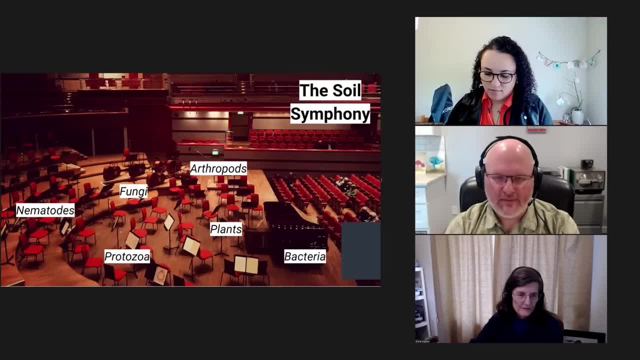 food web community. it's like the violinists, and then over here's the drums, and then the bacteria are playing the piano. And if we step back and say we get to have some influence as humans, we get to be one of the keystones of the system, we can make you know a lot, of a lot. 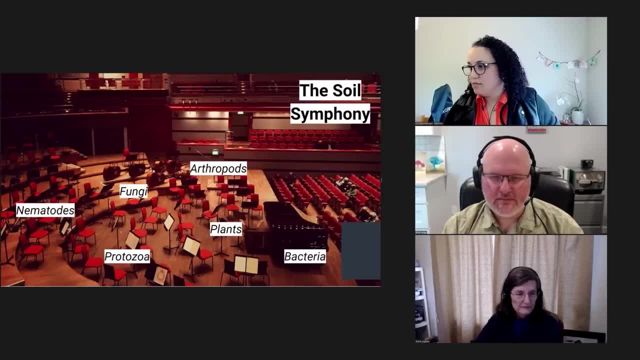 of impact on the system. But if we trust the wisdom that's embodied in how these relationships evolved and we try to emulate and support the symphony that they already know how to make without us, then we get to. you know, I would. I would bring in a concept from Nicole Master's book. 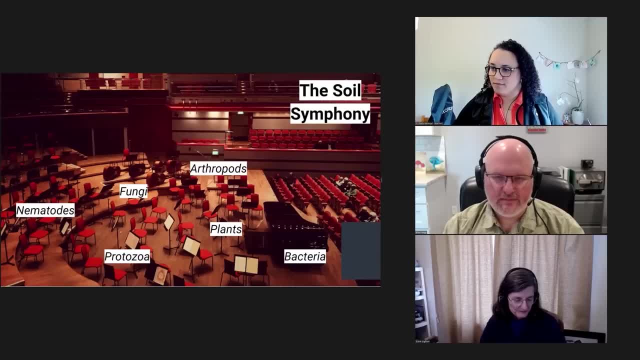 we get to tickle the system a little bit, we get to add a little bit of extra power into this, but it's not our role to be the engineers or the micromanagers of the soil symphony. we have to trust them. 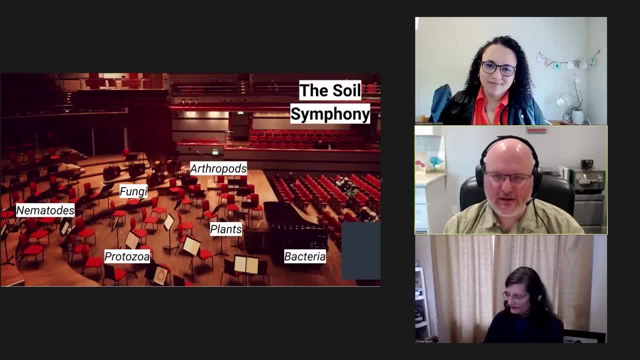 It's almost like we're the general manager of the symphony, right? Just making sure that all the players get there Exactly, And then sit back and enjoy the show. Right, A lot like the leader of the, you know, the orchestra stands up and keeps the time, but 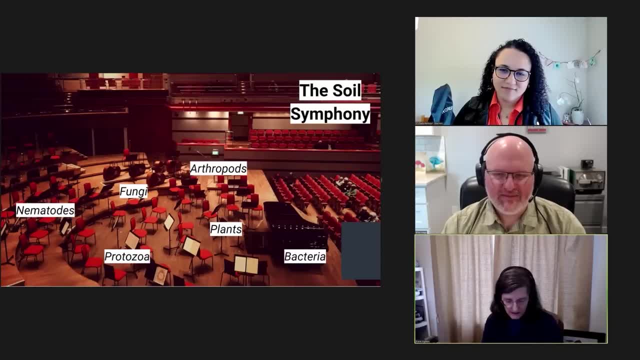 different processes are done by different parts of the symphony And it makes it so different. if you add or subtract, Right, And it's it's, it's a different instrument as compared to another. It's almost a completely different symphony, Mm hmm. 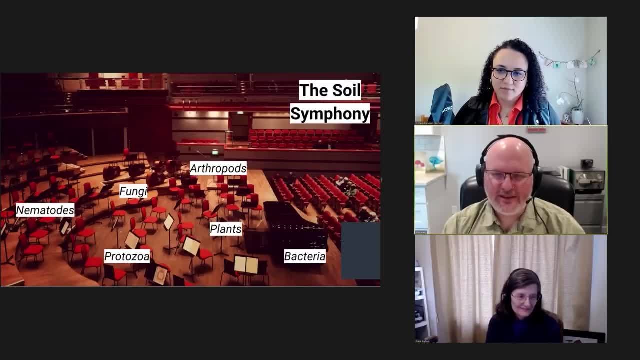 Yeah, I wouldn't want to try to farm without fungi. Yeah, because I'm sick for the day. The protozoa took over Exactly. This is another really good analogy, I think, Adam. Oh, thank you. Well, I think you know, Elaine and I have to share credit for that one, because 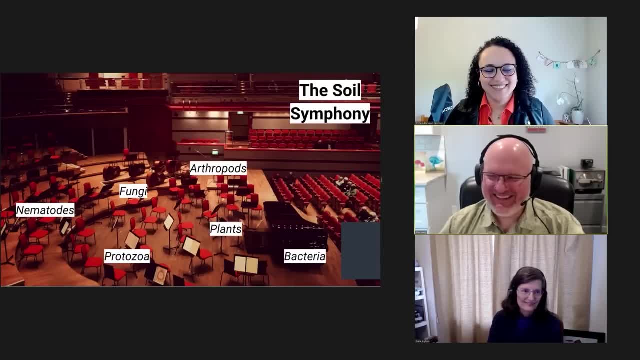 from one of our wild conversations that we have, where we have a lot of fun thinking through how to how to communicate this, and there's a disc from gosh. it must be 15 years ago now where the symphony of the soil was talking about how all of the this life in the soil interacted. 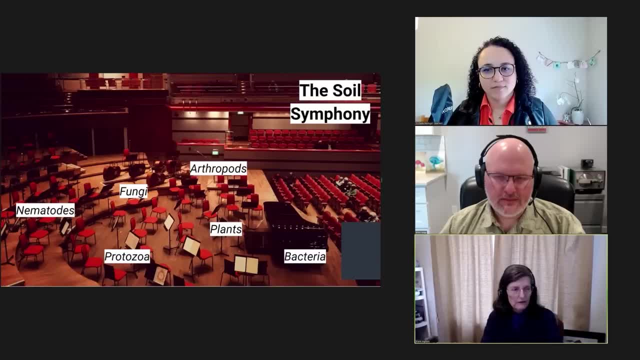 with large industry or small scale plots, or you know, large farms to ginormous farms and all of the pitfalls, as well as the fact that we could deal with everything and get it back into the right place so that human beings could survive upon this planet. all right, next slide, yeah. 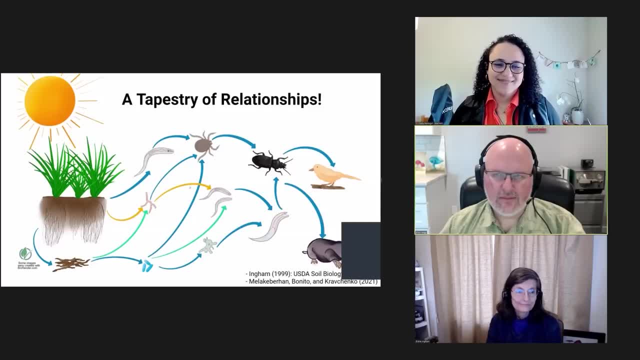 yeah, yeah, okay, this is another representation where we're actually zooming in on the tapestry of relationships in the soil food web. um, we haven't put a lot of complicated labels here, but i want to, you know, say that this really starts with this magic that happens. it's the 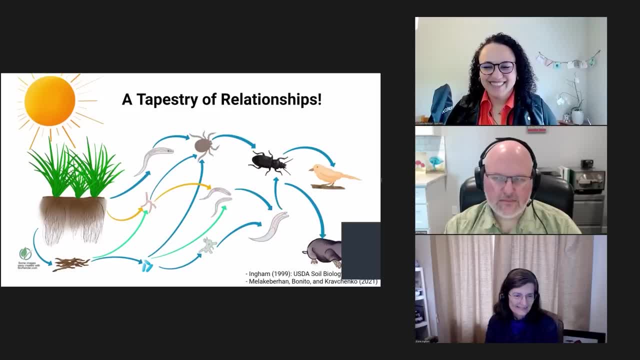 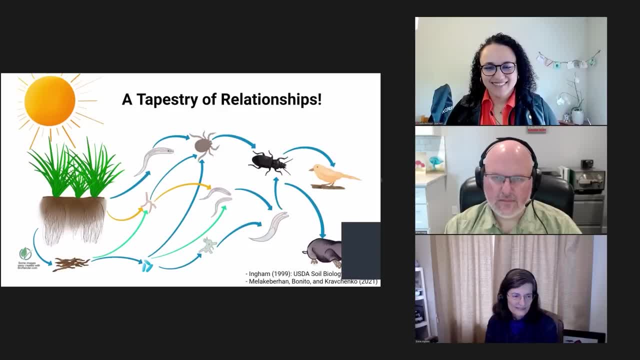 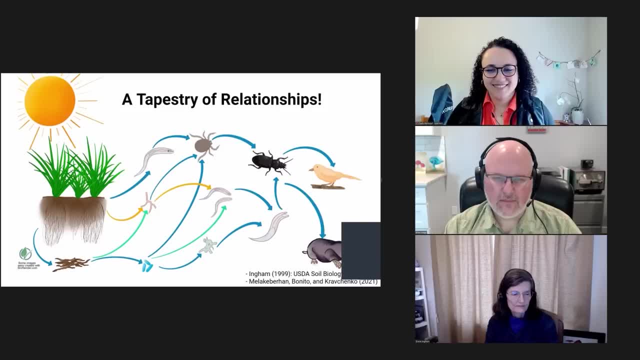 exude it from their roots. we call those exudates. they share that liquid sunlight, that carbon that they've made with the things in their rhizosphere, in that area of soil that's in close proximity to the plants, and so we start to see that bacteria and fungi will be attracted to this place, where 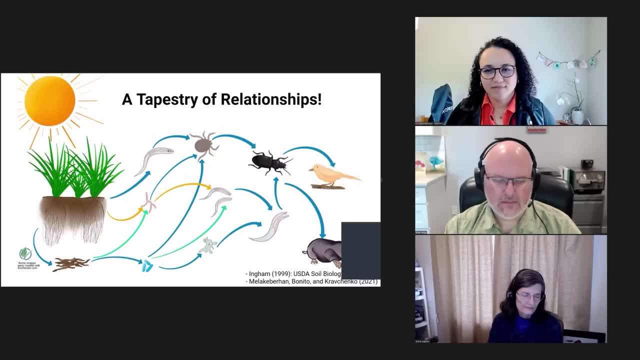 sugars are available and that that will feed them and fuel their reproduction so that they can harvest minerals that they need from the soil system. and then, if the story stopped there, it would be not enough, because the bacteria and fungi would just hold all the nutrients, but eventually the fungi can be consumed by arthropods, which a lot of times we call. 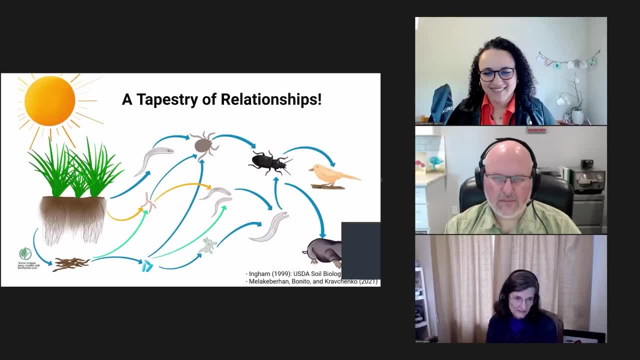 micro arthropods and certain kinds of protozoa and nematodes are feeding on fungi and bacteria and they're releasing those nutrients right by the plant roots so that they can help the plant achieve maximum efficiency in photosynthesis. the magic is taken to a whole new level of 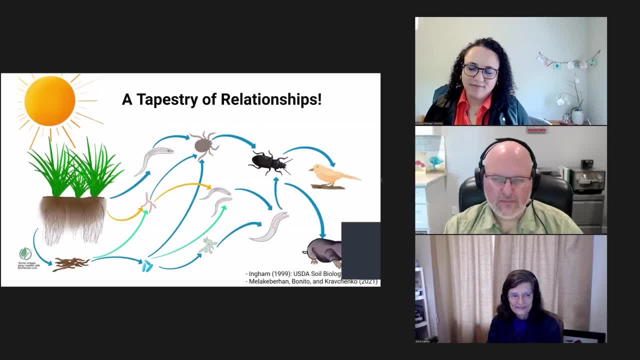 power, and that means even more carbon can come into the system, even more sugars, and then it builds, and it builds, and it builds. then we have higher level organisms, larger arthropods, predatory nematodes, even birds and moles and other things that help prune the soil food web. they help take out things that might be problematic, that might cause disruption. 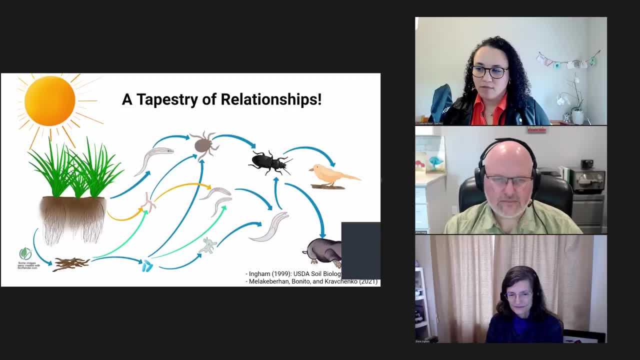 or disease. they help balance the relative biomass of these different groups, And so, again, we can sit back in awe of this. If you go to a tall grass prairie in the central US, you will see a system that doesn't really need a lot of help. Humans can come in and maybe with some fire or some other management. 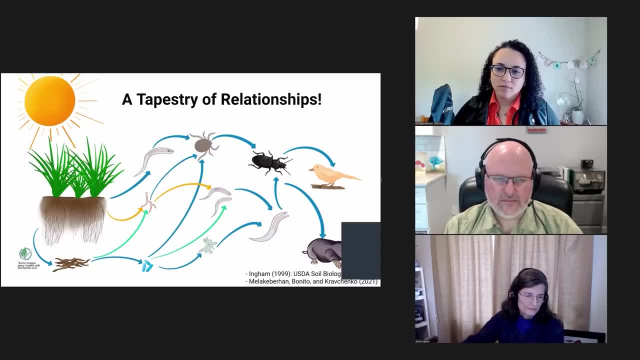 they can help that system Again. they can tickle it and get it to maximum, but it's the bison and the voles and the nematodes and the fungi that are really driving the productivity of the plants And in turn it all just cycles on itself. Did I miss anything? 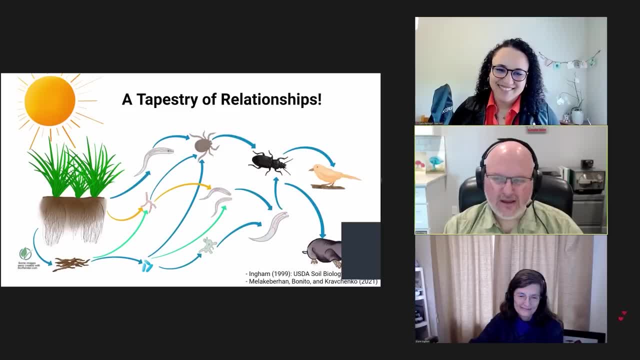 No, I think there's a testament to this particular visual, because, Elaine, you created this in 1999, right, Yeah, thereabouts, Yeah, And it's. I mean, if you just look up Soil Food Web, you're going to find this. 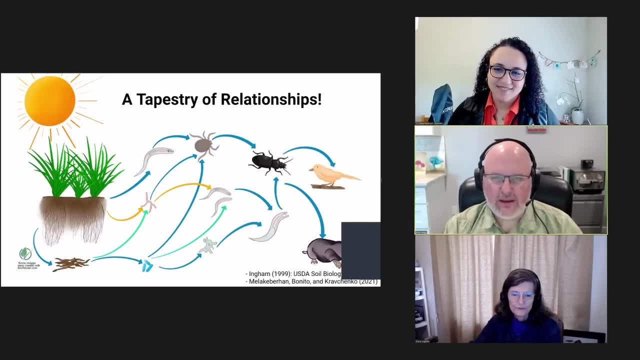 diagram. It's some shape or form, but it's definitely stood the test of the time. There's not very many images that can last 20 some odd years, or graphics like this that still have that kind of that punch, And for me, when I talk to my clients or I'm teaching any kind of workshops, 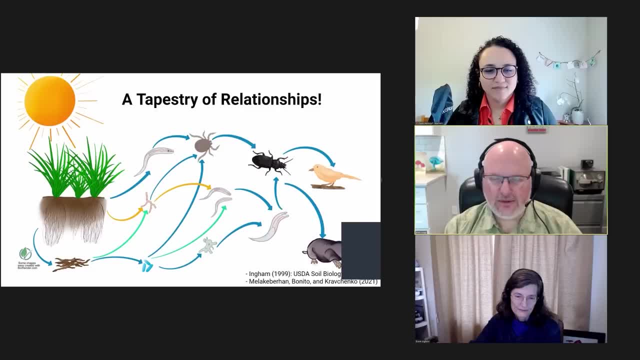 this is usually slide number two or three. It really described the Soil Food Web such an elegant way to be able to do it. Yeah, In fact, when folks know that we're talking about Soil Food Web, they expect to see this tapestry. 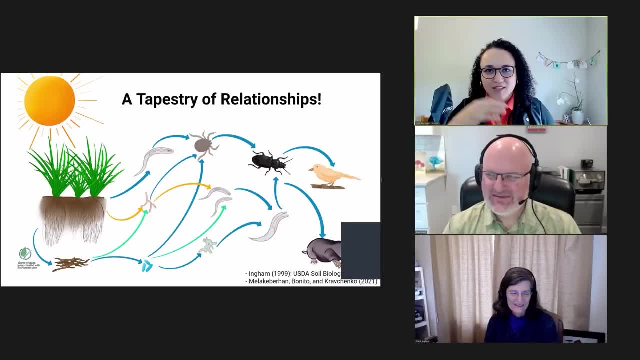 Yeah, It's beautiful to see that other folks are just basically shifting colors drawings, but the main message stays the same And connected with what Adam said. this is: what drives my passion for science is how much we can, just along the years, validate the concept over and over and continue. 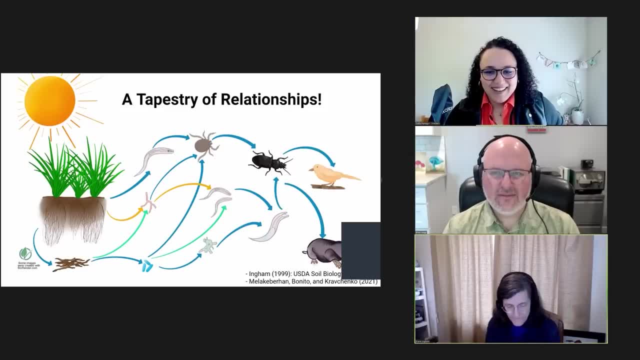 developing at the same time, But we still, Sorry, Go ahead, Sorry, Sorry, But we still have to figure out how to do it. But we still have to figure out how this interacts and changes things above ground, Precisely. 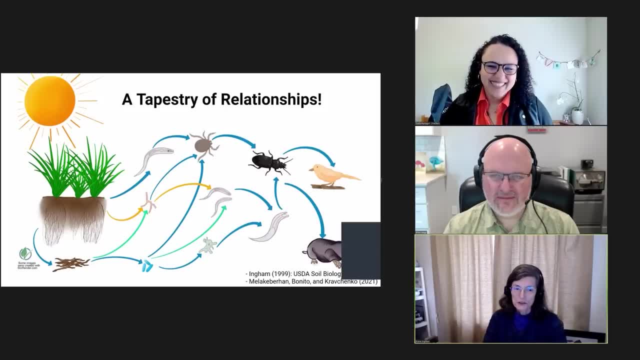 Because there's a whole nother tapestry of relationships and we've got to merge them together. We can't stop now, Exactly, Absolutely. And Brian, could you do me a favor Because Carla has got me inspired. Could you point out that orange arrow coming from plants in particular, and to the fungi there, Carla, what you 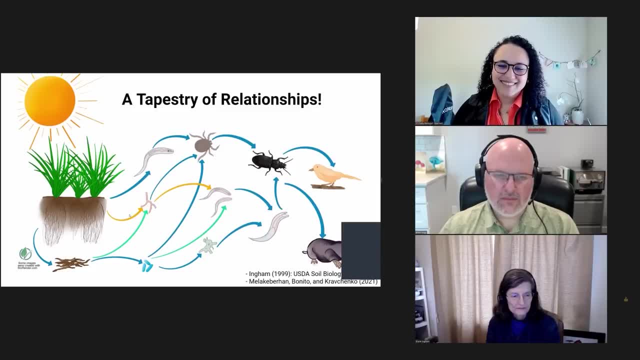 said about this tapestry reminded me that, Yeah, Yeah, It reminded me that for so long, when I was in academia and a researcher, I got really, really focused on one arguably very important relationship. that was our muscular mycorrhizal fungi, and especially with grasses, because it's so critical and we can see 600% more growth when 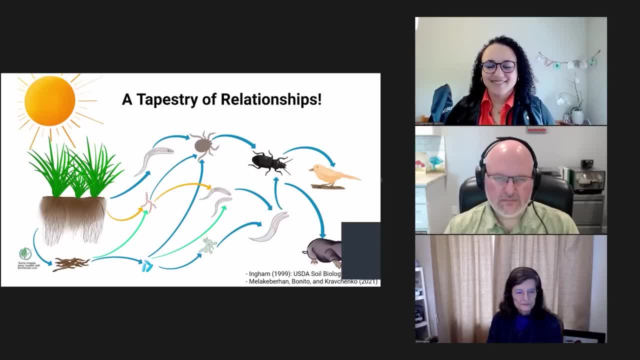 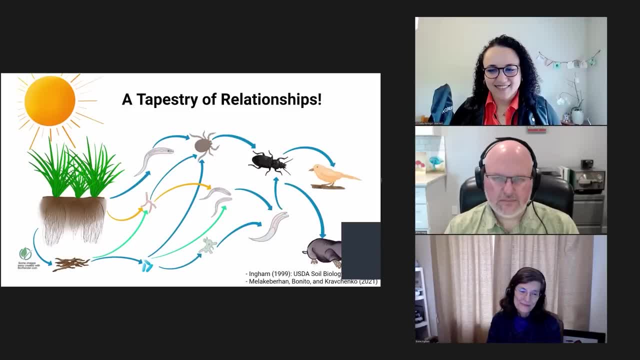 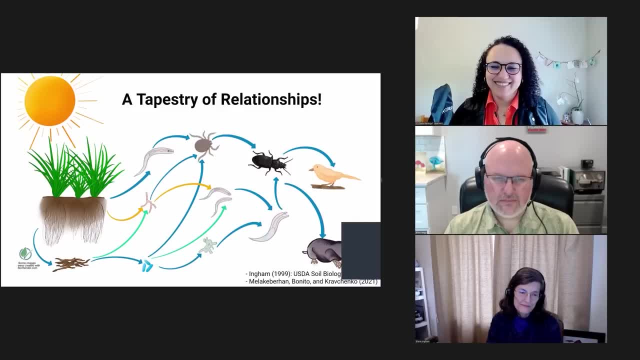 want to blow anybody's mind, except if we were to show you a real soil food web, the connections would be: you know, thousands, right, Because it's that we put these into key functional groups so we can talk about the patterns. but 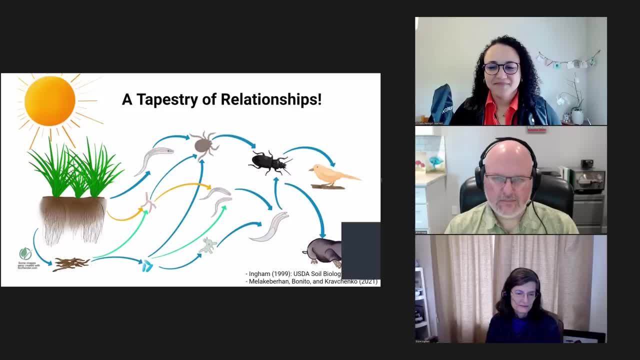 there's hundreds of species of mycorrhizal fungi alone in most areas of the world. the world right, We do. you know. people even argue about what a fungal species is and I can't get into that today, but we often see 14 or 15 different taxa, different types of mycorrhizal. 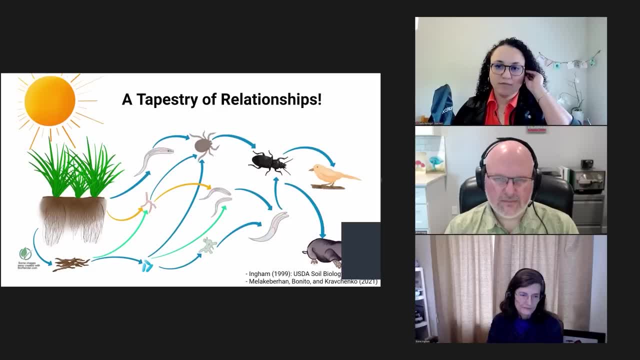 fungi in the roots of one plant, right All along that root system. there's different conditions, there's different relationships, there's a different interaction web of interactions happening so that that plant, all along its root system, can have the pH or the access to zinc or 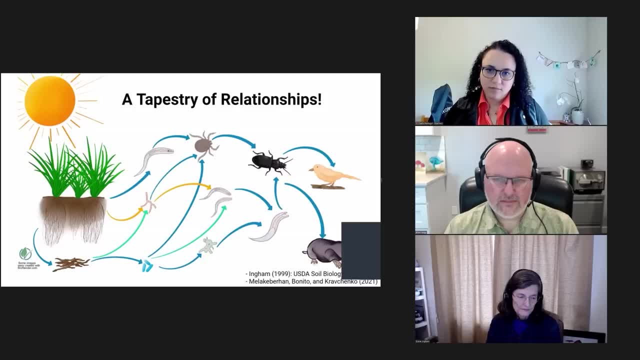 the access to phosphorus that it needs. It's the conductor of this beautiful thing, It's the starting point of, it's the loom that starts weaving the tapestry together. You know, one of the things that always strikes me, too, is this visualization here of a tapestry. but what's amazing is you take your microscope and you actually look. you're really looking at the tapestry and you're like: oh, this is the tapestry. You're looking at the tapestry, You're looking at the tapestry, You're looking at the tapestry. 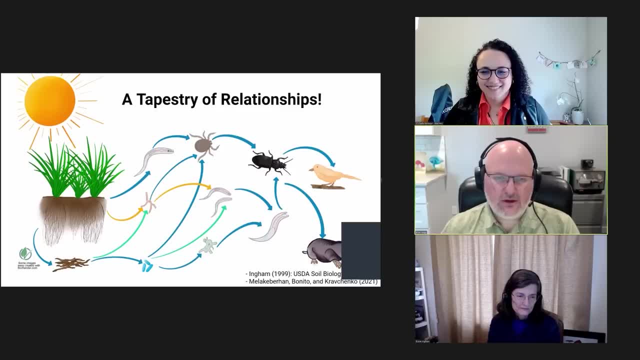 You're really looking for that tapestry And it's amazing to me that you can really take a look at a soil and say, wow, it's missing major parts of this tapestry, It's not nearly as vibrant, And then, when you get to a soil that has, all you know, a really highly functioning soil food web, 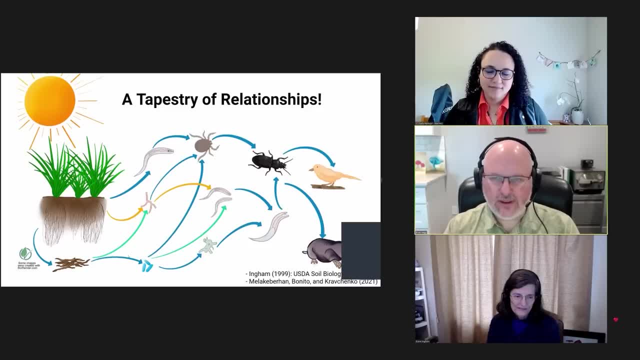 and this tapestry is alive. it really is visually there, You can observe it, and the microscope is definitely a great tool to be able to do that kind of work. Okay, we better go on, y'all. I could talk about this all day. 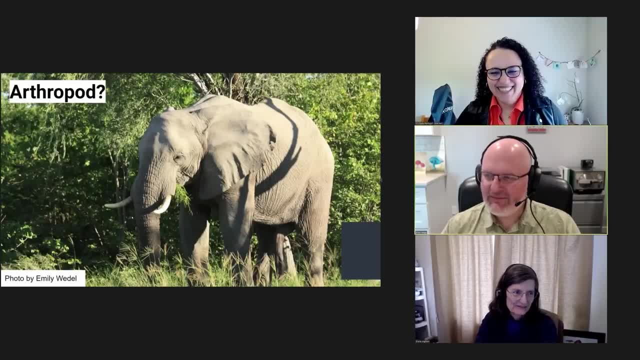 Yep for sure. Next slide. Okay, this is a picture that my friend Emily took when we were in Botswana on the Ogavenga Delta, which is one of the most biodiverse regions in the world, And I just love elephants, love watching them. We did have a matriarch charge our vehicle. 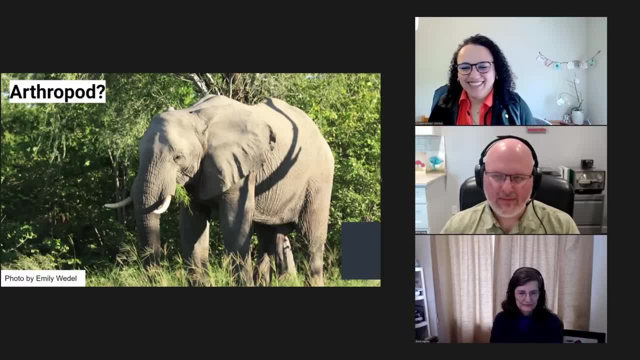 and that was scary. But I've put up there a funny question. It's not a real question, but you know this is not an arthropod, But I'm always looking for a visual that we can see without a microscope, that can help us improve our soil vision for what's going on at the 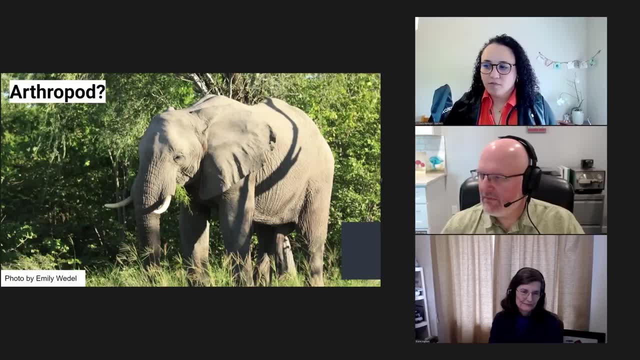 microscopic level, And elephants are keystone species in their ecosystem. They're ecosystem engineers. Just because they need to eat so much, they create different habitat, because they have to tear down trees and eat them. Well, a lot of times when they go into a forested area, you don't get. 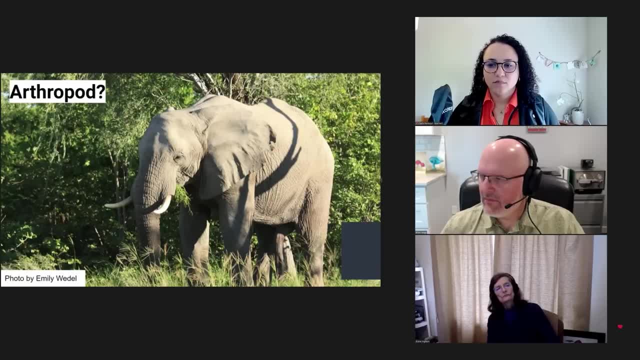 you know destruction, You get space For new things. it starts, they start to establish an ecotone, a savanna where grasses are thriving and trees are thriving, And the trees they leave behind often have more access to sunlight. 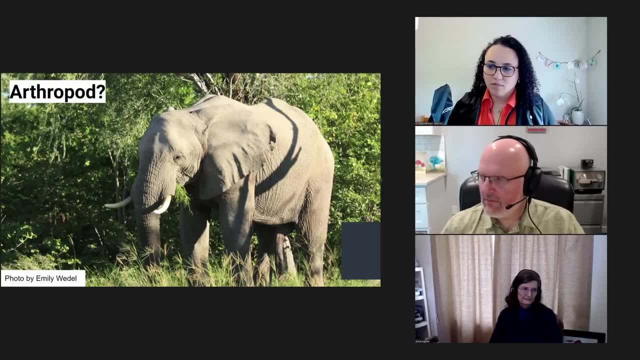 and more room to be healthy and more water or nutrients because of the action of the elephant. And so in my next slide I want to put in, I want to show you one of those functions that happens in the elephant. So I'm going to show you one of those functions that happens in the elephant. 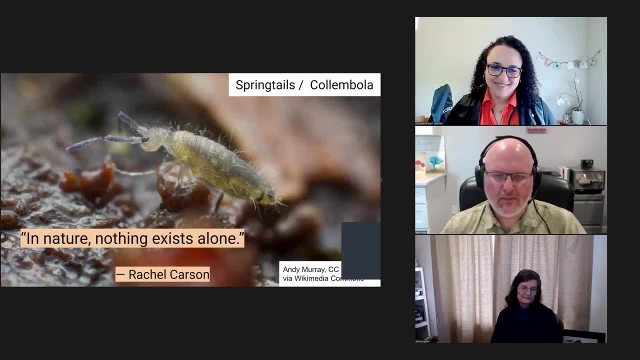 So in my next slide I want to put in, I want to show you one of those functions that happens in the elephant. So in my next slide I want to show you one of those functions that happens in the soil ecosystem, These little guys called springtails, kalembola. there's many species around. 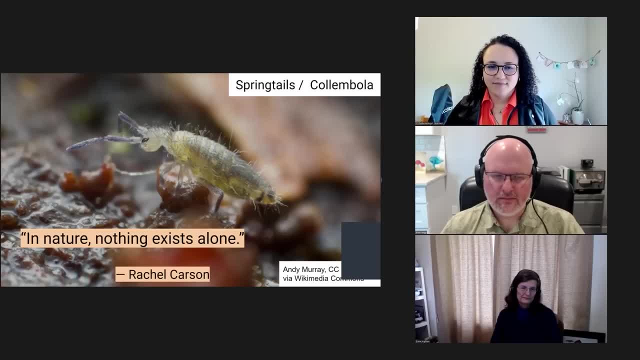 the world. I think of them like a microscopic elephant And they mostly feed on fungi instead of trees. But we don't want humans, you know, who are looking to have these systems be productive and support livelihoods and keep us all alive because we have to eat. We don't want certain 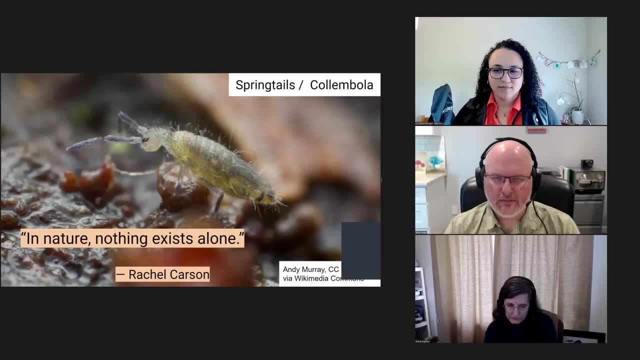 fungi to get out of control. We don't want them to be in the soil ecosystem. We don't want them to be. There's kalembola in some research i've been reading lately, when they're given access to a diverse community of soil fungi, they prefer. 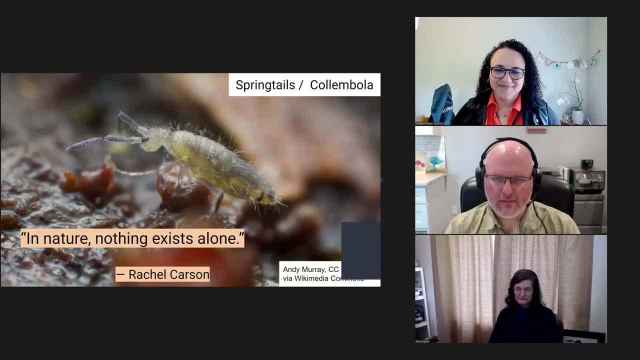 to eat the disease-causing fungi or the potentially problematic fungi. They prune the fungal forest and help reduce or control the dominance of fungi that could be a problem, And so So the ones that really help our plants grow bigger and provide all these other ecosystem. 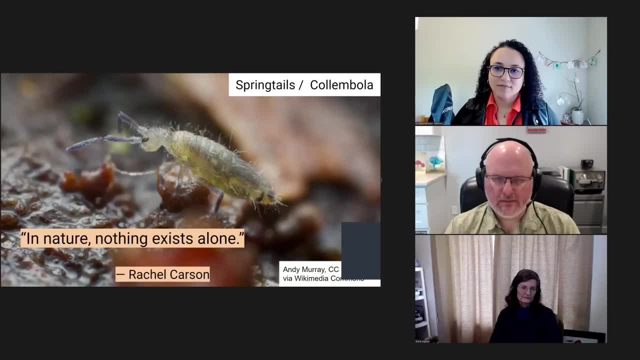 services have more space to thrive, And so it just makes me think of this Rachel Carson quote that in nature, nothing exists alone. Even though I'm a fungi nerd, I love Calembola, I love bacteria, I love protozoa and nematodes. 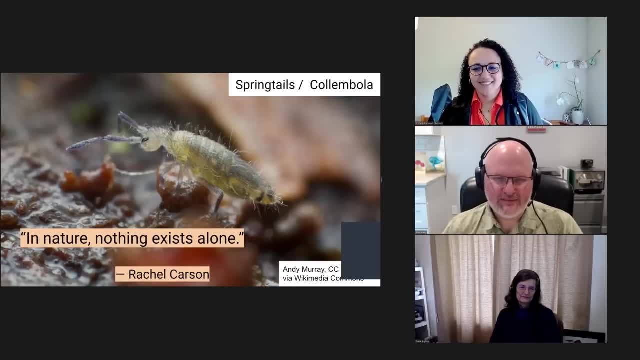 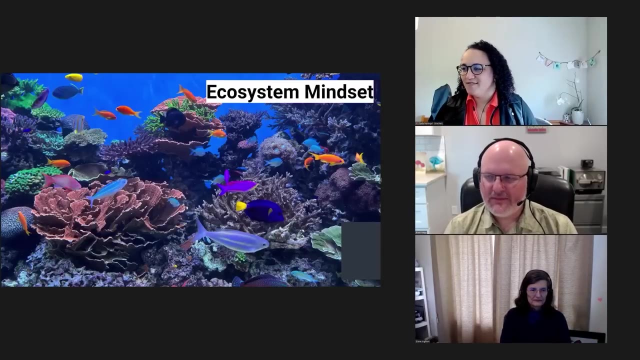 It's all important. I don't think I have anything else to add. Do you want to move on to the next slide? Sure, Okay, This one will be pretty quick. I want us to just think about the fact again that it's easy to look at a coral reef and 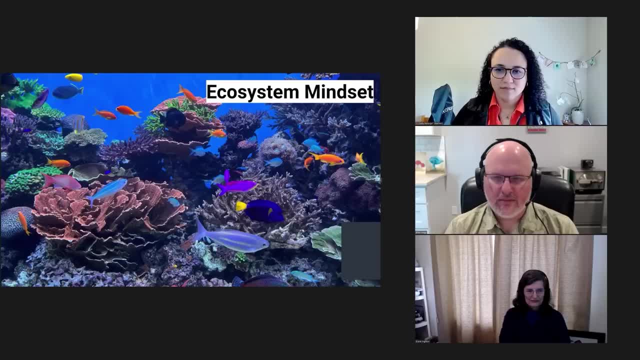 all these different colorful fish and the shapes of coral that are there and say that's full of diversity. There's different relationships happening there. It's easy for our eyes to take that in and our brains to consider. It's easy to conceive. 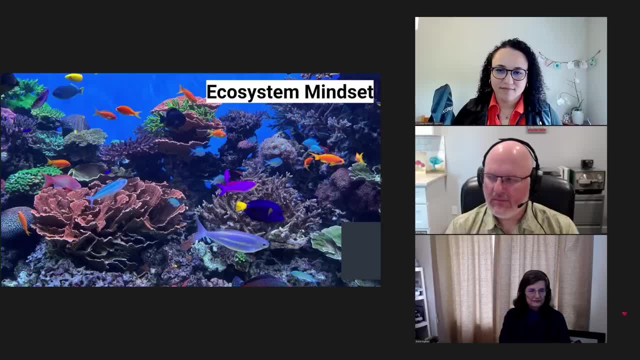 And soil is just as full of interesting stories. We want diverse, thriving, abundant soil ecosystems, And so part of soil vision is having that mindset that the thing we should expect is to be overwhelmed with the amount of diversity in the soil And in so many agricultural systems. you go in there and you find a few measly bacteria. 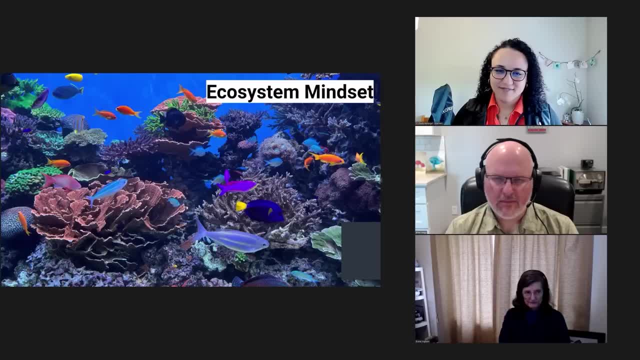 And you. it would be the same thing if you saw a coral reef after a bleaching event and you said there's a few fish and some algae hanging out. that is not a coral reef anymore, It's the skeleton of a coral reef. 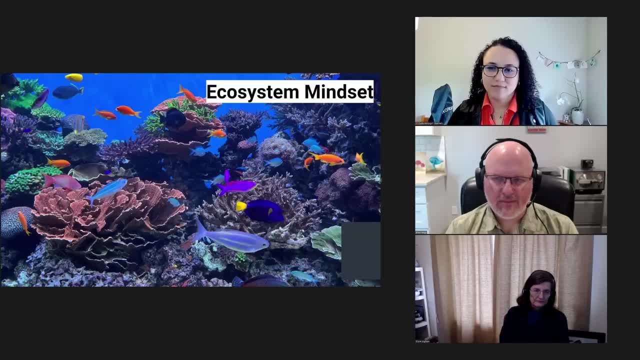 And the dirt that we're farming on is the corpse of the soil that used to be there And it is not. it is not the future. The future is soil ecosystems. Okay, If I just may add, it's not that only intensively high visible biodiversity is what we're looking. 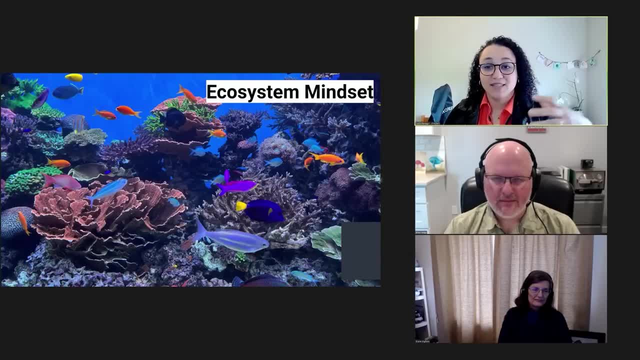 for but the original biodiversity in the place that you are. So we need to respect the origins condition of the place that we are. I'm glad you said that. You know I follow some online groups that are a bunch of ecology nerds and someone. 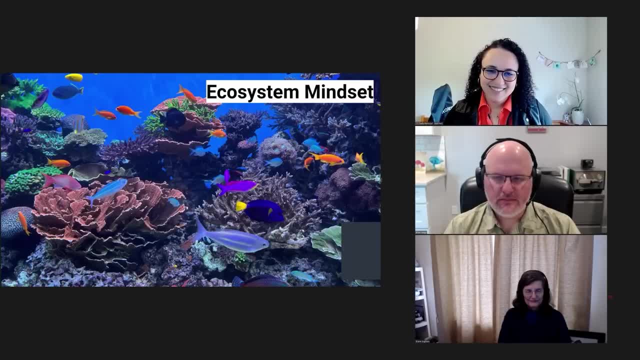 took a screenshot Of the new scene from the new Little Mermaid movie And they said: here we have a bunch of species that never, ever live in the same place. This one's from the Indian Ocean, that one's from the North Atlantic, and all that. 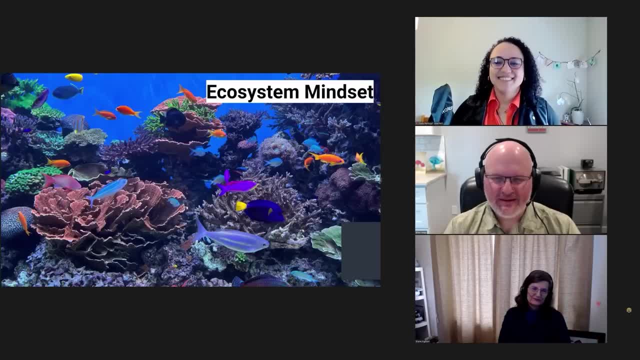 And that's a conversation that comes up online sometimes during our advertising- that people are concerned that we're mixing and matching microorganisms, And I'm here to tell you that as long as I'm here at the Soil Food Web School, I am going. 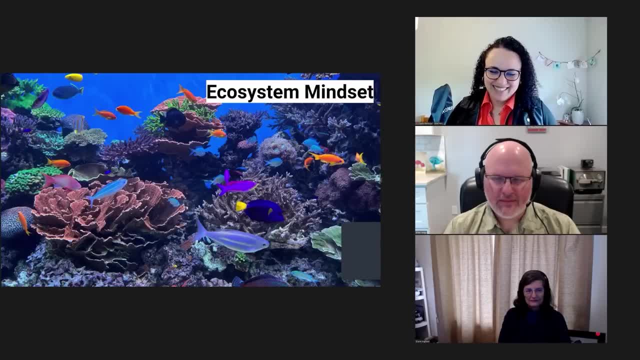 to keep preaching, Preaching this message that it is locally adapted populations of microorganisms, things from relatively nearby to the location, that have the right capacities to work with the local soils And with our- you know- imitation of nature's diversity on the farm. if we, if we manage, 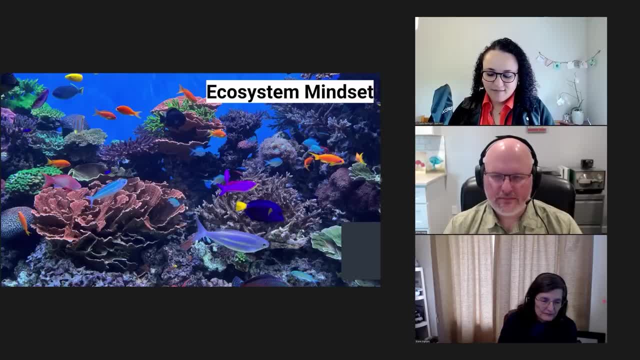 that properly, To create these stages, To create these stable and thriving soil ecosystems, we cannot just pull things from Pennsylvania and use them in California or vice versa. It's so important to understand the limits of your biome, And one biome may be very large and the next one may be relatively quite small. 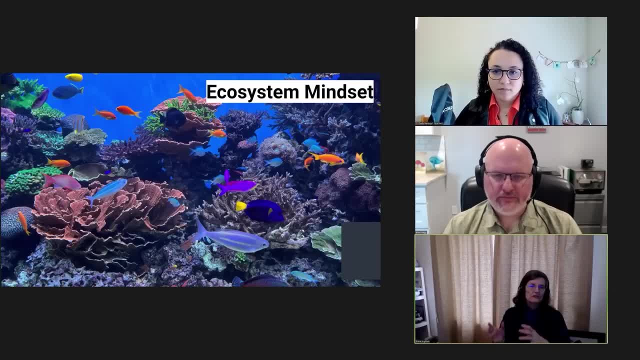 We have to learn that you can't take things from one biome And just blithely put it out someplace else, assuming that it's going to do the same job in the place you put it, as compared to where it came from. So we've got to be doing, be very careful not to cross those boundaries, and we need 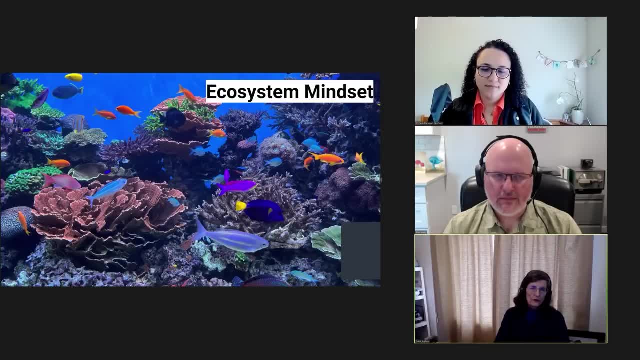 to define those boundaries very carefully For each level of the food web that exists. it's going to be a monumental job, But sooner or later we'll get around to it. I'm excited for that. I'm excited to co-create and share this knowledge across this global. 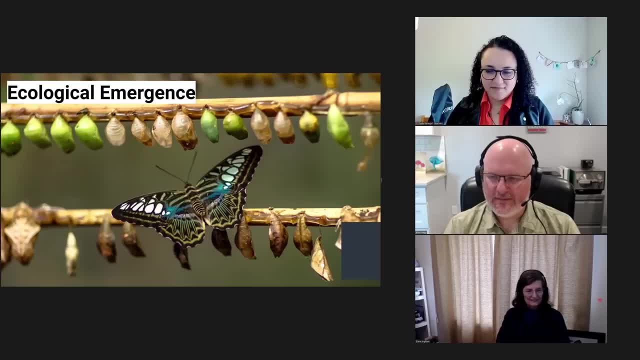 community, Adam, I moved on to the next slide. Perfect, I thank you for keeping track of time for me, Sure, So I wanted to introduce another term, you can. you can find some great stuff on YouTube about Emergence and the theory of how this works in biology and ecology. 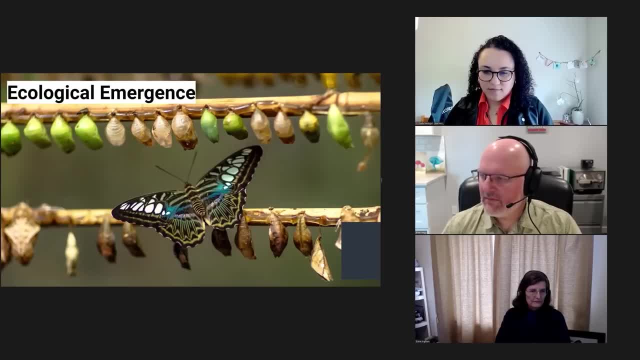 And I think about the metamorphosis of the butterfly here. But let me see if I can explain emergence, When you, when you have two things, living things in an ecosystem, they have one relationship. We have three things, you have more relationships. we have four things, you have more relationships. 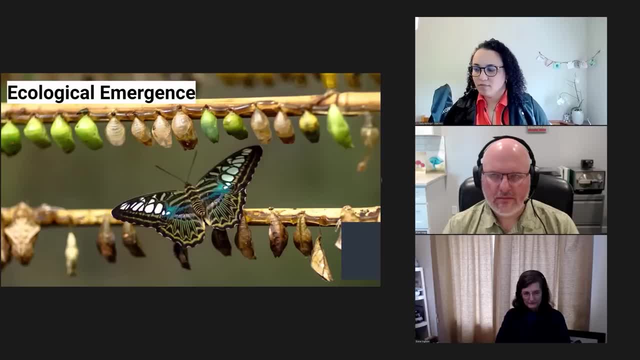 right, Because each thing- maybe it doesn't interact with everything else, But it has a bigger web of interactions. Something happens When you get to a place, through you know what we call succession, where you've had a big disturbance and there's only a few things that can survive in that dirt. 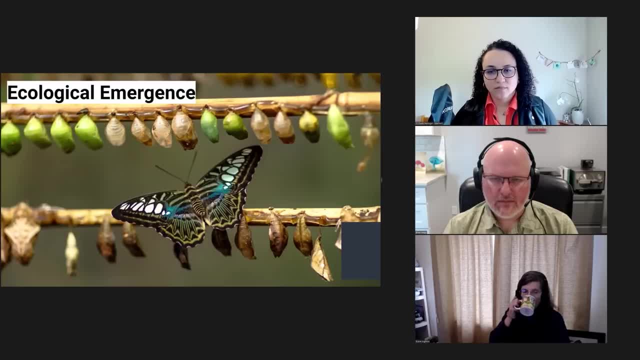 And then they start to build up and change the conditions And you can get more and more life, their diverse life, abundant life. you start to have the emergence of some strength And resilience that, even if we sat down and tried to calculate it, we would. so this: 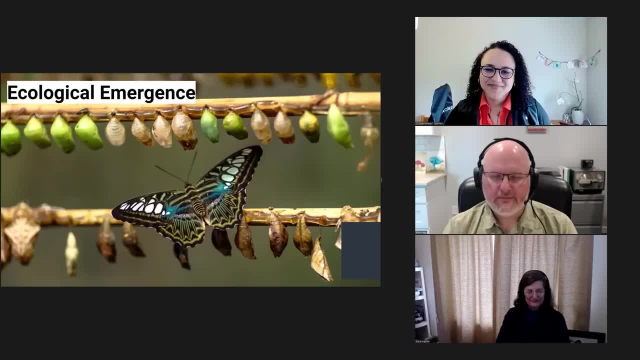 is like more than the sum of its parts. This isn't just what the answer doing and what the fungi is doing and what the bugs are. you know these other bugs are doing. added together, it's multiplying. each new thing in this ecosystem multiplies the power of the ecosystem, the stability of it. 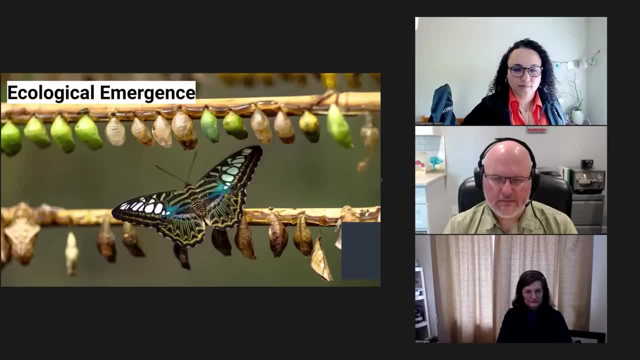 And to me, fungi, Again I go back to. They- are one of my first loves in the science world. They- I think of them as the facilitators of emergence, that that they get into relationship with, like almost everything, And sometimes it's an antagonistic relationship, like if you have, you know, certain problematic. 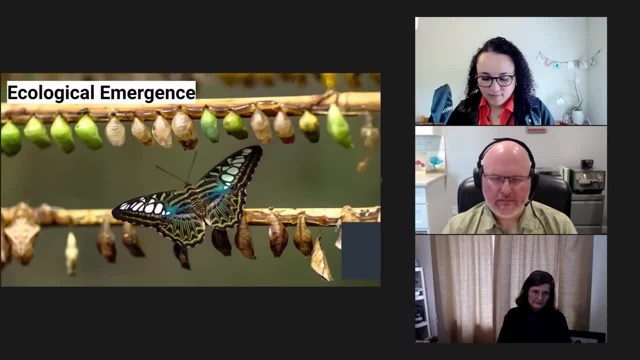 nematodes in your soil that could harm plants. fungi are going to make little traps and keep that population under control And a lot of times, In the case of our muscular mycorrhizae, is majority of a very beneficial or mutualistic 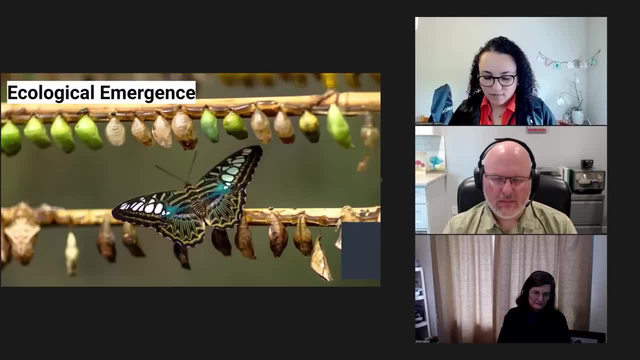 relationship where the plant wins and the fungi wins, And so I I'm just enamored with ecological emergence and what happens there. it's. another piece of the magic to me is the is the diversity of these systems and fungi help it to unfold. 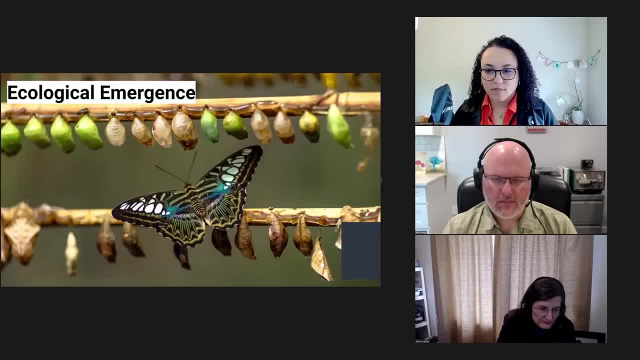 more rapidly and more beautifully. Yeah, You know this is something that I come across quite a bit, you know, in the work in agriculture, where the ecological emergence is definitely not there. You know, when we get looking at soil, sometimes it's just bacteria dominant. there's no predators. 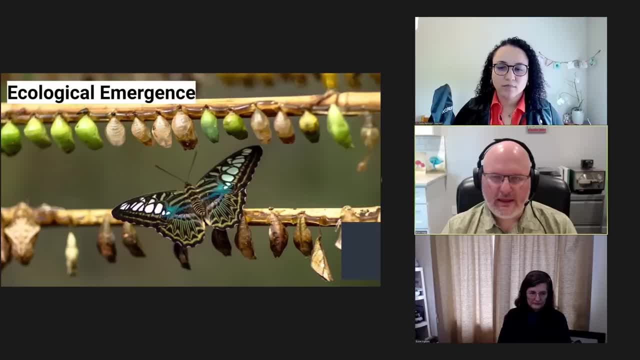 in the system there's no fungi And it just kind of amazed me that as we start to establish that soil food web, The speed at which the plants respond to and the amount of vigor, It surprises A lot of Clients. It surprises me. 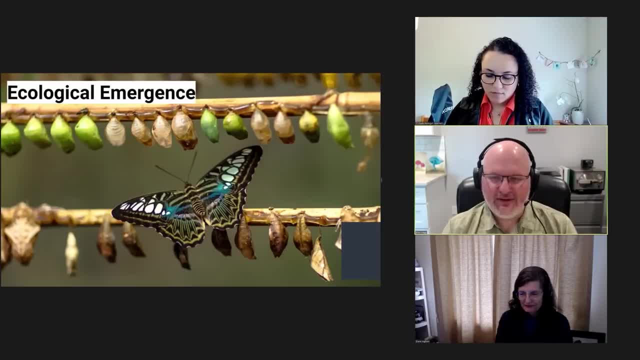 Hell. most of the times too, It's like wow, this is just really taken off, And I think it just- you described it elegantly- about the that it's the multiplication of powers, not just the sum of all the parts, that that really makes the system work. 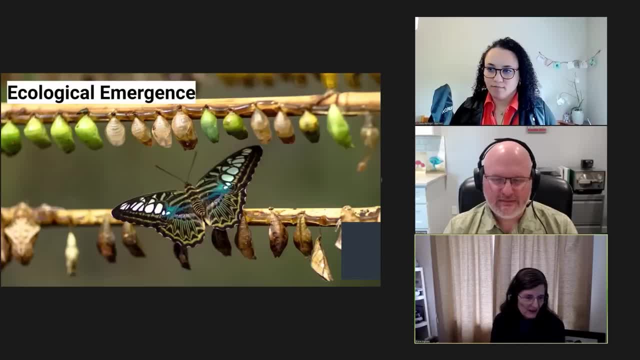 There definitely are emergent properties When we started having lots of individuals of different species all doing their thing. So everything gets faster, Everything gets more conclusive, That diversity that we have. well, you know, do we have all of that diversity or not? 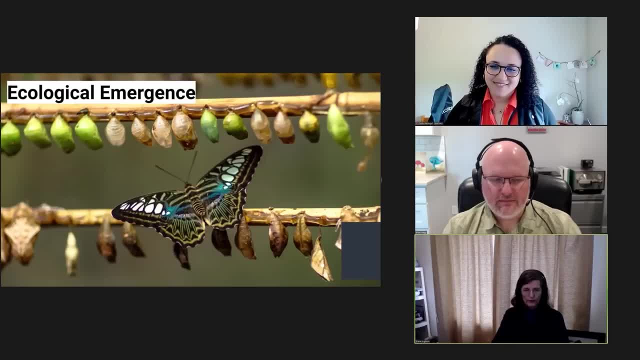 We need to have places where we've stored away that biome So we have a place to go and get the diversity of organisms If something catastrophic happens outside that reserve. if you will, We've got a. We've got to understand that we kill these organisms off to our own less stable conditions. 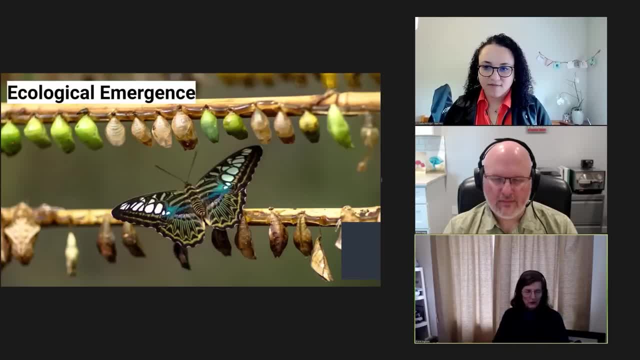 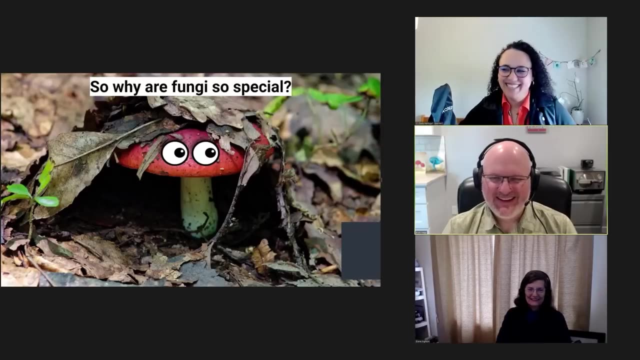 When we're trying to be healthy and wealthy and wise. Absolutely Okay, We can go on to the next slide and I think I'm finally going to talk about hollow bite. No, Okay, I got Okay. I think I've already fronted this a little bit. but why are fungi so special? 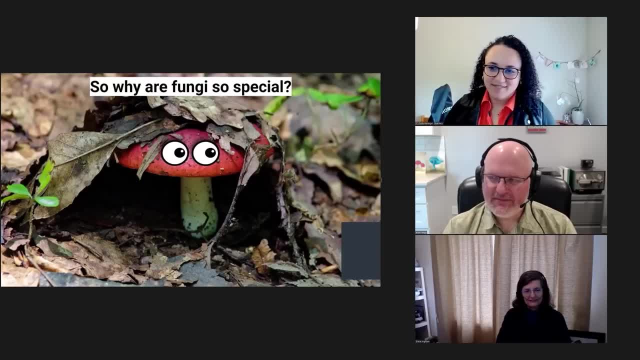 Well, there's the, the cuteness of mushrooms in the forest right, And Heather helps me make this one even cuter, I think. But it's also, it's what I mentioned, It's the fact that they're facilitators, that they're in deep and beneficial relationship. 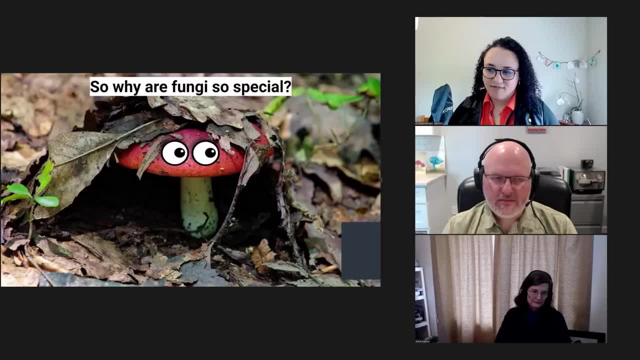 co-evolved with many organisms And, in fact, Some of the fungi I'll talk about today. We think we're instrumental in in plants being able to move out of aquatic systems where they first evolved- onto land. So we're talking about a 400 million year old love story between the fungi and the plants. 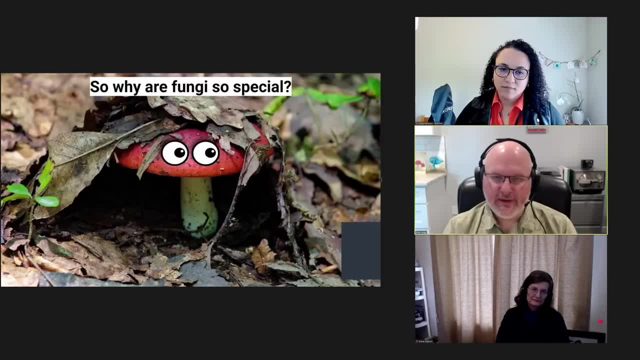 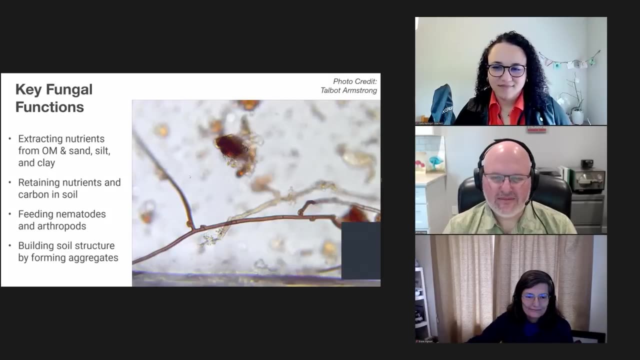 That's a lot of time to evolve, right? Okay, Yeah, sure, Okay, Oh, perfect. So a lot of times, we have to speak to the practical benefits of things as well, And so these are just a few of the key fungal functions in soil. 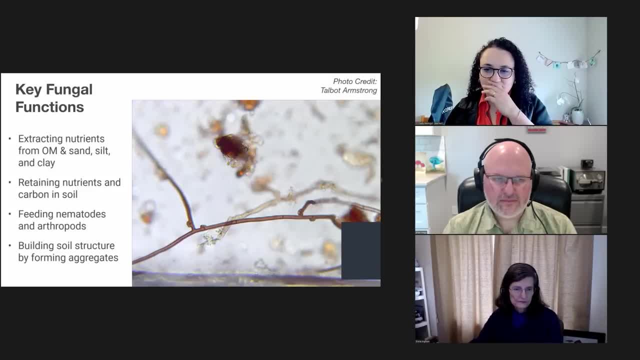 If you, if you bring back a thriving, diverse population of fungi into your soil, there's going to be a greater capacity for your soil food web to extract nutrients, and from organic matter They can supplement different types of nutrients. So when they actually come up, they're going to give you the better enough nutrients to 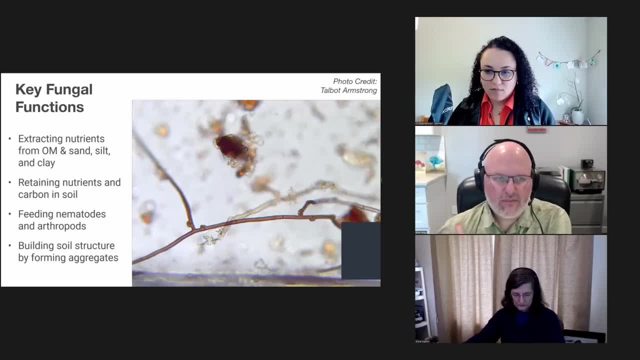 feed the plant. So the more that you have the right nitrogen that we produce, at least as an information source for manure that you can get, the more nitrogen you can get into the plant So you can have the best nitrogen output or the best nitrogen to get to your vegetable. 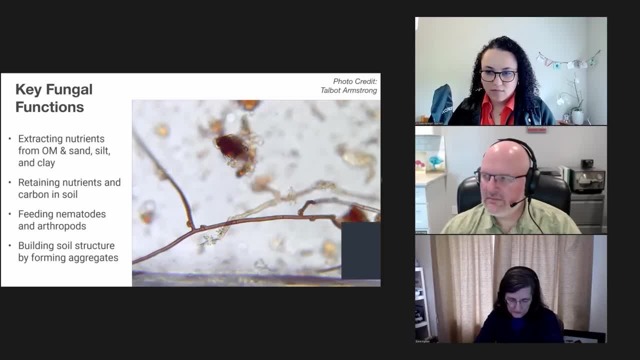 harvest, probably your vegetable garden Right, In a way that is equal to the amount of nitrogen that you can get from your field. your plant, your land Right, And so it's an important part to work that You can't just say I'm going to plant this plant, but I'm going to upgrade it. 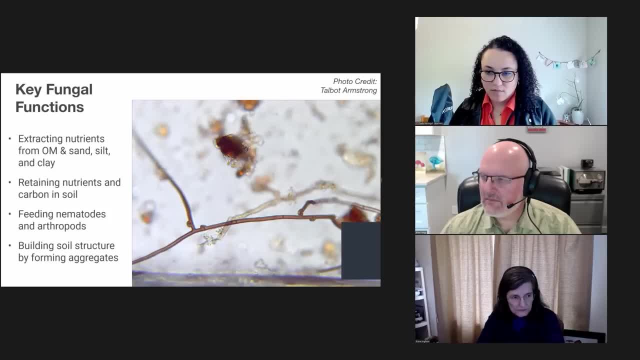 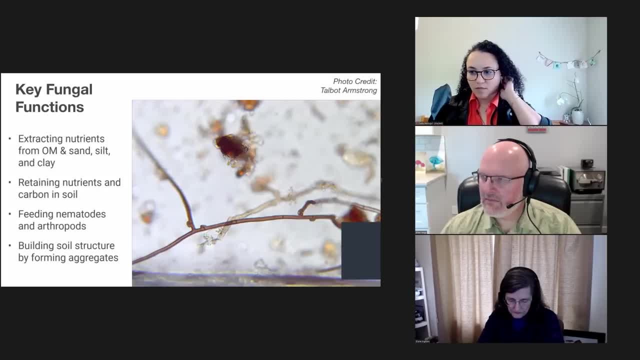 or animals or whatever, off the farm and sell them, And fungi are absolutely important for that, especially when we're talking about the digestion of more complex materials. Bacteria just simply don't have you know the chemistry that they need to chew up some. 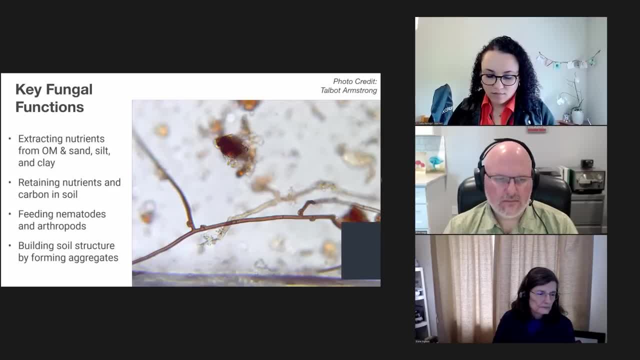 of these woody materials and other things very rapidly. but fungi are specialists in that. They also really help us retain nutrients. Bacteria do as well in their bodies, but fungi have a special role to play in getting more carbon into soil and holding that carbon there longer. 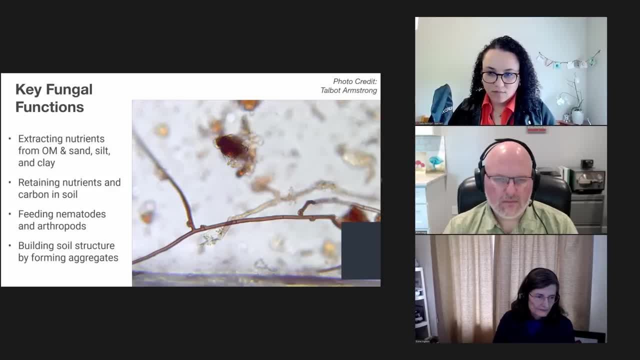 So a bacteria. if you chop down your corn plant and put it under a little bit of soil and the bacteria eat it, they're going to respire about 60 something percent of that carbon as they digest that corn. They're not very efficient. 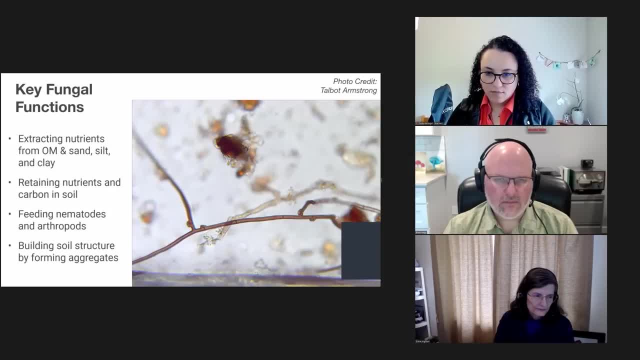 And so a lot of that will go back to the atmosphere and we won't have this, you know, this desired drawdown of atmospheric carbon. If the fungi are really dominant in that soil and they're highly involved in the decomposition, instead of losing 60 percent, we can retain more like 60 percent of that carbon. 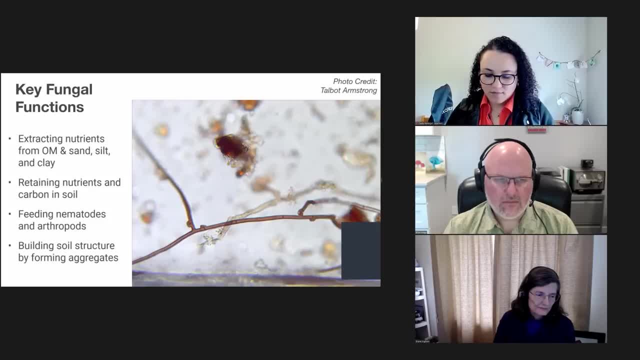 So that's really important. Yeah, Yeah, Yeah. 60 to 80 percent of the carbon that was already fixed through photosynthesis into that plant because as they make these hyphae which we show here of the Bissidiomycete, and it's nice. 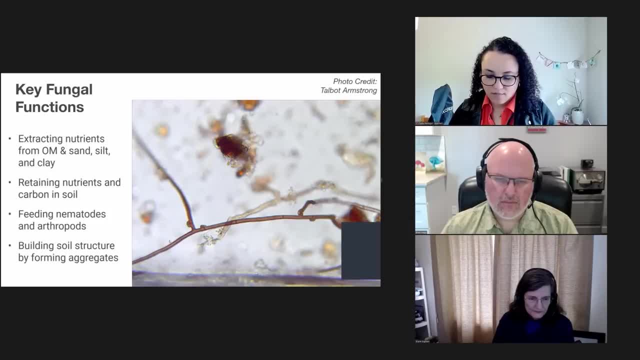 brown hyphae and clamp connections. they lay that carbon down as a very complex form. They have physical protection. One of the things they make is chitin, which is what make insects and crabs really strong, armored, And those won't just disappear very rapidly back into the atmosphere. they'll be retained. 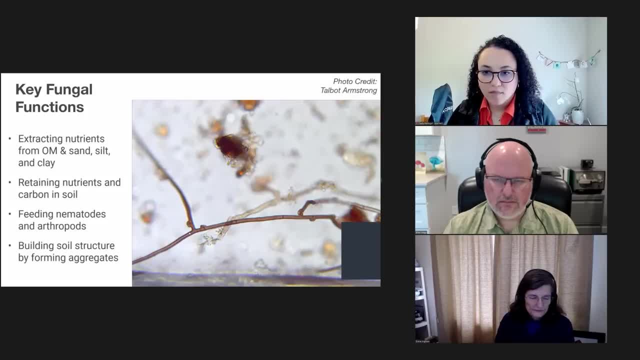 in the soil, in some cases for hundreds of years. They do provide food for nematodes and arthropods, things that can pierce through that tough shell and suck the juices out of the fungi. they get those nutrients And then, when they excrete their extra nutrients as waste, it feeds the plant. And then maybe my favorite thing is that they help build structure in the soil. The bacteria help glue together little, tiny crumbs of soil- that we call micro aggregates- and the fungi come along and entangle little crumbs and make big crumbs that we call macro aggregates. 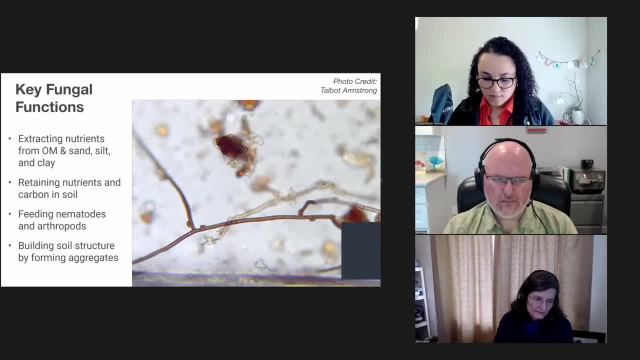 And when you glue together and entangle and make a complete, complex soil structure, air can move deeper, water can infiltrate and be held there You start to form the soil sponge And fungi really facilitate that kind of stability and structural improvement in soil ecosystems. 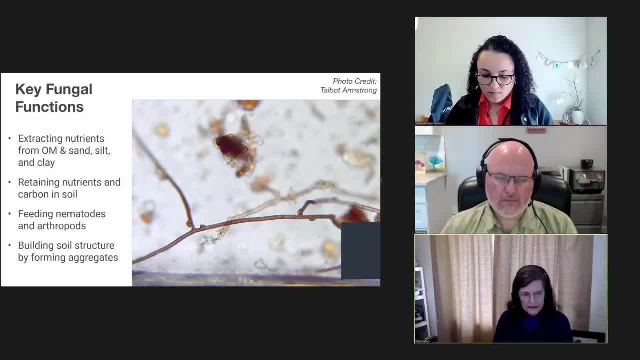 One of the things that we've been working on a little bit is to understand where the fungi are putting their nutrients. So again, this is how we do that sort of parcel. You see a lot of different troops that are putting down, or laying down layers of almost pure carbon on the inside of the hypha, And so the communication gets less and less, if you will that. highway of liquid material going back and forth through the hyphae And also it gets less and less, if you will, of that road, so more and more kind of sale to that road And if you see that there isn't a lot of oil or compostgang canceled on those soil, structuresiasin Вторny photo__·. 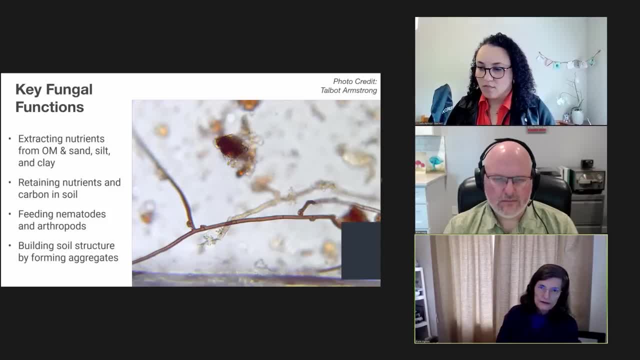 Now 100, I'm not going to get the. I didn't go and look at the. yeah, so whatever the normal amount is, you know, some people said: well, you know, soil can't take up and hold more than 0.01 amount of carbon. 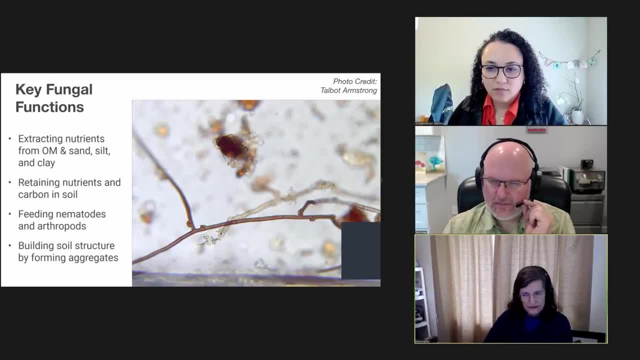 When what we're seeing in the fungi at least, is that we could be, you know, 100 times higher than that. So we need a lot more understanding of what's going on in soil, but we need to recognize the role that it plays- that fungi play- in carbon sequestration. 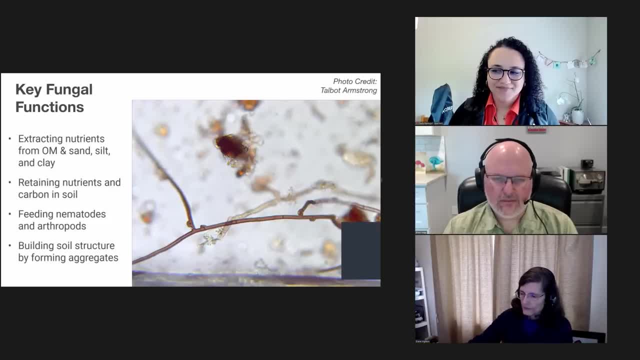 You really hit on something, Elaine. The dominant story about soil is mostly based on the story of education. Dirt, Yeah, That's what most of the universities are working with, That's what a lot of farmers have experience with, And so we are not talking about soil that's full of life and fungi and all the other things in the soil food web. We're talking about dirt, and dirt can't save us. 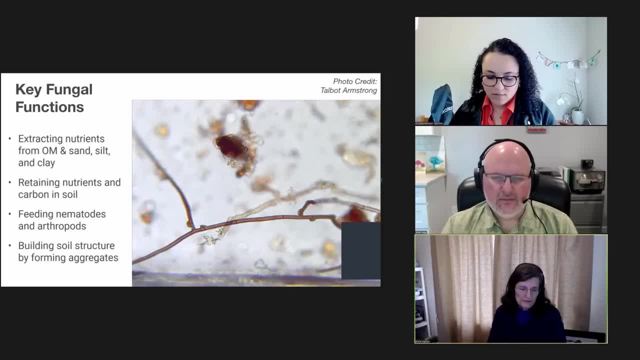 There's no mechanism for them, for dirt, to be able to do anything, Because you have to have enzymes, you've got to have a means of changing your world, And we don't see that if we are trying to make a case out of dirt. 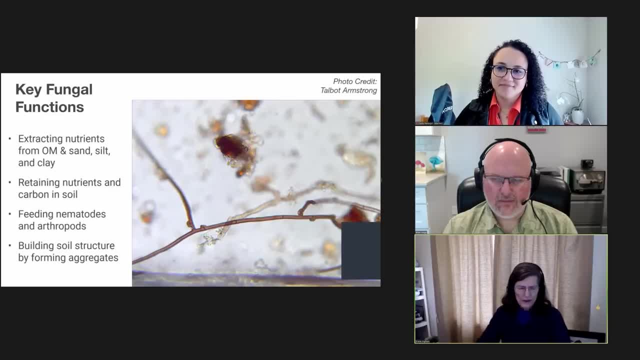 So when people are growing their plants and they see the plants aren't growing so well, they go out and they get an inorganic fertilizer and come home and dump it on the plants and say, see, that's what was wrong with these plants. 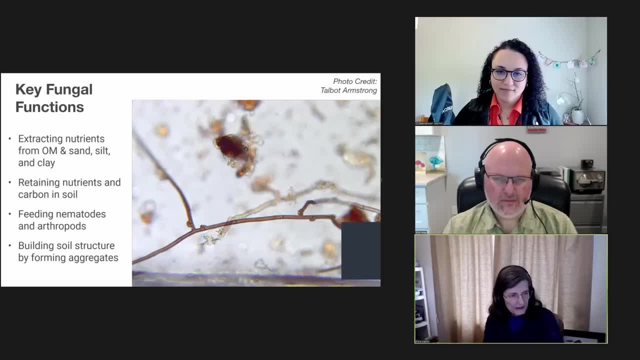 They just needed a little bit more inorganic nitrogen. When most of that inorganic nitrogen, When most of that inorganic nitrogen is actually going to be lost from that soil, from the dirt- sorry, 80% of what goes on to fields where you can get a reaction, an improved growth, it looks better, it grows faster for a short period of time, but ultimately 80% of that inorganic fertilizer is going to be washed out of the system through leaching, through erosion. 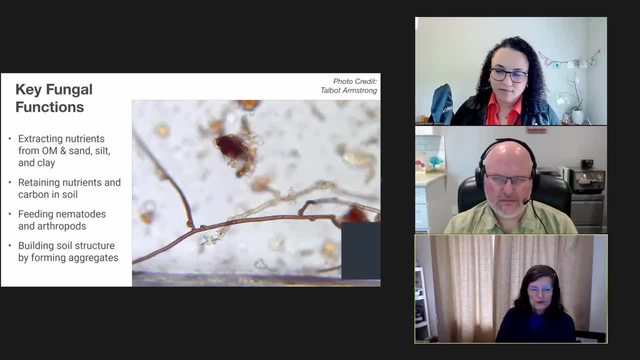 You can't hold on to those nutrients unless you have organisms growing using that to tie up that carbon And then all the consequences that come along with that, leaching right. I mean look at all the watershed damage that's been done. 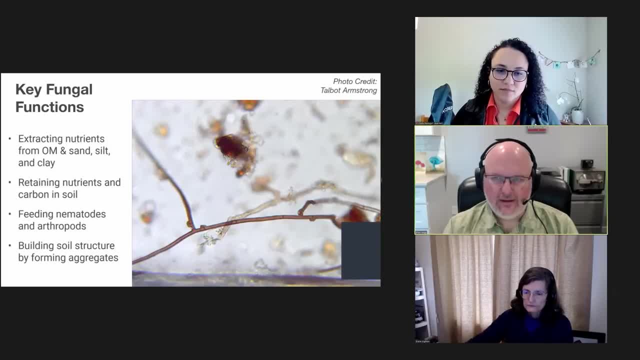 The Gulf of Mexico is just really all that inorganic N ends up there, causes massive algae blooms. There's a lot of unintended consequences. I think that comes with that kind of fertilization paradigm, Plus all the damage that's not been even mentioned, right. 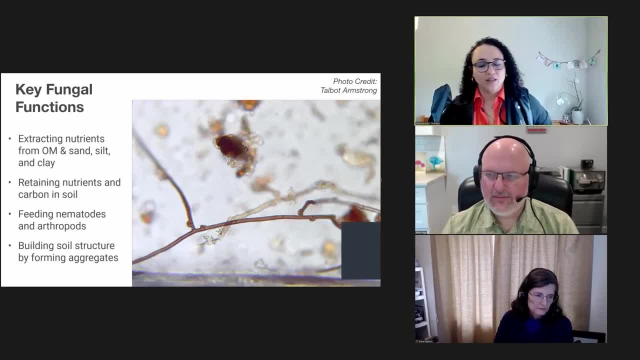 It's not being measured, It's not being monitored. So there's a lot of things that we can do, and fungi definitely plays an intense role on that: restoration, recovery, everything in the process. You're absolutely right, Carla. I have watched. 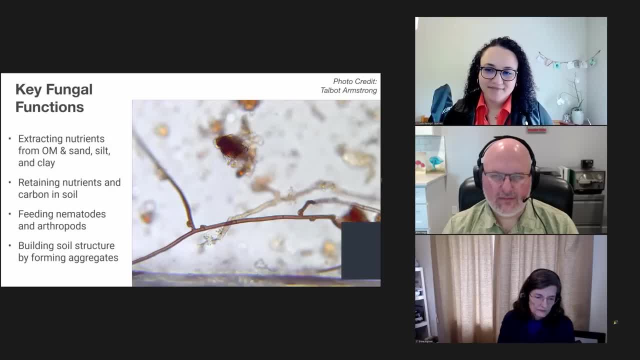 It's been very gratifying over the last 15 years since I fell in love with soil, to watch the world Falling in love with soil and these conversations happening. We're getting to the deep awareness phase where more and more people say we have a problem. 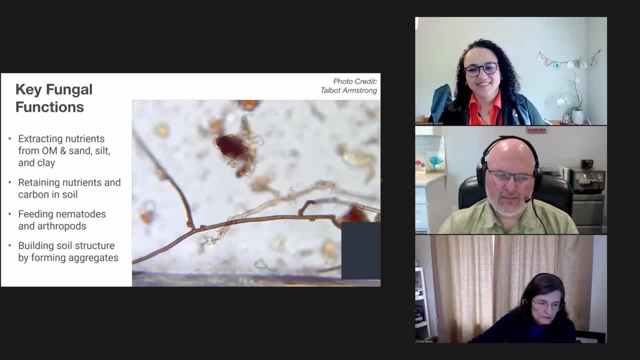 There's only so much before. it all erodes away and is gone. And now here at the school, other communities in the regenerative sector, we're starting to say: let's reach for answers, then, And let's teach those answers widely and share that knowledge and build a community that can co-create. 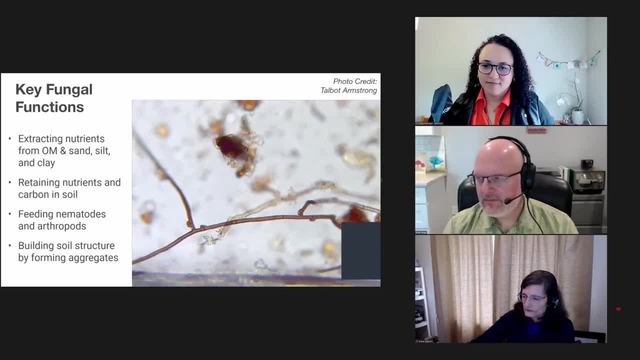 The future together And I am so excited to be part of that story. A question was just put down about how do you determine when you've got more fungi or any one of the organisms, the constituents of our food webs. You need a microscope because it's really easy to see whether these are fungal hyphae or not. 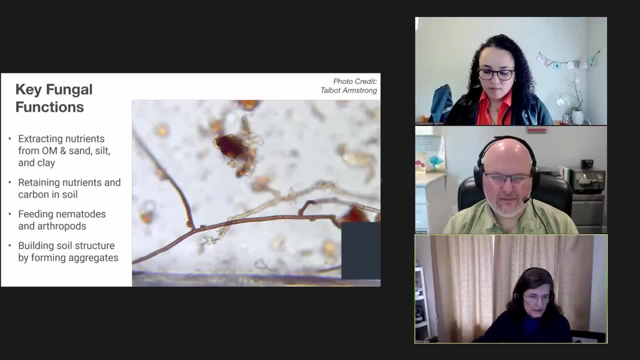 We can even show that it's a basidiomycete. It's got clamp connections, It's got cross walls, So you can differentiate fungi from bacteria, from protozoa, from nematodes Very easy. It takes you well when you first start out and you're having trouble feeling absolutely certain that this is indeed a fungus. it may take you half an hour to do a sample. 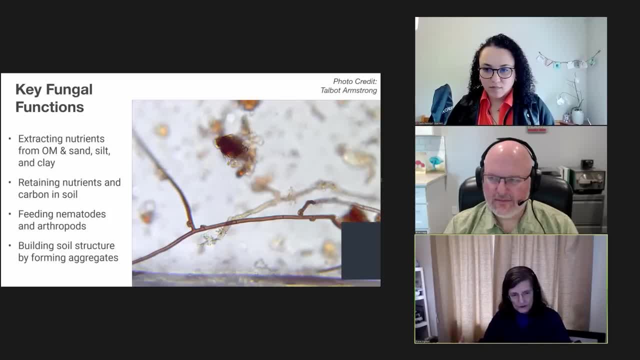 But by the time you start getting comfortable, having looked at enough of these of the preparations, you can get the whole sample done in the matter of maybe 15, 20 minutes. So that's all of the readings that you need. So it starts out slow, but you learn and you get faster and faster as you have more confidence. 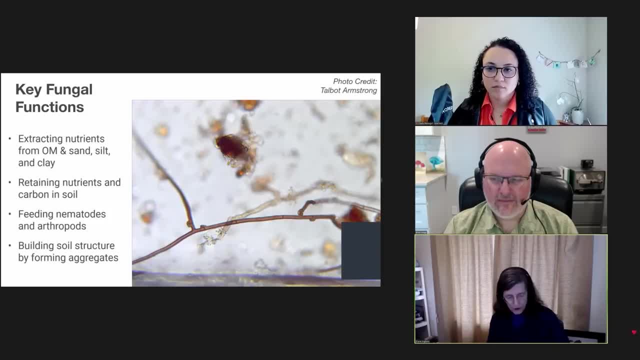 So that's the easiest way to know whether you've got. how much bacterial biomass do you have? How much fungal biomass do you have? Yes, Yes, Yes. And then by comparing today's date and what you saw, with next Mondays or Tuesdays or Wednesdays. 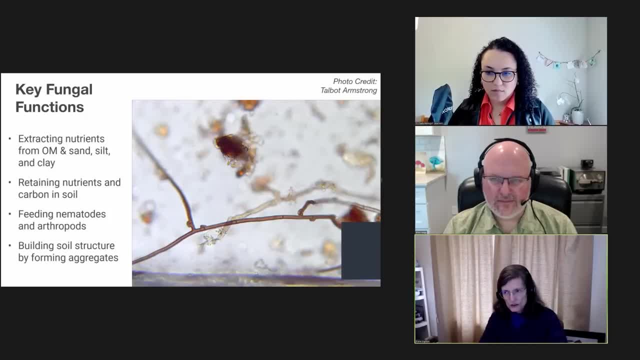 you can determine how much bacterial biomass increased or decreased. Same thing with bacteria, same thing with protozoa, nematodes, microarthropods, earthworms. you know the whole shebang. So it's a very effective way of understanding the differences of who's growing and who's not. 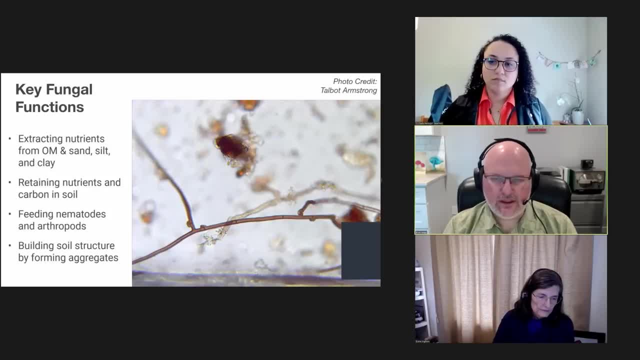 And it's accessible too. I mean, really, the type of microscopes we're talking about are you can start off in the $300 range and you're plenty fine for assessing these organisms, And in fact I've got probably- I'd say maybe 25% of my clients have now purchased microscopes. 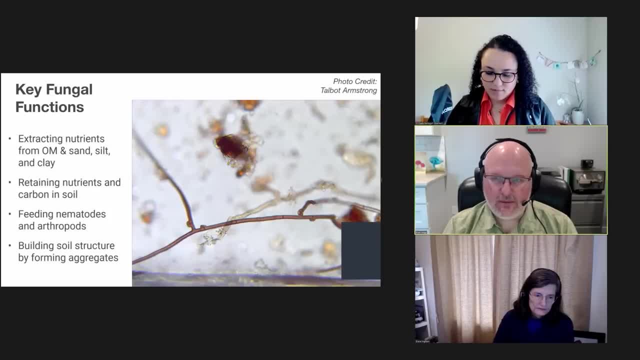 And you know some of them have no microscopes. They don't have any microscope experience at all, but just a little bit of training and starting to tune their eyes to seeing these organisms. They can do pretty good qualitative assessments of their soil and say, yeah, I've got fungi growing. 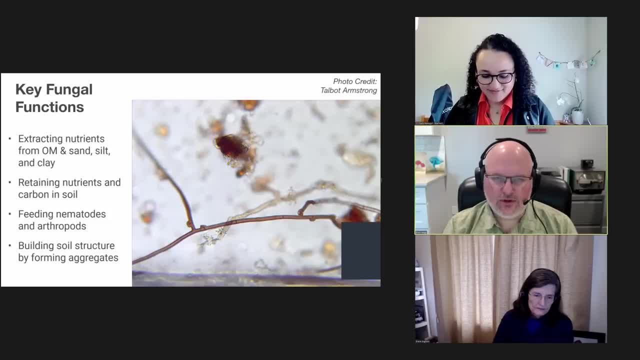 I see a difference or a change. I think it's such a powerful tool Absolutely, And it's pretty different if you go from zero to a lot. Almost anybody can tell the difference between zero and a lot, A lot, exactly. You don't have to have to actually be quantitative. 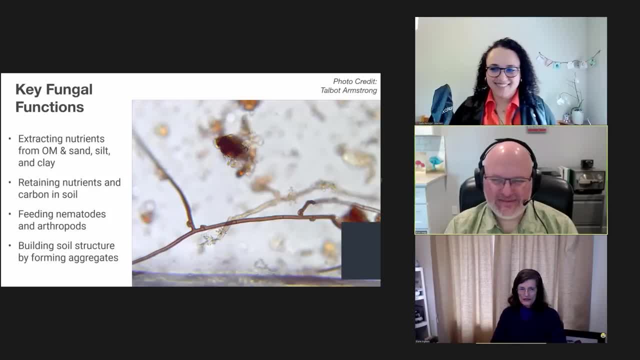 You can be quantitative to the nth degree in order to understand that things are very different now as compared to before. We've brought the fungi back into the soil and we can start calling it soil. Nutrient cycling gets going again and you don't ever have to put. 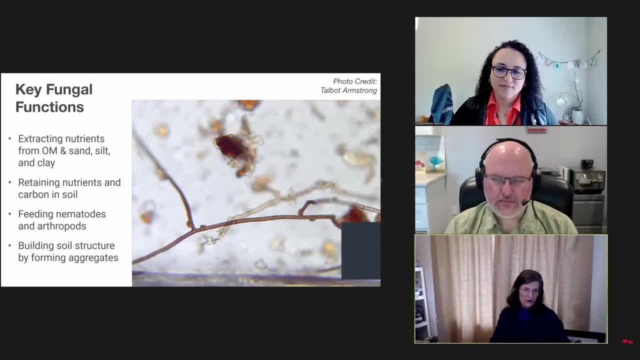 and that is now held in that microbial biomass through that wintertime. next spring, when the predators start waking up and start eating their bacteria and fungi, Massive amounts of nutrients that the plant requires are released right in the root zone. 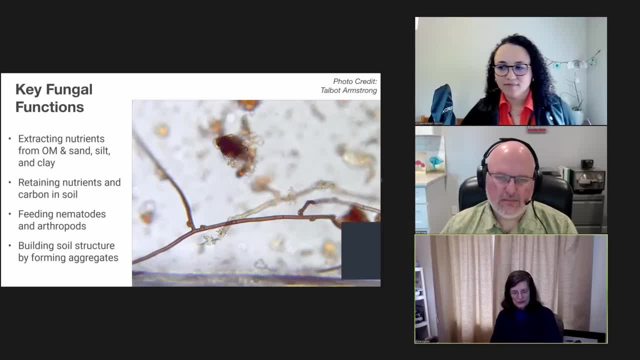 There are a couple new systems that have just been discovered, rhizophagy, for example, and at the soil summit that we hold here every year. The first is the James Winters, James White. Thank you. 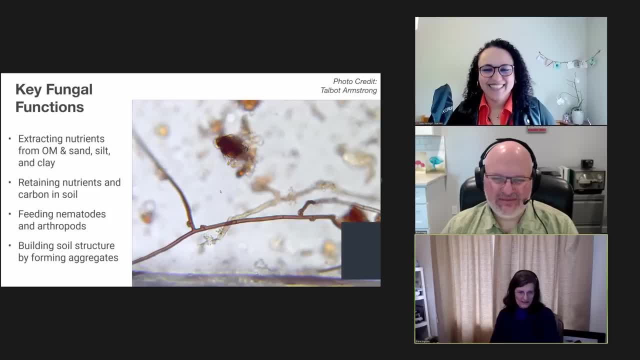 White Rikers actually is where he's at, And so he talked about this whole other way to do pretty much the same thing as the predator prey interactions, But with that system, with rhizophagy, it's the plant attracting the bacteria to come into my area and the plant closes off those bacteria, extracts the nutrients that it needs. 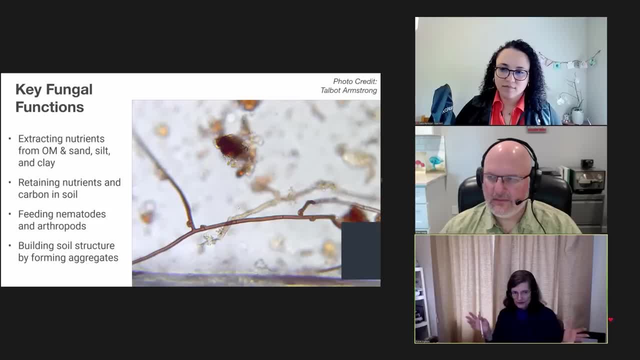 And then all of those little bacteria get to escape out of whatever it is around a root hair that allows open space. And then those bacteria go right back down to the root tip and they want to do it all over again. So it's really interesting things being discovered. 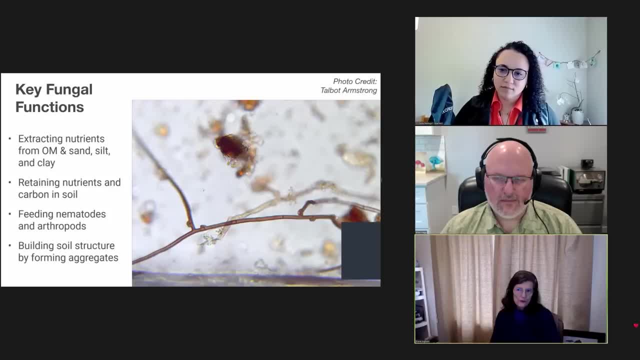 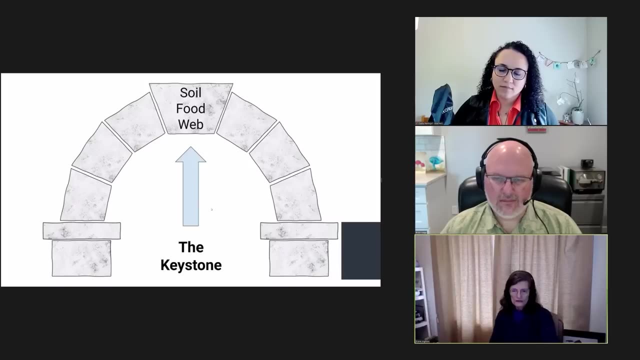 Just finding out that we have nitrogen fixation occurring in the sap Of many of our agricultural plants. Just begun trying to figure that out. So stay tuned, Come join in the fun. All right, I think Brian is signaling to me that I need to speed up a little bit, and that is okay. 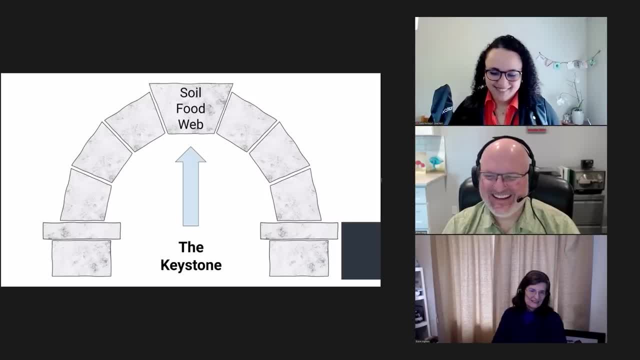 Because, you know, when I had this technology problem, it was almost like getting an extra cup of coffee for the amount of adrenaline I have in my body right now. Sure, So I've mentioned keystone species a few times. I just wanted to quickly put this visual that I haven't hear a lot when I give talks, because it was an aha moment for me. 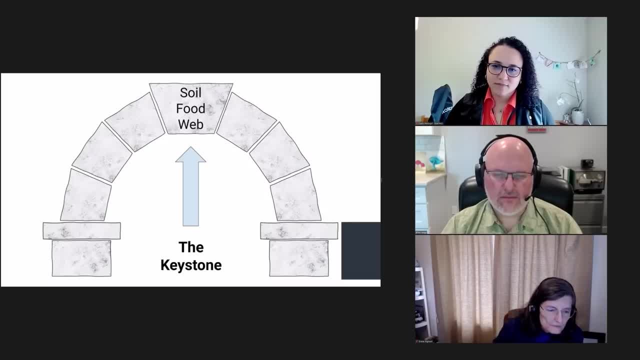 That anything that we do to study the management, nutrient dynamics, habitat, how to adapt to climate in an ecosystem or an agricultural ecosystem, is like putting another piece of this arch together. Right Yeah, But if we do not have the keystone in the arch, the arch will fall down, and the keystone to a sustainable and regenerative agri ecosystem is always going to be the soil food web. 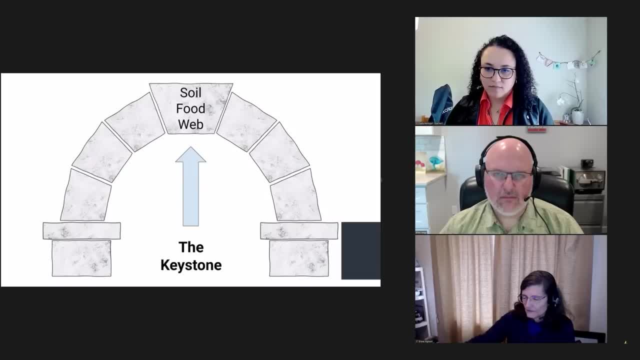 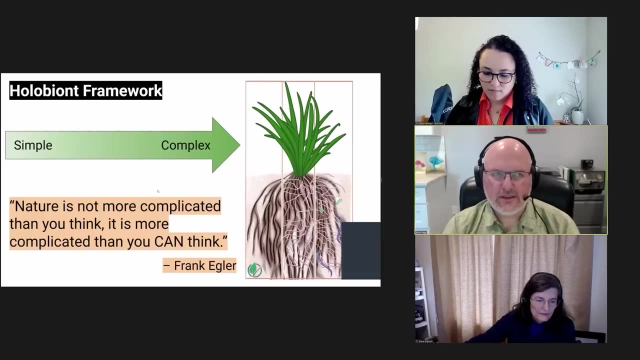 And so again, I'm just saying fungi are a really cool part of the soil food web It's. but if we're missing it, if we're missing those key functional groups, our arch will be weakened and eventually it will fall down. All right, I moved us to the next slide. 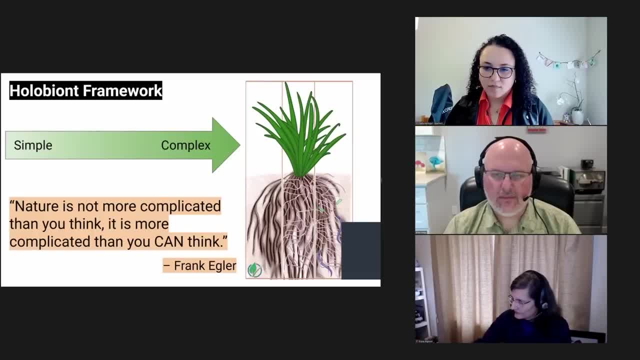 Excellent. So I said that I would explain the hollow biome, And I've got one of my favorite quotes in the world by Frank Eagler there: Nature is not more complicated than you think. It is more complicated than you can think. This reminds me of the way that for years we said agriculture is about growing plants and taking care of animals. 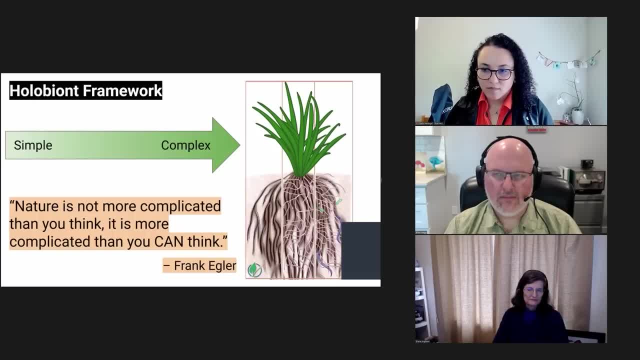 And we just thought plant, animal. And then You know, we've had a nice amount of time, several decades, where a lot has been discovered about these important fungal relationships represented in the middle panel of that graphic. And that's where I spent a lot of my time in grad school was looking at the mycorrhizal fungi and the other important part of the of the system and how they extend the reach of the roots. 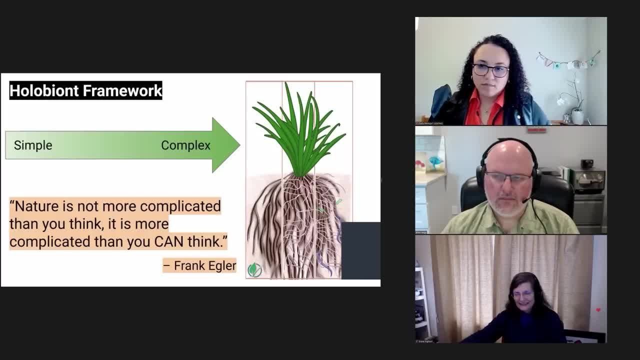 But then through the foundation courses and my involvement With, with our staff And with Dr Alain here, I got to the fully complex, the better picture of more correct visual, a visual capacity or imagination capacity to say There's actually a lot of things in there. 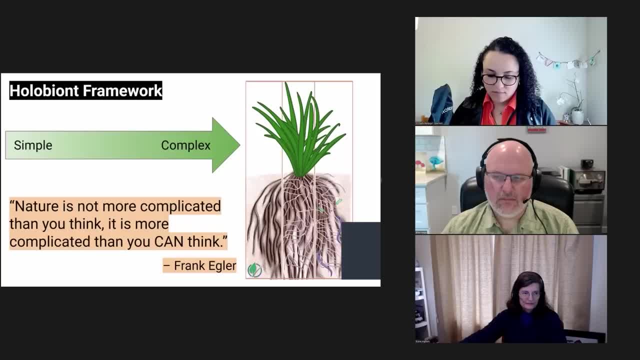 The fungi and the plants are not enough. It's more complex than a human can think It would. it would probably take more than any of the computers, even with all the AI and stuff that we're doing now, to really get to parse out all of these relationships. 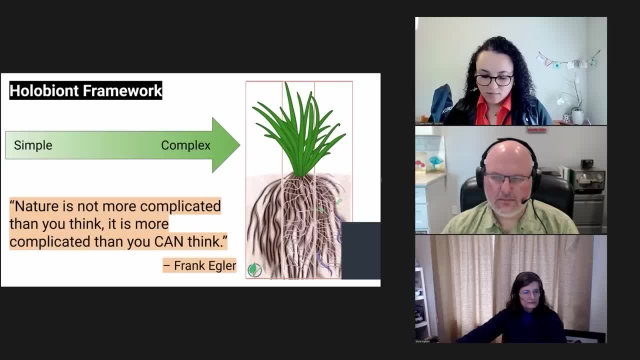 and connections. so the holobiont as an idea says you can't separate the plant from its microbiome, you can't take it apart and really study just the plant and get good answers. it's essential that it has its fungi, it's essential that there are bacteria and protozoa and nematodes, and so this: 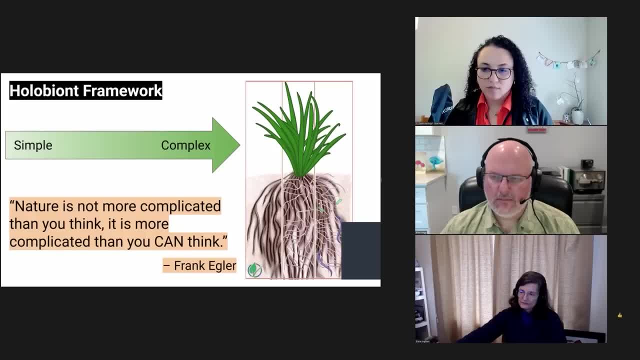 is why we say we're not anti-science. we're not against the research that comes out. i read science papers every day, but i always come with this filter of: did they set this up, where they separated the and broke these key relationships, and and how does that affect their conclusions and what about? 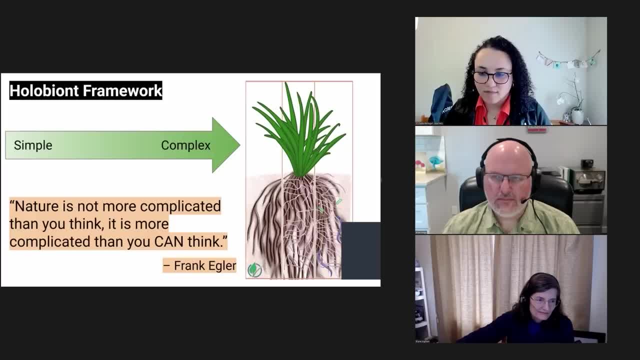 the system that continues to say reduction is the answer, instead of looking at the holistic emergent properties of complex agroecosystems. and and what are the people in that system have to gain, potentially, from keeping all of us under the dominant message, the dominant discourse in our 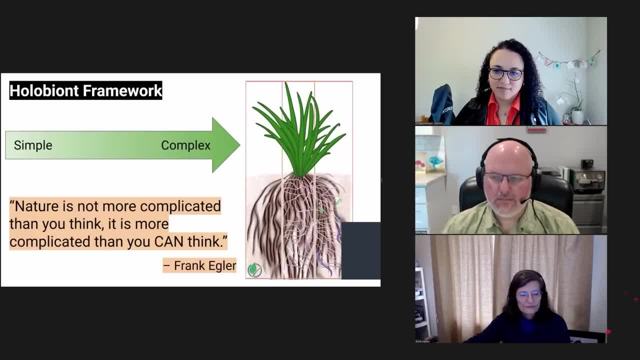 society that plants are just. soil is just a substrate to put your plants in, and you put your nutrients there and you put your chemicals there and you get your yield. and that's how it has to be. it's not how it has to be. this is the outlier of human history, for much of human history. 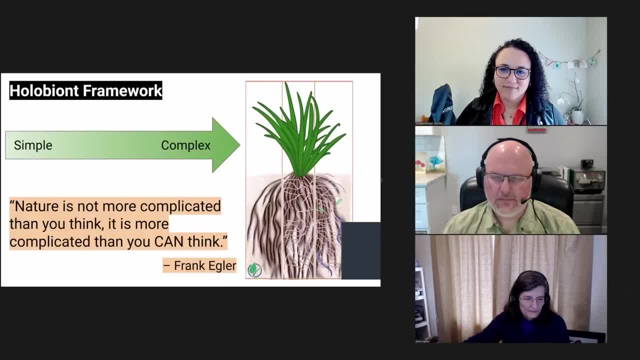 people only survived if they did things to make a thriving plant microbial holobiont network, because that was the only place that the nutrients and the productivity came from. and the future? in a lot of ways, it's not going backwards. it's taking the lessons of what the world used to be and applying all the best science. 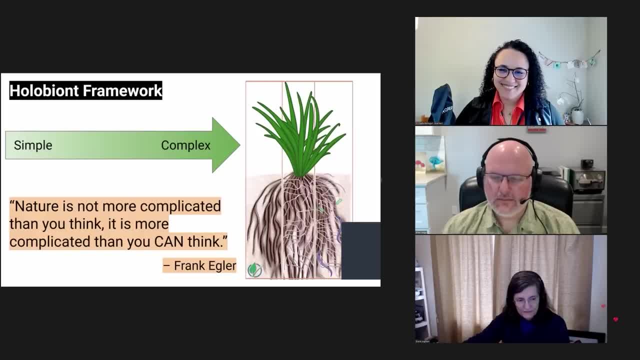 and designing systems forward where humans can really be our own like keystone species. we can expand how much life is on this planet if we want to, instead of killing all life on this planet like we've been doing here here. that was a great, uh great way to summarize that up. 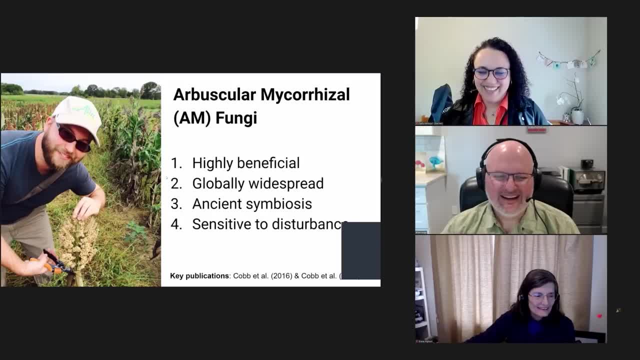 i hope this isn't weird. i feel like i'm just on different soap boxes today. but too funny, i moved you to the next slide out- excellent, uh, i'm just going to briefly mention because the next um webinar promotional i'll talk a lot more in depth about. 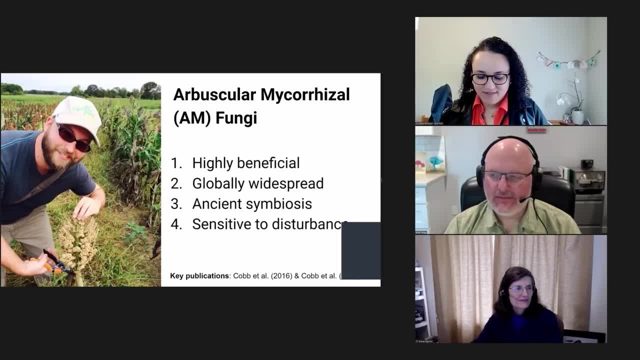 these arbuscular mycorrhizal fungi. they are a very highly beneficial, typically, connection to plants. they're one of the flagship organisms of a holobiont that's healthy and effective and they're- and they're quite globally widespread. um, it's the arbuscular mycorrhizae we 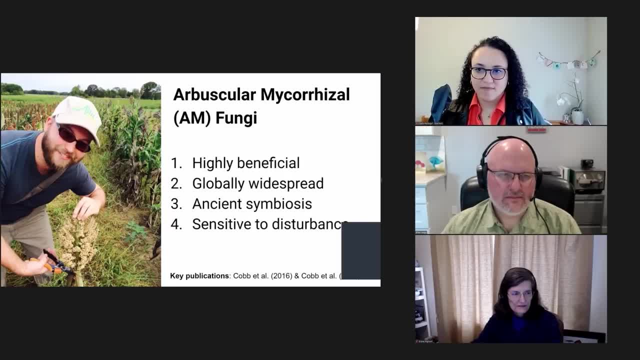 find, associating with around 80 percent of plant species across the planet. it's a very ancient symbiosis. i mentioned that some part of its lineage was probably responsible for plants being able to colonize land in the first place. it's very sensitive to disturbance and when i wanted to. 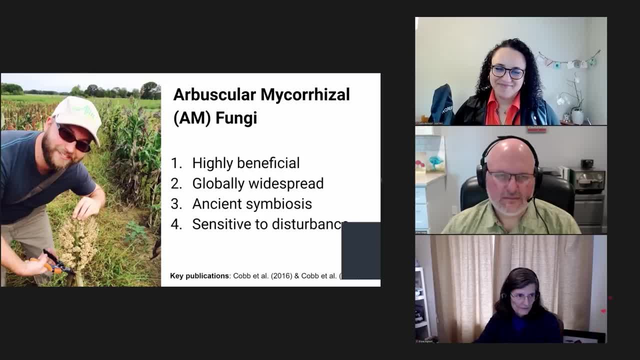 study mycorrhizal fungi in agroecosystems, i had a number of people say: what's the point? they go away as soon as you put down a little fertilizer or do a little tillage. that's never going to work. that's never going to work. and i was like, well, what about systems that don't have those fertilizers? 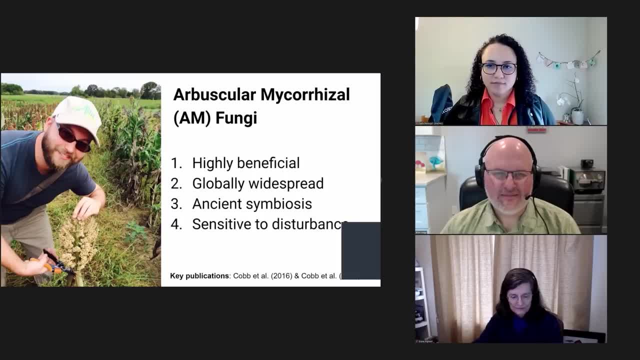 and don't have that tillage like the tall grass prairie that is, you know, full of abundance and diversity. so a few of my key papers I've just mentioned down there, and especially, you know I've asked the question through my research: have we bred our plants, even in a way that causes disturbance to the? 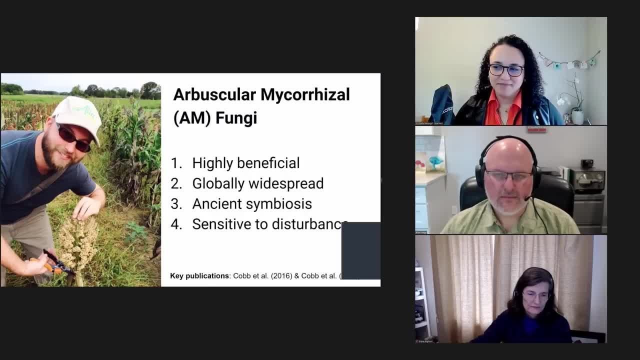 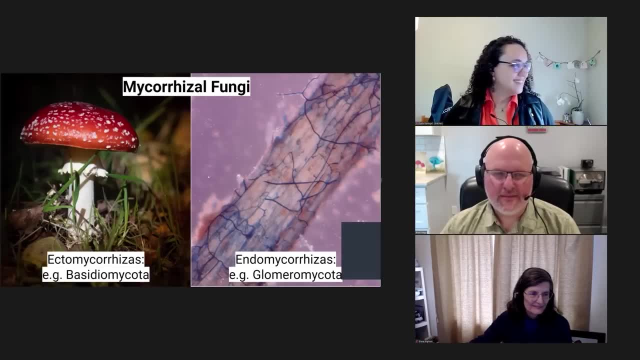 soil-food web and to the mycorrhizal relationships. So tune in next time. All right, next slide. I will say just briefly that the word mycorrhizal refers to the relationship myco fungal rhizal root. It's things that are. it's where a fungus. 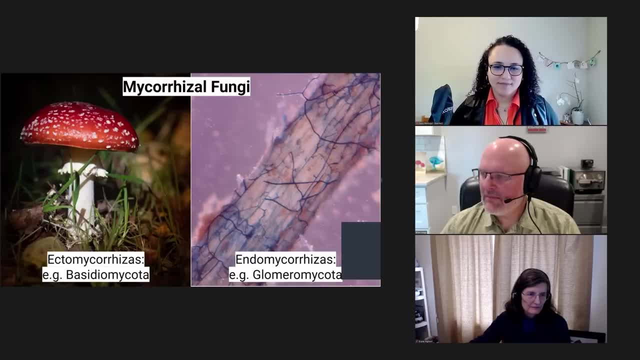 and a root live in a very mingled existence, right, Not that they're fully attached or you know, but that they're really taking a big, they're embracing each other, they're hugging, they're friends. The ectomycorrhizas make some of the coolest mushrooms. 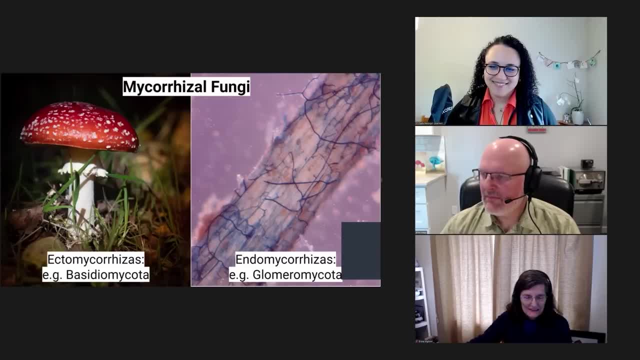 in the world And the ectomycorrhizas are very diverse. The last time I checked it was like two to 5,000 species that are estimated, but they associate with just about 2% of the plants on earth, mostly trees, And most of them are basidiomycetes. Some are ascomycetes. There's 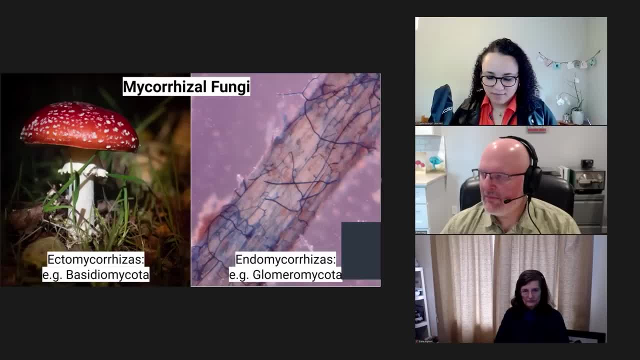 always outliers there, but the ectomycorrhizae. I see people conflate these two things or get them mixed up. The endomycorrhizas, which I took this picture of a plant that I grew and we stained them. 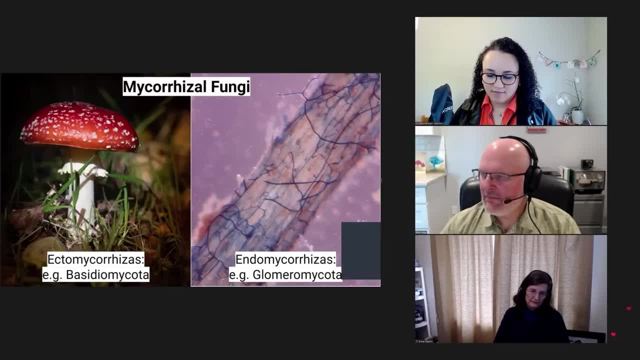 The arbustular mycorrhizal fungi, which is an endomycorrhizae. They have their own designation in the fungal kingdom We call it. most of them fit into glomeromycota and they're very different. They don't make mushrooms. 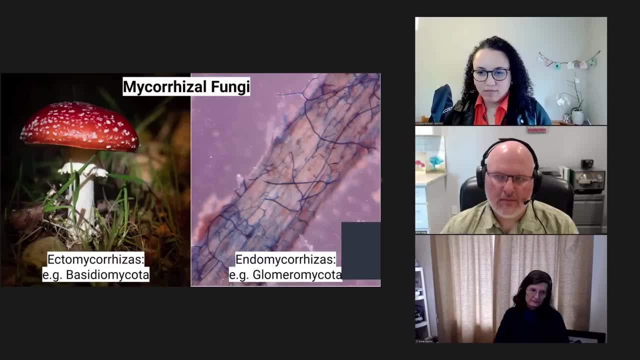 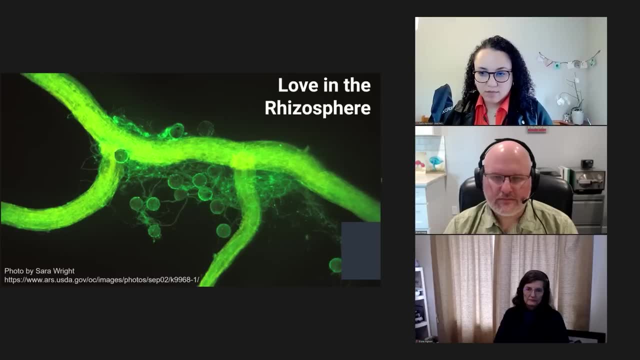 In fact, if you go to the next slide, Brian, this, this picture does a great job of showing that they just bud off spores off of their hyphal network, So the hyphae connect to the plant and then they make the next. 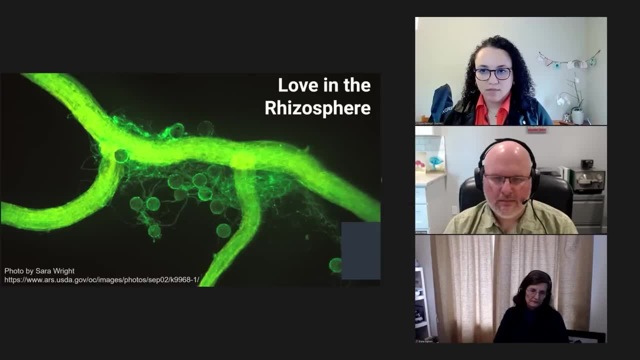 Generation. It's kind of like clones, sort of of the parent. It's not exactly, but we think they're fairly clonal and their, their reproduction is quite mysterious actually. but right there in the rhizosphere they can propagate themselves, And a lot of times the same species. there's fewer. 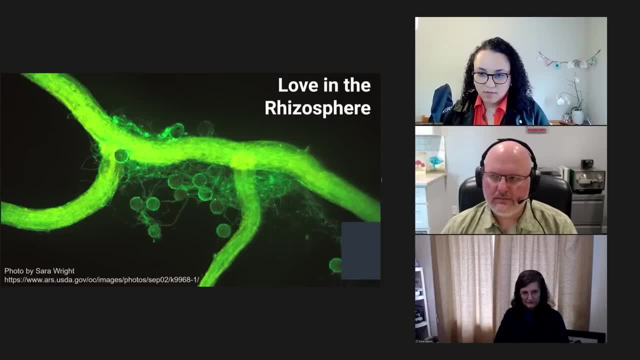 species or taxa of our muscular mycorrhizal can associate with many different plants, So people often have it in their head that one Species of mycorrhizae goes with one crop. but if you have a healthy, diverse population of mycorrhizae, 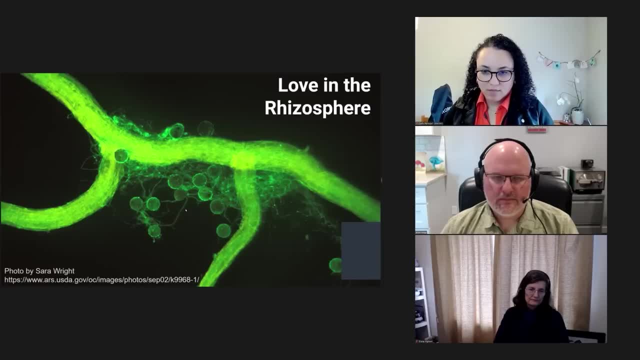 they're. they're very likely going to benefit. in many of the crops that you would grow, Brassicas are kind of iffy. There's very few circumstances. For a long time we thought brassicas didn't even form mycorrhizal relationships, but there's a few places where they seem to now. 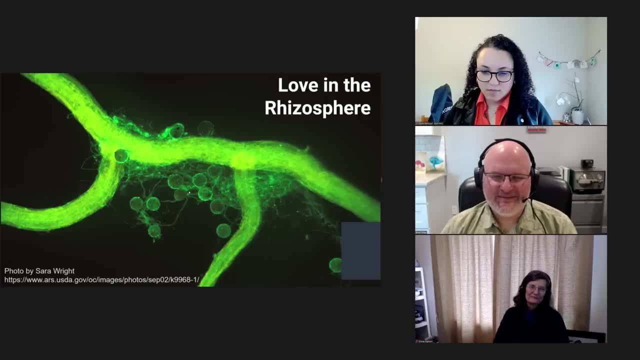 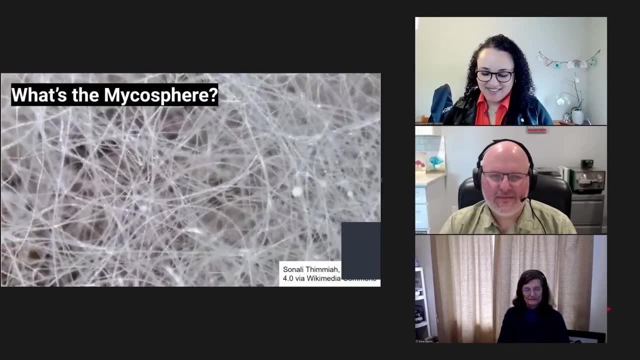 So that's just some fungi nerd talk for you, And then we can get back into the main flow on the next slide. because I said I'd talk about the mycosphere, So I mentioned the term rhizosphere, that area in proximity to the roots the mycosphere can have a much further reach into 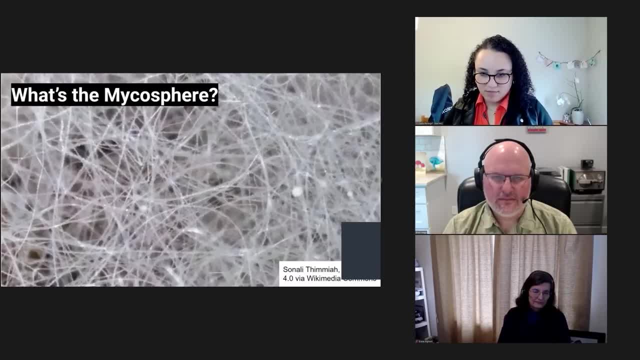 the soil ecosystem, and at a finer scale, because these hyphae that Elaine and I have referred to a few times, these filaments, they're like little spider webs or threads in the soil. They reach out further than the boundaries of the plant roots. And in fact, on the next slide, my main 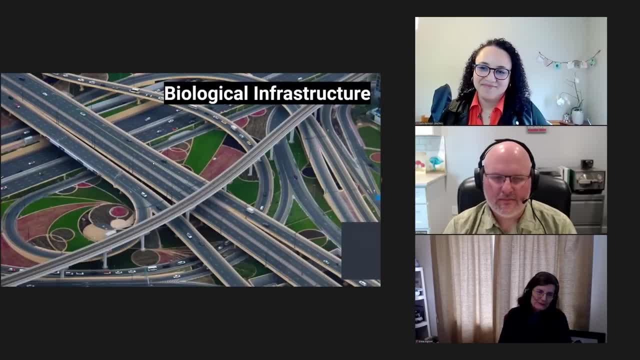 metaphor here is: if the roots are sort of like the highway or the main river, the hyphae of fungi are like the side roads or the tributaries, And they in we actually see that they carry carbon. they facilitate more life out further and at a finer scale. 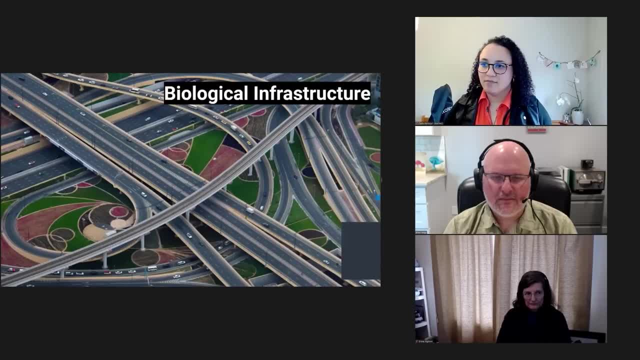 then the roots would be more fertile and they would be more productive. And so we're looking at what we do just alone, And- and I'll show some pictures next time- of some alfalfa I grew. But do you want a two inch tall alfalfa plant? Or do you want a two foot tall alfalfa plant? Because the 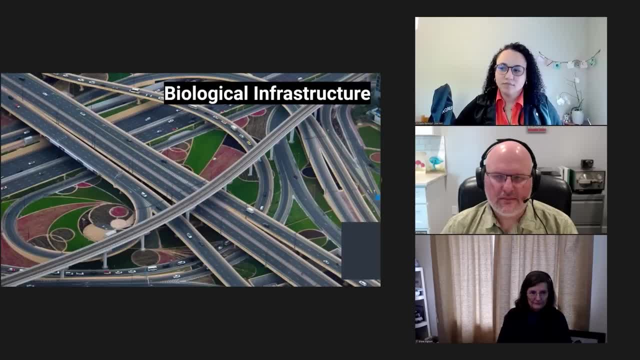 difference can be whether or not they have fungi in the same soil in the same greenhouse. that facilitation. the plant gets more nutrients, the soil food web gets fed more carbon. they are an essential component. I'll show you an example of the same work. 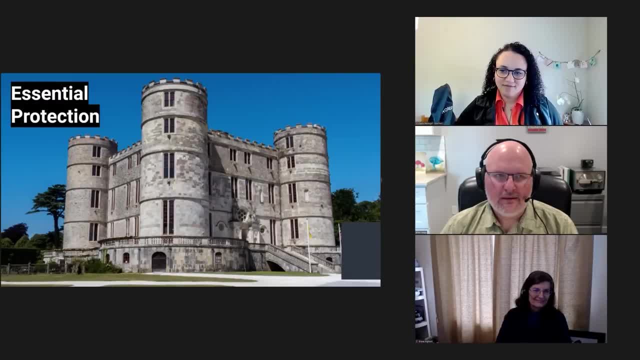 Did I miss anything? y'all? We just got a few more slides to go through. Yep, no, I think we're tracking really good. We're on to essential protection. So when we talked about dirt, in a lot of cases due to tillage and other historic things- that 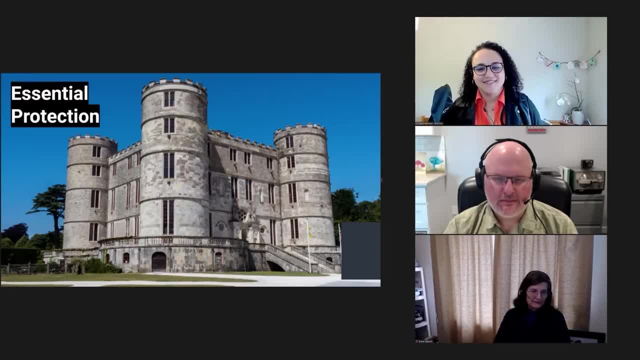 humans did. it's sort of like when an invading army came in and smashed all the forts in a whole area And then the people didn't have protection And they couldn't get. they couldn't accumulate any resources, resources or protect any resources from raiders. 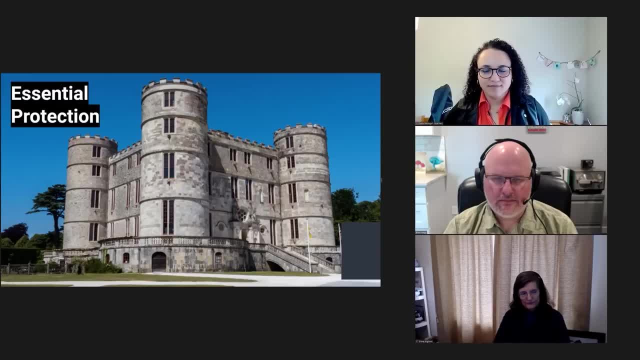 And that's what dirt is. Fungi can come into dirt and they can help through that aggregation process and through the reach of the microsphere they can help rebuild those that essential protection, those aggregates, those little tiny parts of soil where different organisms can thrive right. 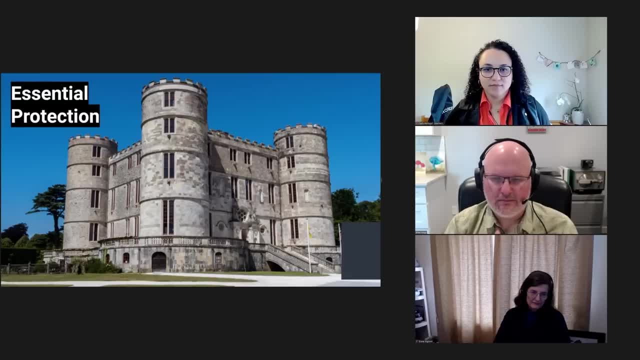 And again, this is both further out from the plants and it's at a finer scale than roots. Filaments from fungi can be much smaller than the smallest root hair And what they're doing in there is building up that structure and building those places. 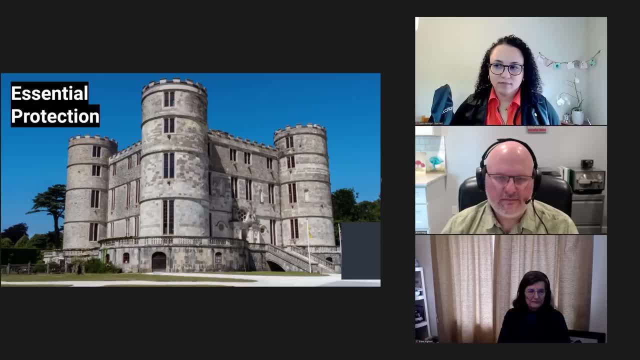 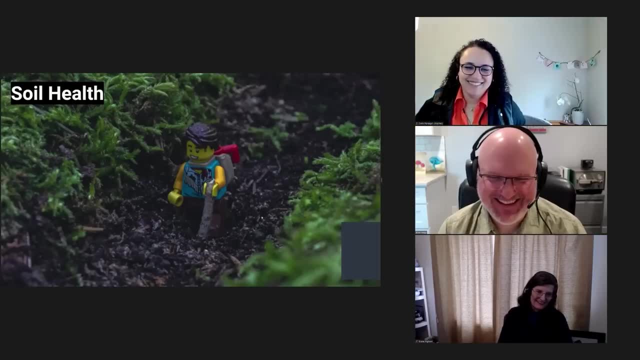 of protection. I think my next slide is a picture of me walking in the forest. Great picture of you, Actually. you know what? Yeah, You know it's not me, because of the hair and my dog is not with me in the photo. so 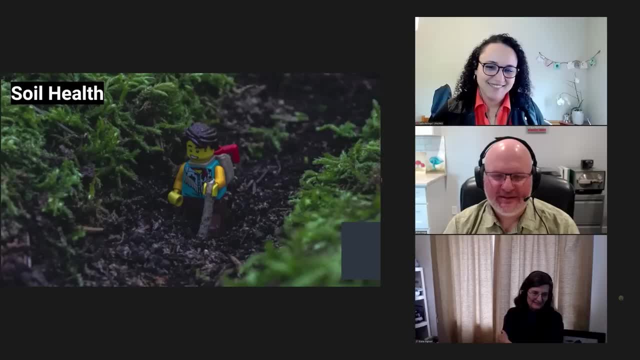 But I hope that everybody on the call today has had a chance to spend some time in a really mature, beautiful forest. I had the chance to live in Oregon for a year and I got out into some of the best forests on Earth. The soil is fluffy. 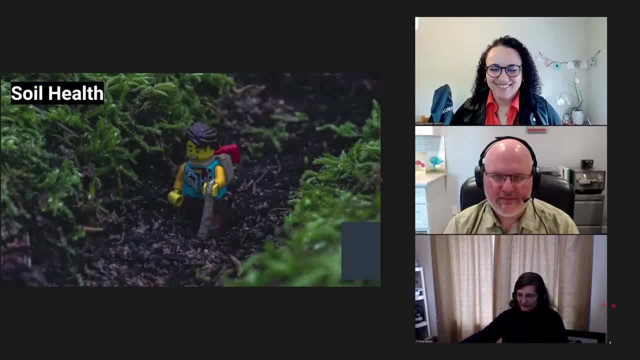 The soil smells amazing. When it rains, the soil soaks up the rain And then it holds it so that if it doesn't rain for months and months, the forest is fine. There's still water there, Soil health- if you reach down into forest soil and take up a handful and if you put 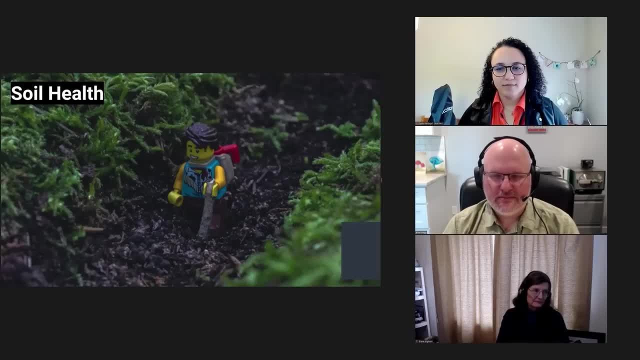 it on a microscope and look at it, sometimes even just with your eyes- you will see it's bursting with fungi. This is one of the processes of succession in ecology, that we move from systems that are more dominated by bacteria To ones that are more dominated by fungi. 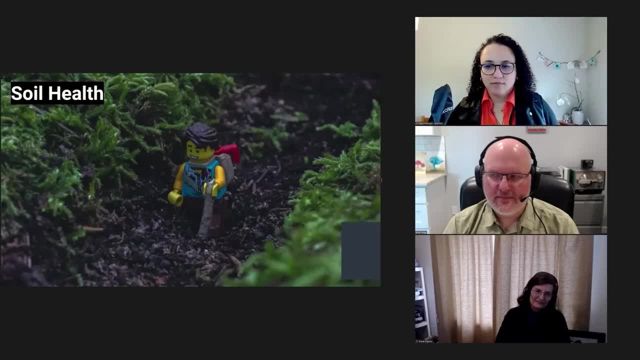 And an early successional to mid-successional ecosystem does not have the soil structure and stability and general health and wellness right. That's a big term. I know people don't always love this term, But again it's like I'll show you disturbed soil and I'll show you forest soil and anybody. 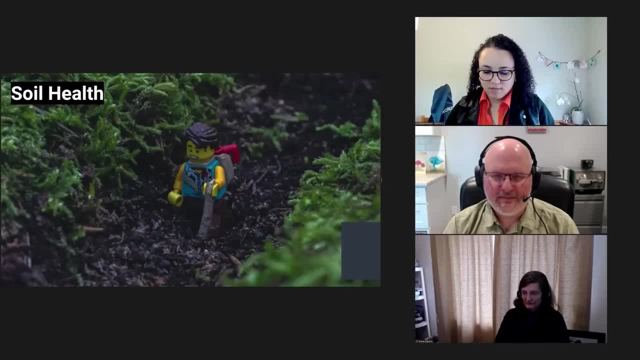 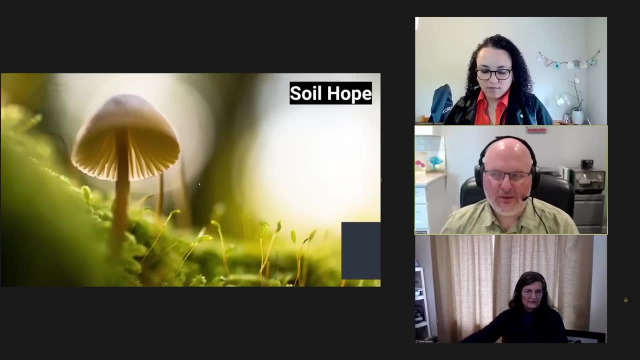 can tell that they're different, And the fungi are a huge part of why they're different. All right, I think we're on to soil health. This is the last slide. I added this yesterday because I listened to a podcast with Peter McCoy, and he's one. 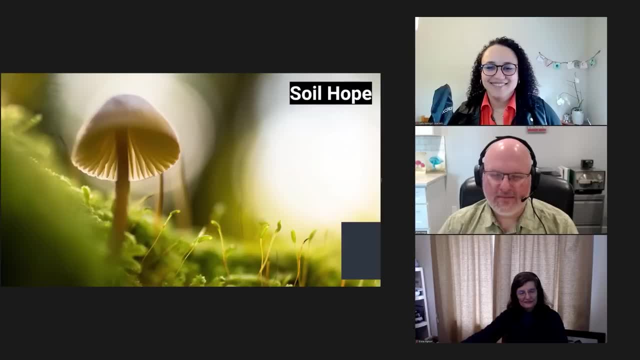 of our favorite mycologists and has been on webinars with us before. And Peter inspired me so much because he said that, when we consider all of the threats that we face to humanity at this time, you know what some people call the poly crisis, where 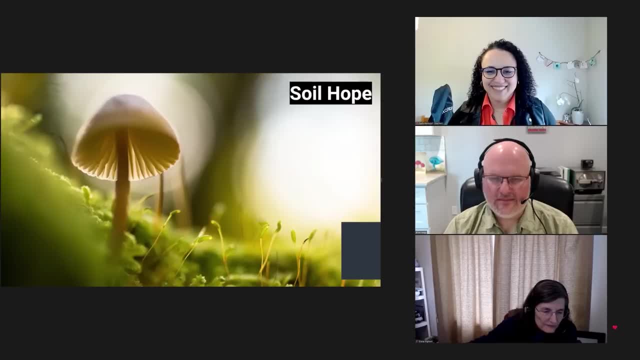 there's many crises, crises, crises, crises happening all at once And it seems overwhelming. And it's it's not just our food systems and our way of life, It's our whole society that feels in peril. If we look at fungi, 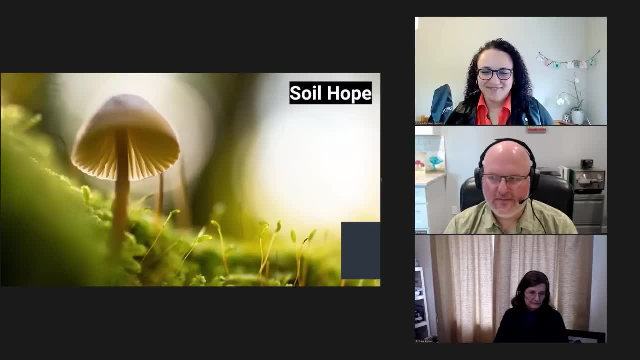 And the fact that they've been here for over a billion years. They've been here for over a billion years And the fact that they've dealt with so many global scale disturbances in the past, like the asteroid that took out the dinosaurs, And they just sloughed it off- and use their immense diversity to say: we found a solution. 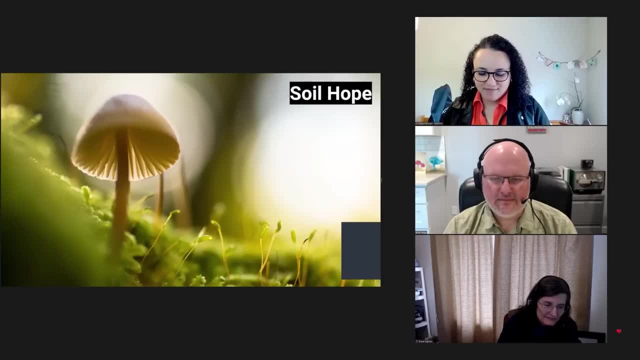 we can rebuild this thing, we can make it better. It gives me so much hope to think that if we partner with this piece of the tree of life, It has the wisdom that we need to tackle our problems. It can clean up environments that are contaminated. it can put carbon back into soil. it can provide. 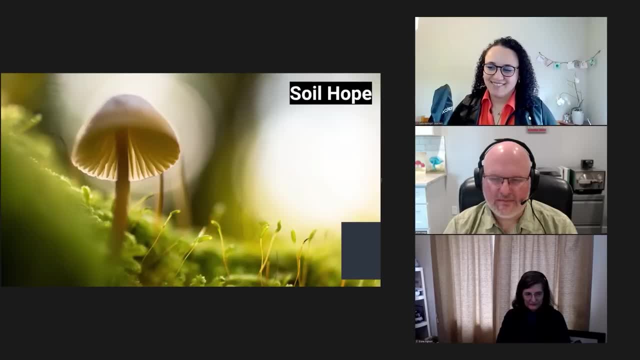 an abundant food supply that doesn't require these chemicals that destroy rivers and streams. It is this, this kingdom, this part of the tree of life. It has so many answers for us, And I'm here to tell you today That we have not begun to figure out how much is in there. 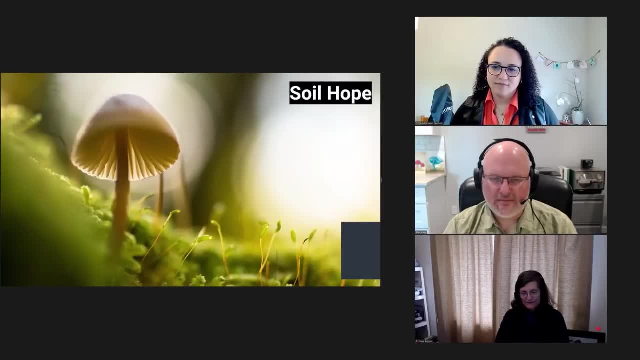 I read a paper recently that said about 150,000 species of fungi have been defined, described by human beings, And the estimates range from 2 to 14 million species that exist on this planet. They have the answers. We should look to them. 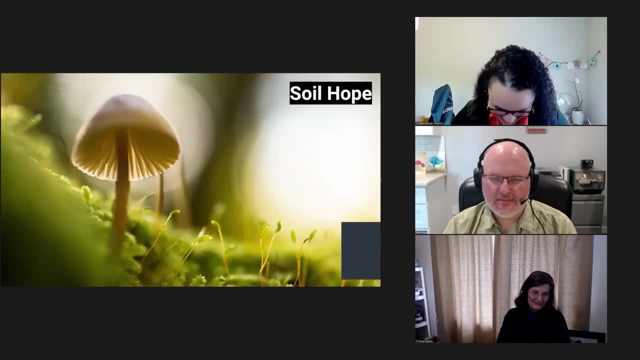 Humans are not as smart as fungi. They haven't been here as long. They don't have all the answers. We have to humble ourselves and look to the fungi for our hope. Very well said, Adam. What a fantastic presentation. Thanks for bearing with me on the 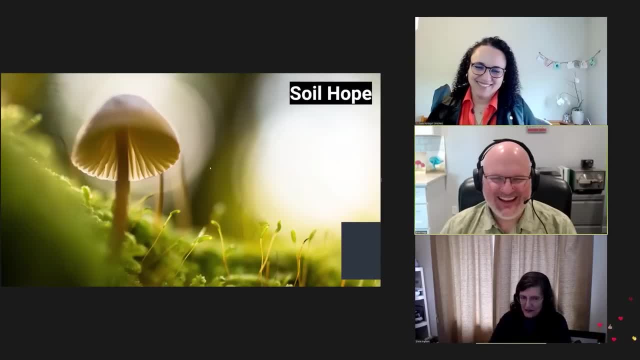 No worries, Easy peasy. I guess I'd like to add just a little bit for all the other organisms in that food web. Fungi alone aren't going to do this, but together we can turn it all around. We haven't lost all of the diversity yet. 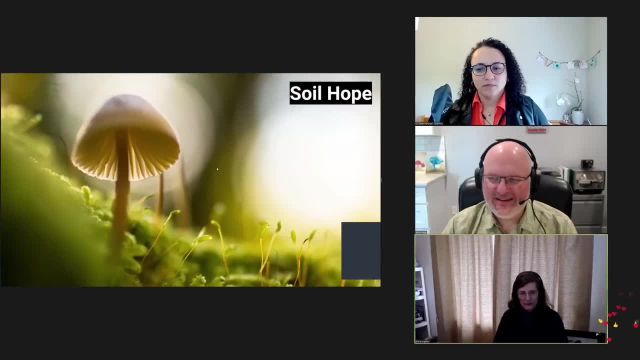 We're working on it, but we've got to remember all parts of the food web. Absolutely, I totally agree, And you teach me new things about the food web every day, Elaine, So thank you for that, because I fall more in love with it every week that I'm here at. 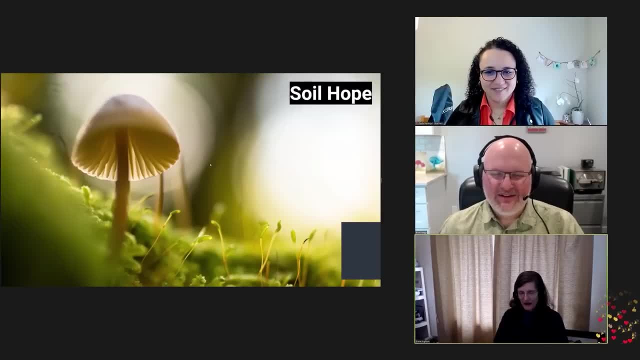 this place, Yep, And I'm glad to have you around because you always correct me so kindly. Teamwork, It's so fun. Yeah, It's a part of the whole teamwork at the symphony, And my students always tease me because every session I just tell them that, oh, this is. 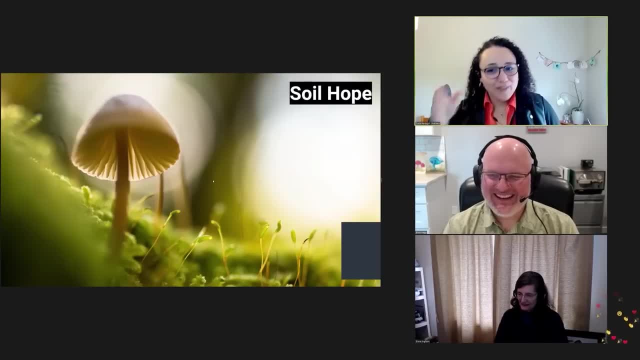 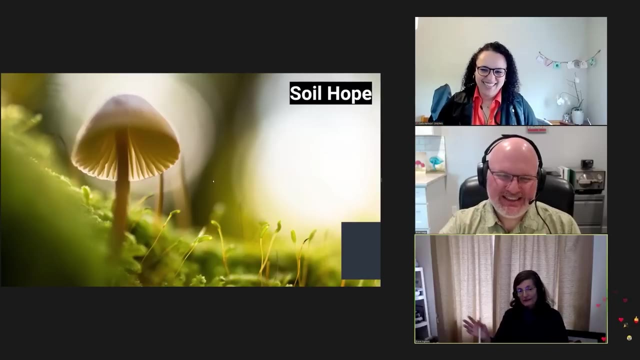 my favorite, Just like. hey, Carla, can you just say that all of them are your favorite ones? I'm biased, but I like all those fun guys as well as fun gals. That's right. Okay, I'm going to move us along to talk quickly about our April promotion, and then we're. 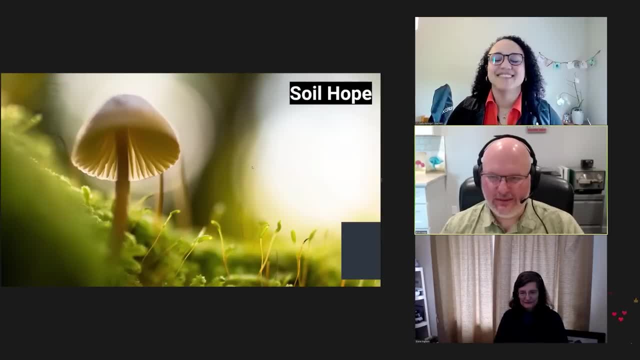 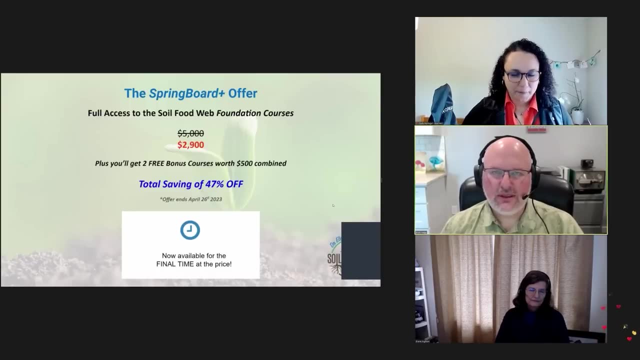 going to get to the Q&A And I tell you what we have had. a lot of questions come in, So fantastic. So first of all, before we get to Q&A, let's talk about our April promotion. This is the Springboard Plus offer. 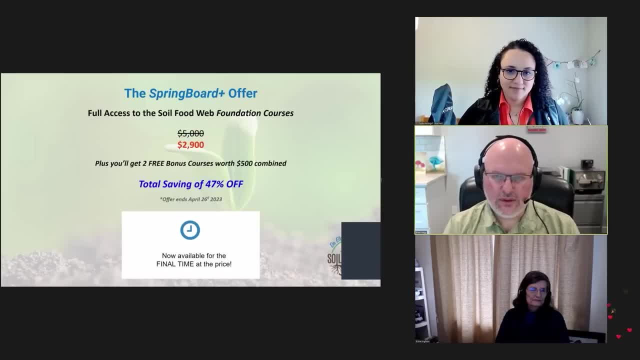 And so you can see from the Soil Food Web Foundation courses there's a really significant discount, about 47% off, And the offer is going to end on April 26 of this month. And before we get to the Q&A, let's talk about our April promotion. 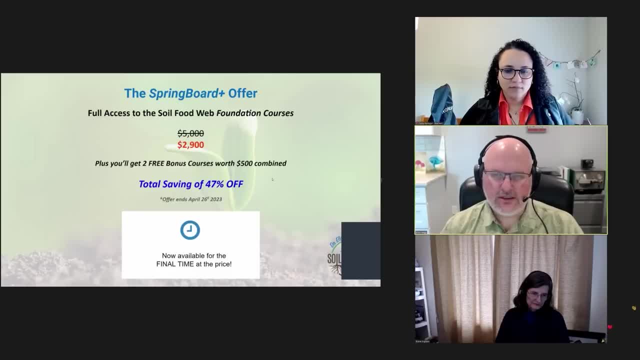 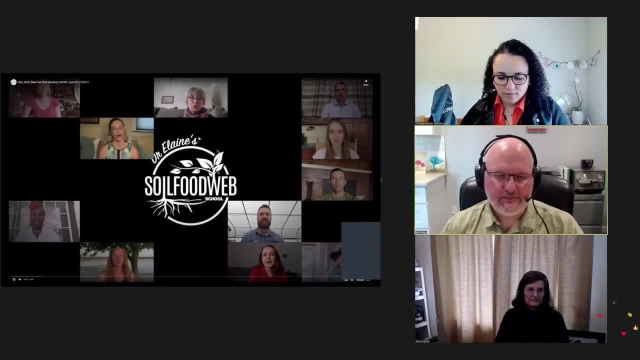 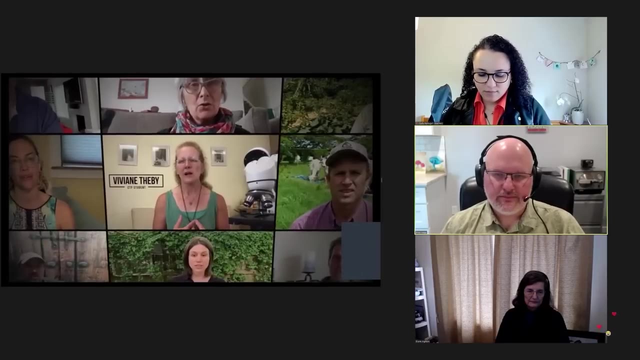 Okay, Before we move to Q&A, let me play a quick video just to kind of describing the foundation courses and what this promotion is about. When we're talking about the soil, we're talking about the base of everything. Even our health depends on the health of the soil. 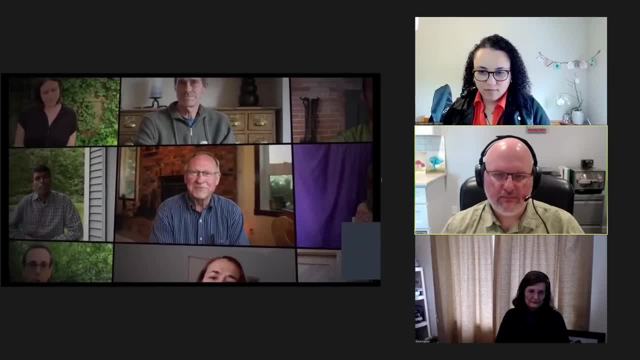 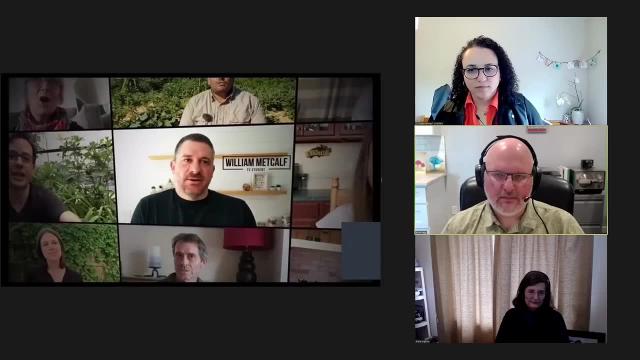 All the sickness and disease leads back to where you live, how you live and what you eat. People don't want to use the chemicals, but they don't have any other way. They don't have any other way. It's not a desire problem, it's a knowledge problem. 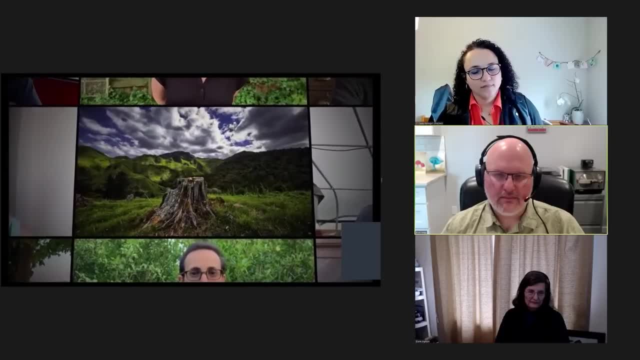 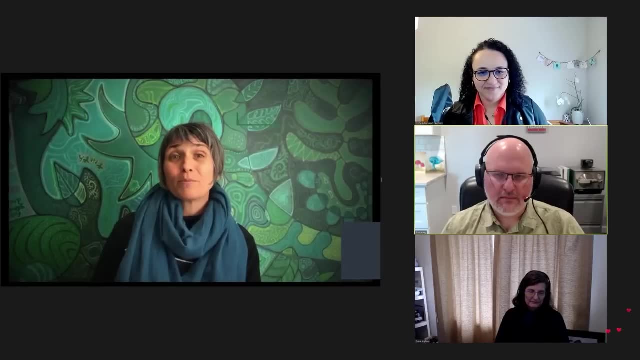 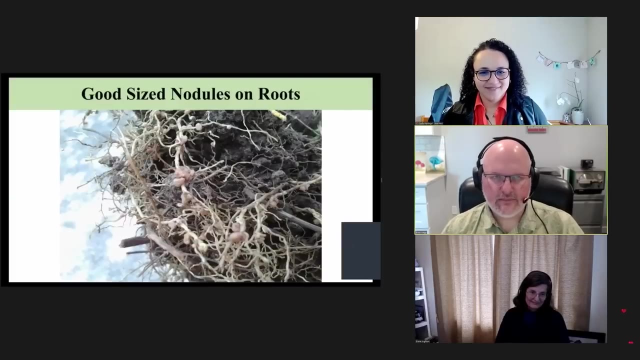 Everyone needs to have some awareness of what our Earth is experiencing right now and how we can make a big change. I find that this information hasn't been taught to me and I had to get off my high horse And, even though I have a PhD, I feel like I'm totally under-trained. 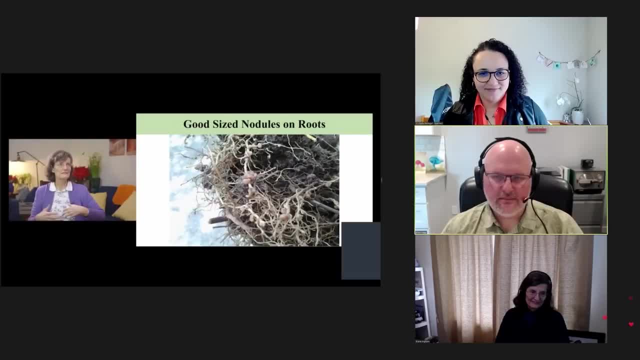 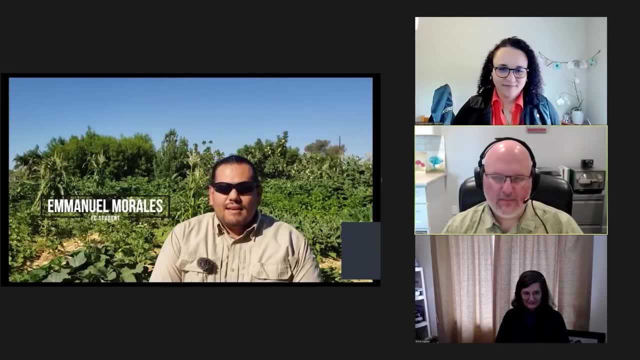 I feel like I'm learning more with this program than I have with in-person classes in the past. I've taken classes on microbiology before, But this course really makes it easier. It makes a difference in the way that a story is put together. that unveils the relationships. 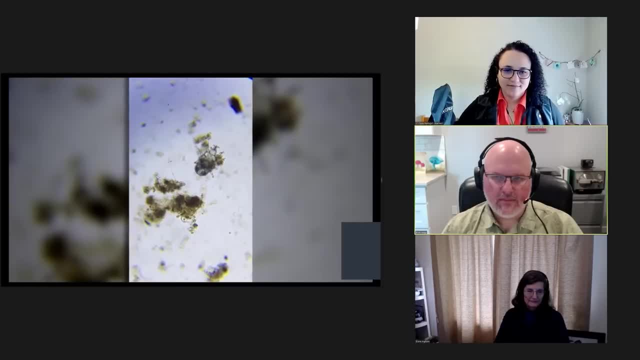 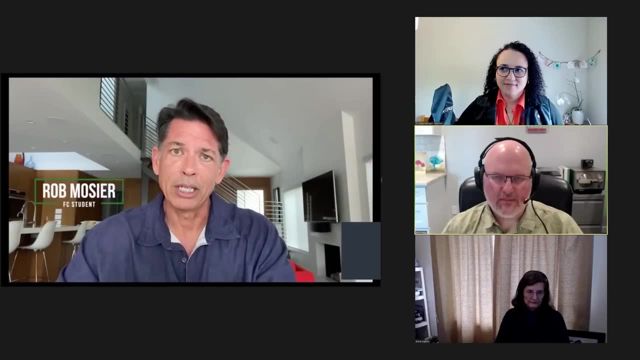 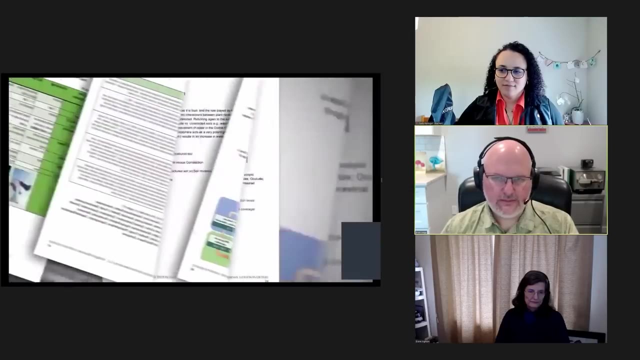 between plants and all those beneficial organisms that we just cannot see without a microscope. If you're looking for something that does a deep dive into soil biology, this is it. It is just an incredible knowledge base and it's really relevant to what's going on, right. 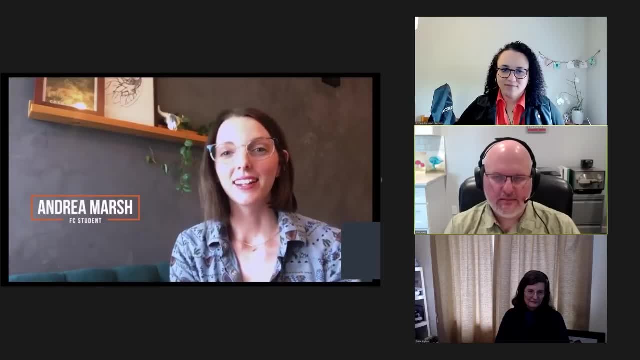 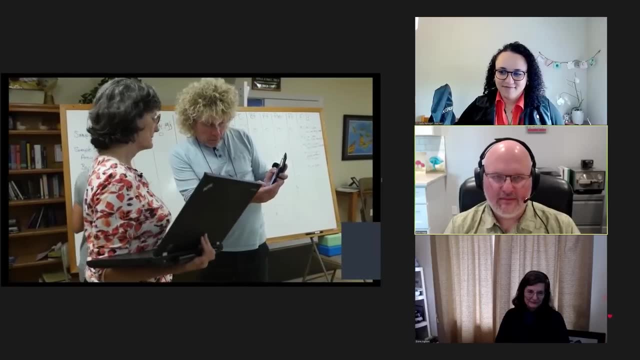 now in the world. Without it, the only way I could have gained this knowledge would have been by dropping my life and going to school, And that just wasn't realistic for me. But Soil Food Web has made it possible for me to build a meaningful career in land restoration. 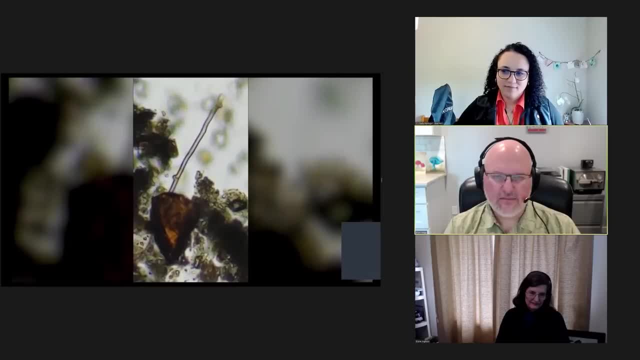 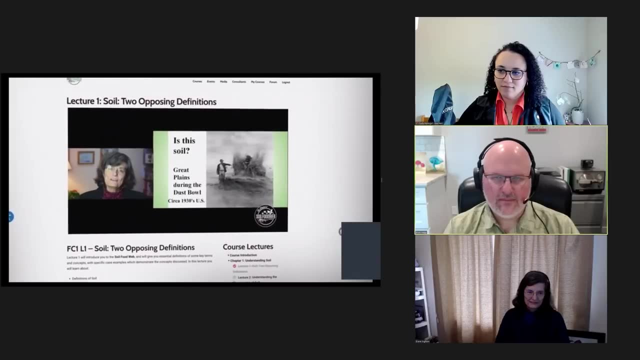 I was really nervous that I was going to put quite a bit of money down and not get that bang for my buck. But once I actually got into the FC courses I was incredibly impressed with how professional they are and actually the level of education you receive. 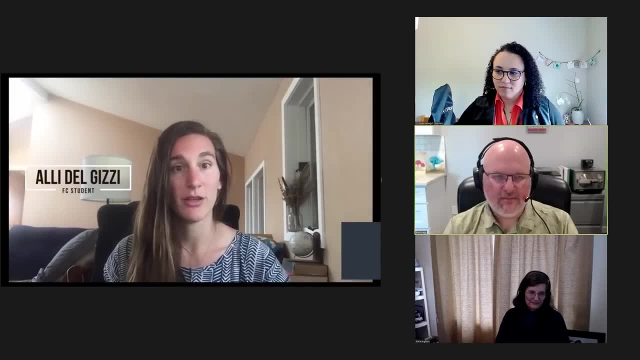 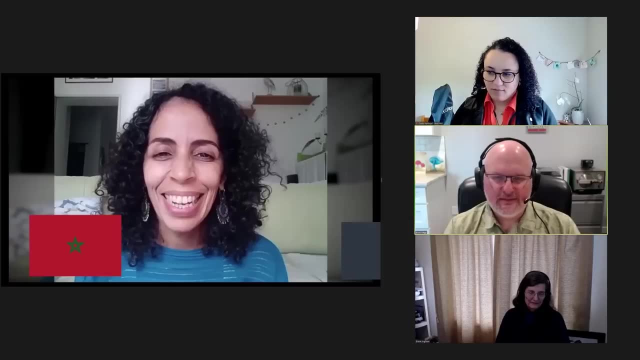 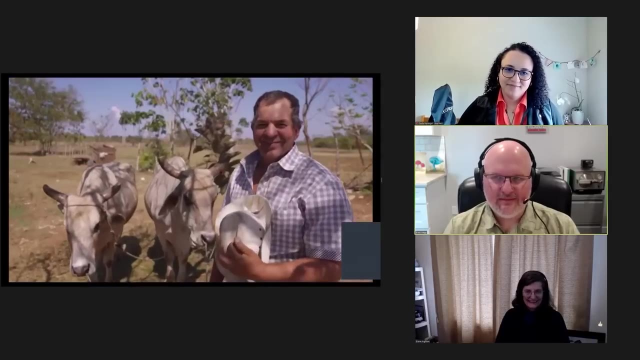 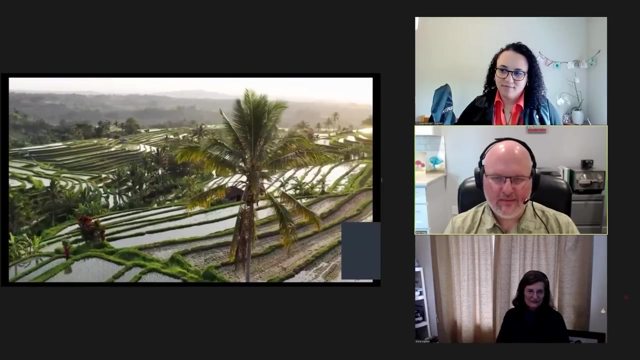 This is the career path I've been looking for in the biological community and I was having trouble finding. It's absolutely amazing to me that there's people with their same approach to life wanting to do better things all over the world. What the course is doing is actually getting those people together. 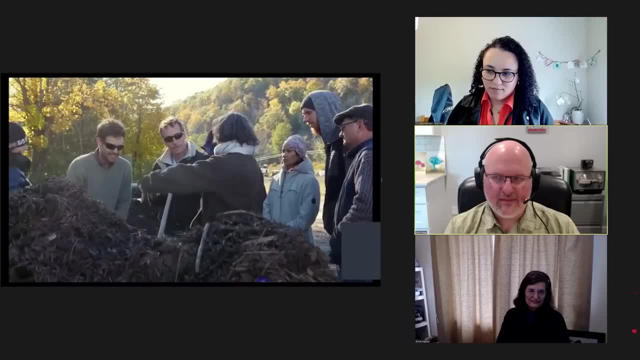 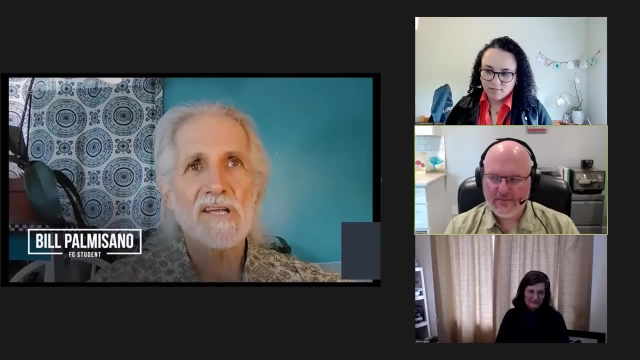 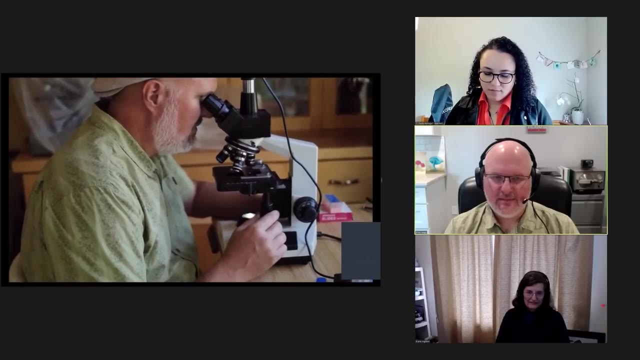 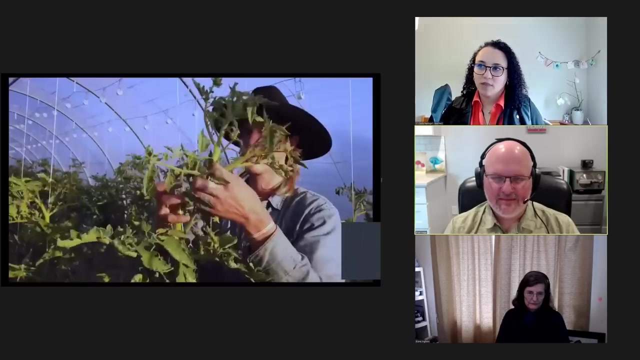 In terms of the connection to the network, I have found just an environment. It's an environment of camaraderie and cooperation. They want you to succeed and they bend over backwards to give you all of the resources to have you succeed. At the Soil Food Web School, we train farming professionals and ordinary people who are 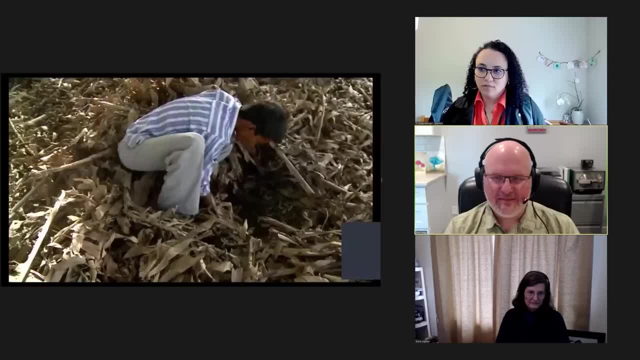 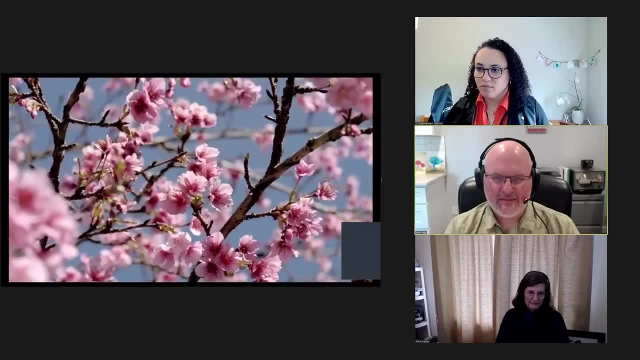 passionate about the environment, Our students are able to help make a real change to the way that food is grown in their communities and to how the earth is being treated. Spring is in the air and there's never been a better time to launch your career in. 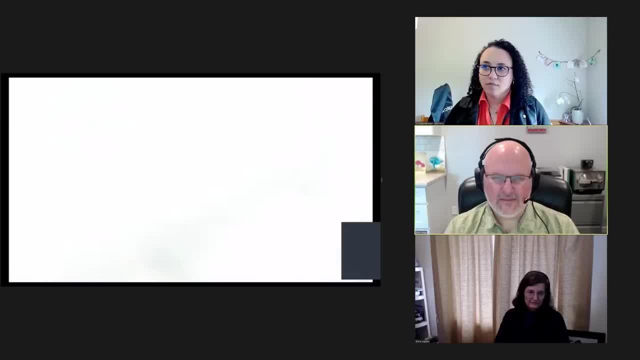 soil regeneration than right now. With the SpringBoard Plus offer. you can register for the Soil Food Web Foundation courses for just $2,900, and you'll get two free bonus courses, saving an incredible $2,600, or 47%. 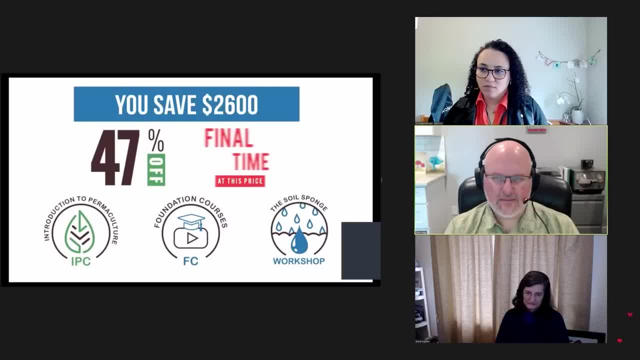 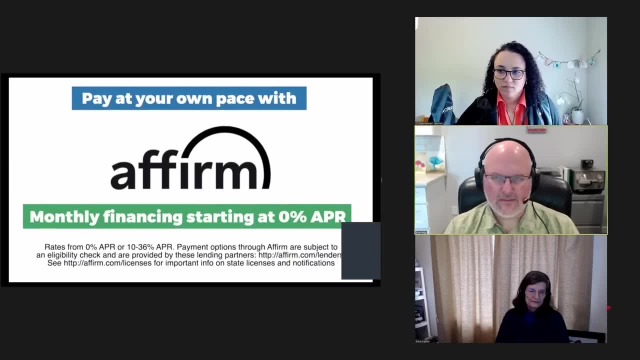 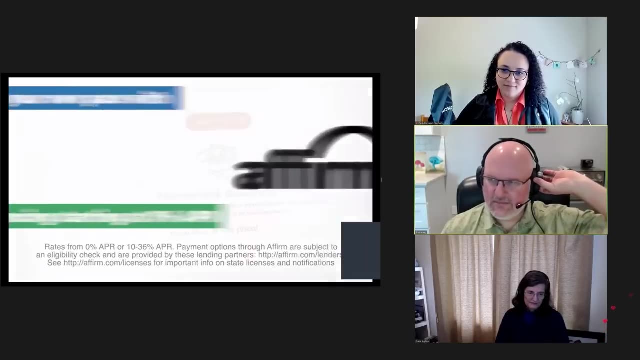 off the regular fee price. This is the final time that the SpringBoard Plus bundle will be made available at this price. Financing options are now available so you can pay at your own pace. with Affirm And remember, the Soil Food Web School offers a 100% money-back guarantee, so if you're 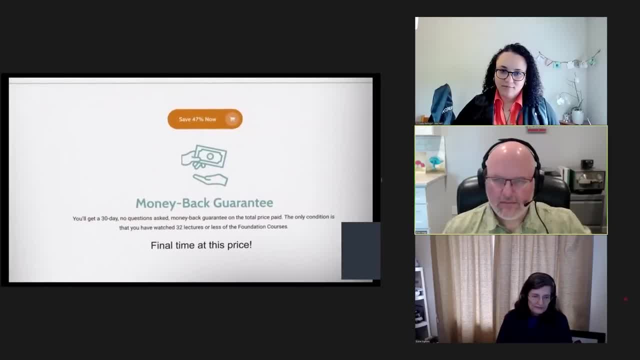 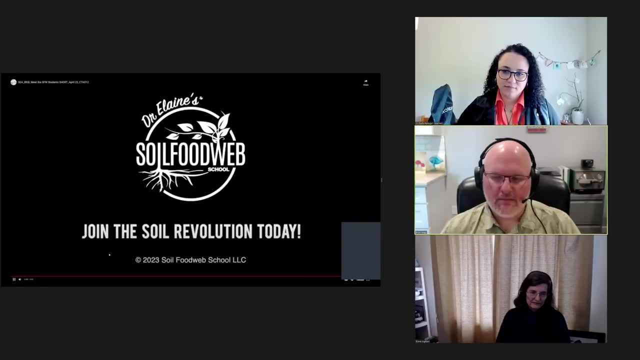 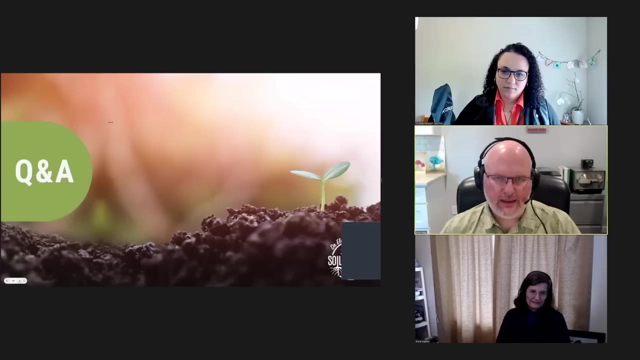 not completely satisfied. you can get a full refund in the first 30 days, so long as you've watched 32 lectures or less of the foundation courses. Start your new career in soil regeneration today. All right, the panelists. I think we're back here. 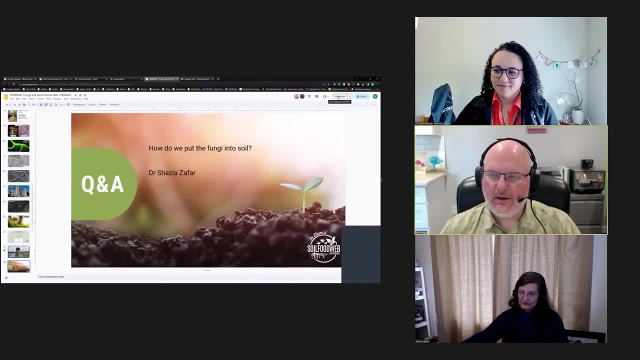 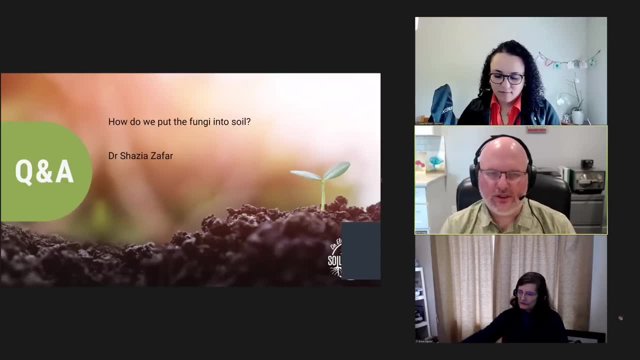 Let me go ahead and get our Q&A set up. All right, the panelists, if you can go off of mute, let's take a look at our first question. This question is from Dr Shahzad Zafar and the question is: how do we put fungi into? the soil. If it's not there, how do we get it there? Well, you want to grow some good fungi in your compost. You do have to make certain that you select for the conditions that will allow the beneficial fungi to out-compete consume. That's right. Consume and take care of the competition, so you are getting a compost that has the beneficial organisms in it. You can't be anaerobic When you think about plants of the terrestrial level. all of them are obligately aerobic. The terrestrial plants just don't tolerate the waterlogged or the anaerobic conditions. So we first want to be making certain that we gather all of the fungi, all of the bacteria, protozoa, nematodes from the biome. So you want to take small samples, bring them back to your compost pile. inoculate mix. it through the whole pile And then let the heat and the conditions inside that compost pile that will prevent the bad guys from being able to live, Okay, Okay, They're not going to be able to make it through the conditions that they had to experience. 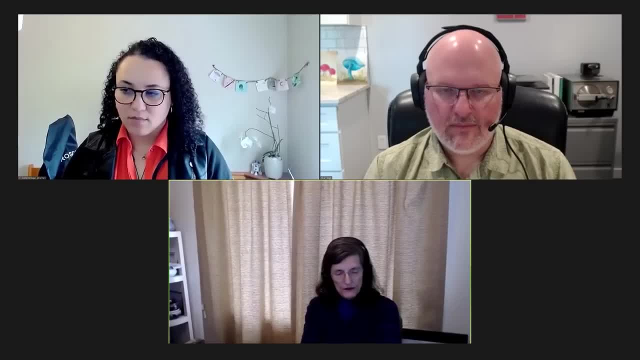 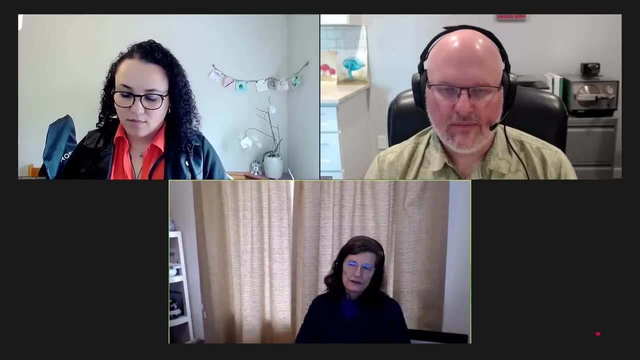 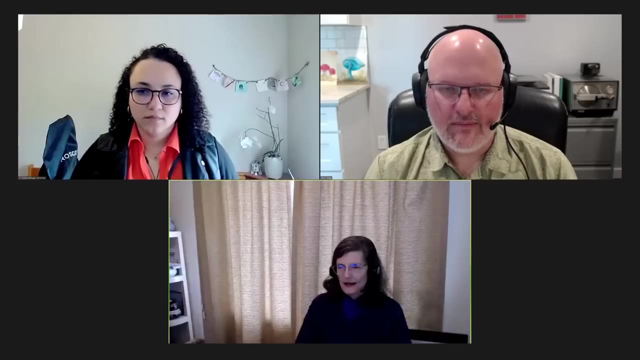 So we've got a material now that you can feel safe about applying to your different parts of the soil, of your ecosystem. You've got that medicine, if you will. I mean, I always kind of shudder when I use those terms, but it gets the idea across pretty. rapidly. We want to put down maybe just the barest dusting, so somewhere along about one ton per acre of your system that you want to bring along so that you get these organisms applied to the soil surface. Now you can't leave things at the soil surface, You want to get them to move into the soil. So come along with a really good compost extract. We're going to just use the motion of water bubbling up and through a bag where we've got our compost in. And we extract most of the organisms from that compost. They're now in the water. It's a lot easier applying a a liquid than it is to apply a solid. So we you know there's any number of different ways of applying that extract. You just have to make certain that once you've extracted you get out and you put those organisms on your land, or you're going to have to have special equipment to try to hold the compost extract, try to maintain it in an aerobic condition. 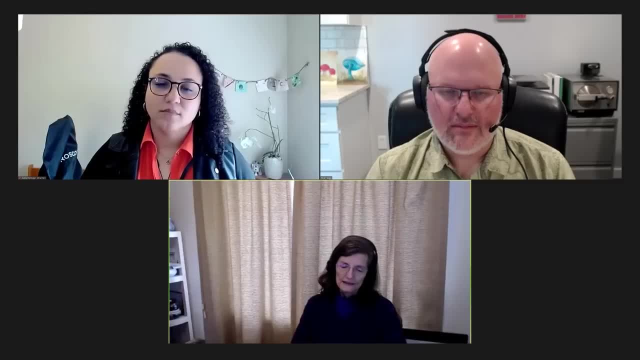 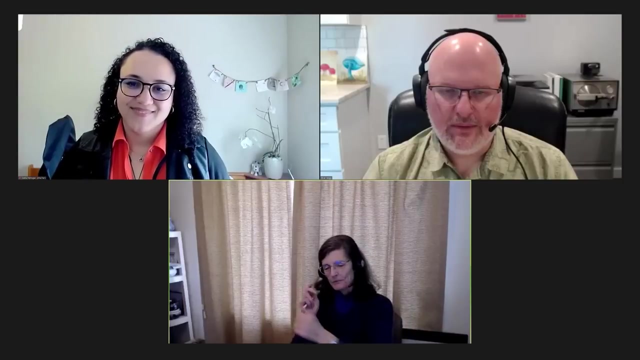 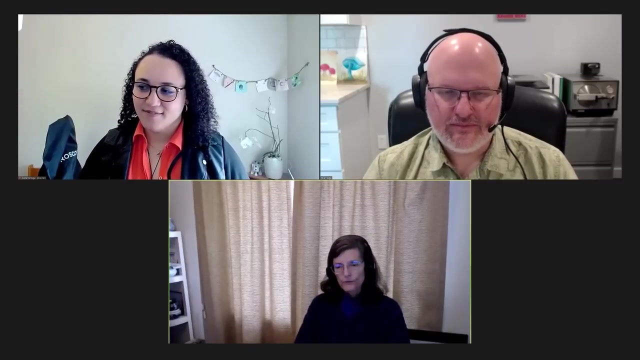 Which is possible, but it's going to cost you money If you just make your compost extract and go out and put it out. there's no Equipment- Yeah, so engines, whatever- to mix that material. So we'll be able to hold it maybe for an extra 24 hours, 32 hours, something like that. But you want to get this material out as fast as you can. Because while it's sitting there in your house or in your garage, it's such a wide open area that many of the predators in that system will wipe out Some of the good organisms That might have been present in your system. So you want to make it and use it. Compost teas, typically the same thing where we're going to add foods to that water, So that to that extract, so we can increase the organisms that are alive and active at the conditions That you'll be the organisms in the compost extract. compost tea, sorry. Compost tea will be able to grow on the leaf surfaces, on the bark, on the flowers, on the fruit, on the seeds. whatever plant you're trying to deal with, You want coverage to protect your plant from those disease causing organisms, from things that are going to be attracted to leaf material that is stressed or unhappy, unable to get the full nutrition that it requires. You can save, prevent the damage to those leaves, the reproductive organs of the plant, So that you get the organisms back out doing what they're supposed to be doing, in the right balances. And so when we start off with perhaps very a real high level, 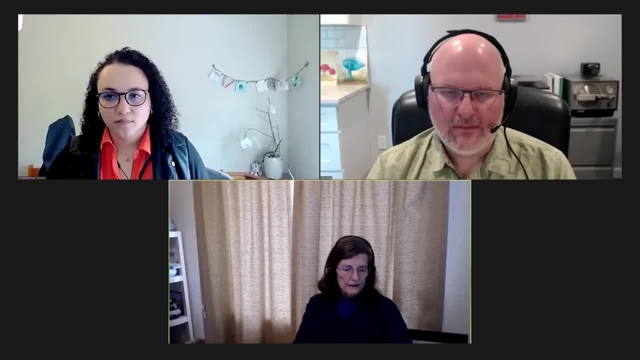 We're going to start off with very, a real high level. We're going to start off with very, a real high level Because a rice flower has a. they have red and a a lot of white leaves And they're supposed to find it. 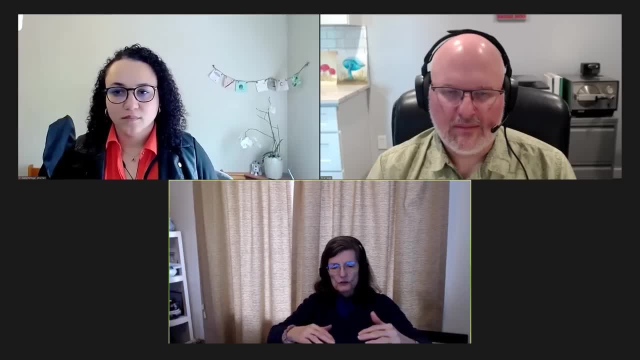 So that they find what they need to do. And you've got a plant that has to grow one to one full, And you've got plant that has to grow one to one full, So it's good to start off with. I can help you. 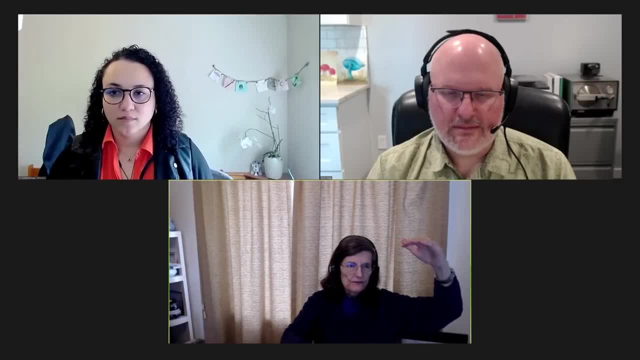 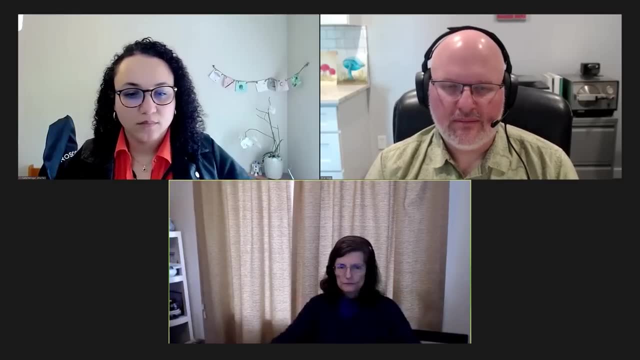 You know, now, when you see you have a variety of activities, The roots right, You're going to start smiling. You know you're going to say, well, you know all of those ْ. Yeah, I wanted you to swing. But my answer is: you have to have the roots you know, and the bushes. When you're trying to grow vegetables, you want it a little bit on the bacterial-dominated side, because you're making the conditions in the soil such that the plant you want to grow. 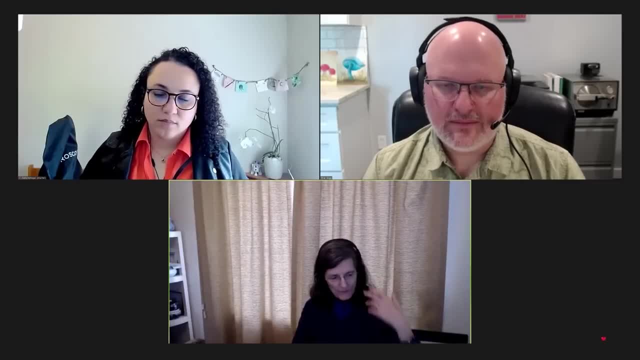 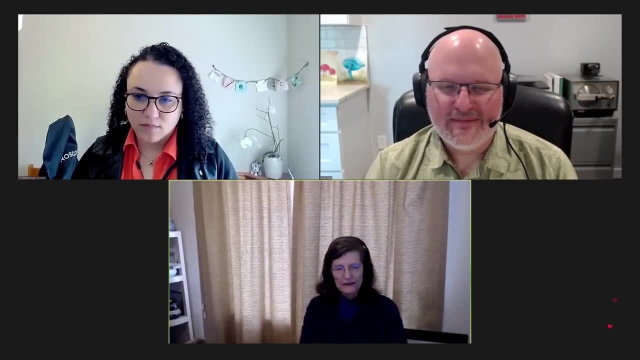 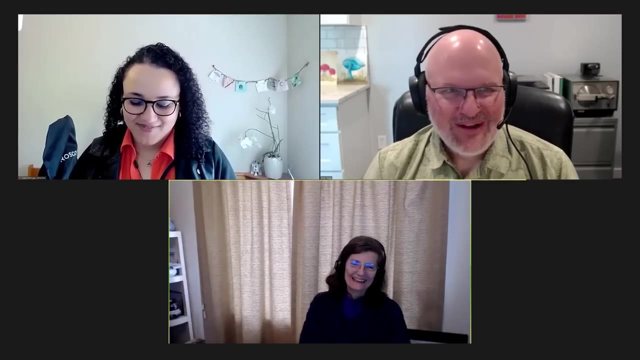 will be able to give you its best genetic steps. you'd have the best you can in the conditions that you're in. So did I talk fast enough? That's great, I think. the only thing I would add to that was we kind of mentioned it in Adam's presentation. was around the bioregionality And when we're making compost, that's one of our primary vehicles that we use actually and not get the soils with fungi is to go out into your local environment, find healthy ecosystems and take very small amounts. You don't have to go out there and load up a truck full. You're taking handfuls or pinches of the humus, the organic matter that's breaking down. That already is really well inoculated with a lot of the different organisms. 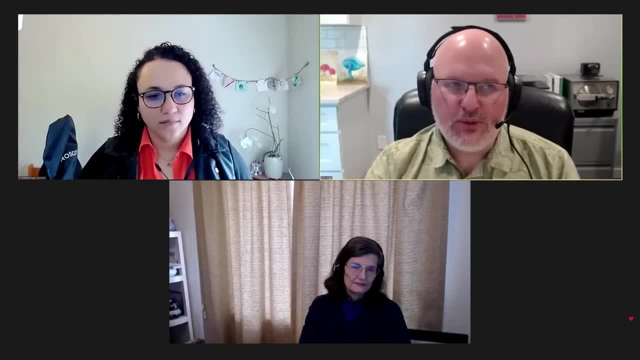 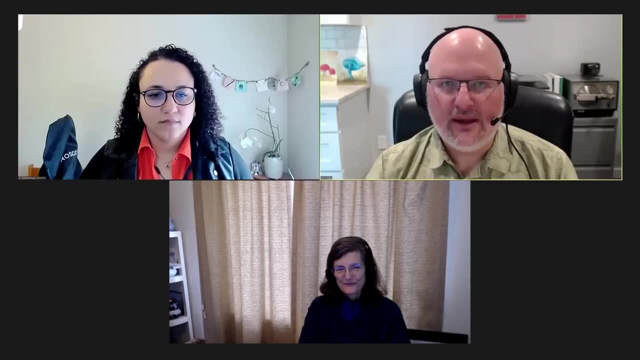 both fungi and predators and nematodes and so forth, And you bring that into your composting operation. So there you're really trying to enhance that indigenous microorganisms that are going to be set for your climate to be in your compost. Getting back to bring the tapestry to the field, right, Yeah, And that way you don't keep going out to those places and collecting every time, because you would pretty quickly Take up all of that material and you wouldn't have anything to go back to. So you take one sample and you see if you've got the massive diversity in that compost pile. You might, you know, do a second inoculum to your second pile, but always put an inoculum from the first pile into all of the. you know you might make four piles: the small size if you're small scale, If you're doing four windrows. you want. you want to inoculate with that first batch of compost that you made. It just gets better with the second batch that you make with that. with it You just keep increasing that diversity and then maybe go out and check to see if there's any more diversity. 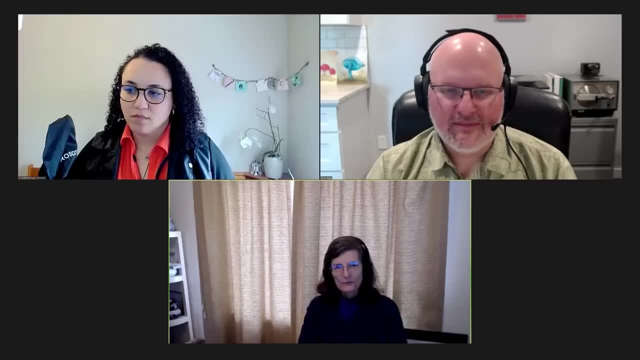 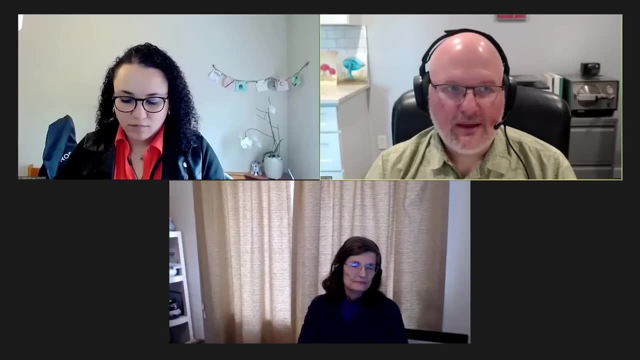 that you can add into the system, so that you keep making this just the best that could possibly be. Yeah, Okay, Carla Adam, anything else to add before we move on to the next question? Yeah, Dr Alain. like always, this is what comes. 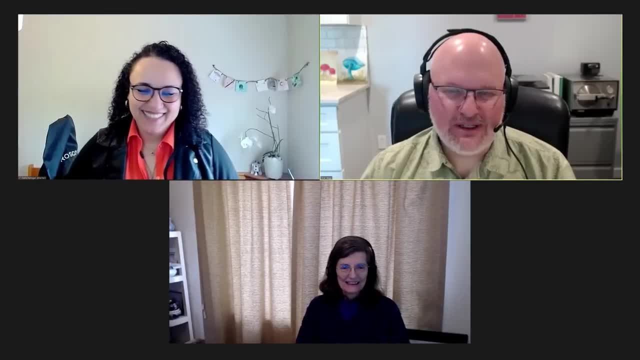 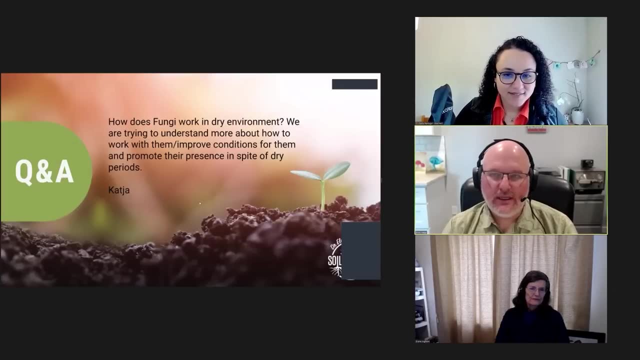 Exactly. All right, let's move to the next question, And this question is from Katja, And the question is: how does fungi work in a dry environment? We are trying to understand more about how to work with them and improve conditions for them. and promote their presence in spite of dry periods. Well, it's probably not any different than any of the other organisms that are in your soil. They've all got to be able to deal with changes in temperature and moisture and all of that, So they will always try to build an aggregate around themselves. They're protected. from some of these wild swings. So you know, make certain that in the springtime you've got these organisms already in the soil. So the instant you start to get snow melt, get the inoculum out there, get that compost out there. You want to maybe make extract. so that that extract 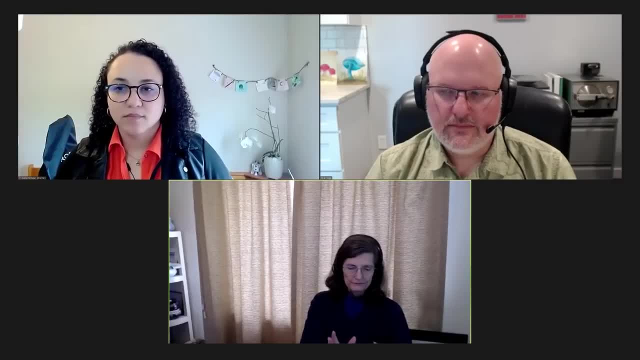 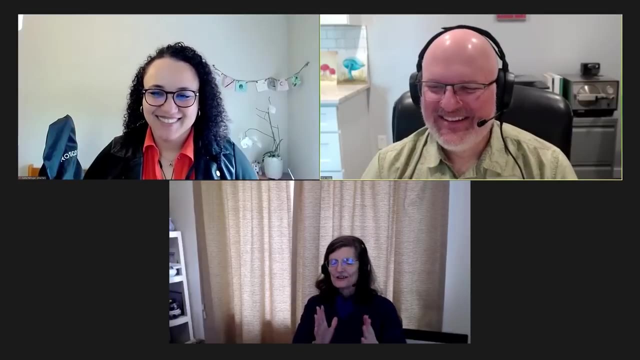 goes on the surface of the, you know where you're going to put the seed into the ground. I love my ability to not remember nouns. Those are my the biggest problem. So down the furrow, there we go. So we put a compost extract on the ground right in front. 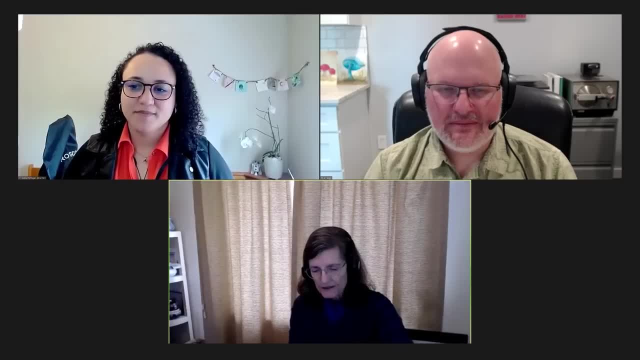 of where we're going to drop the seed, right on top of that biology. So all as soon as that seed germinates and grows, it's going to get totally inoculated by all of these good organisms. So now I forget the question. 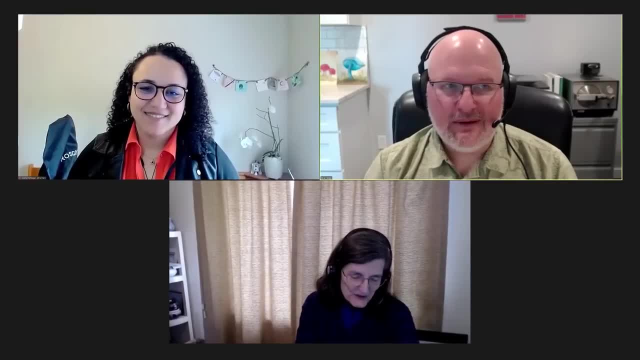 Oh, it really came down to. you know, dry environments, Right? Yeah, You know, and I look at it is. you know, nature has strategies for dry climates and it's all about protecting the amount of moisture that has been imparted to that system. And you know, like you, already mentioned, the aggregation of the soil is a huge thing. I mean, that's, if you want to extend the amount of moisture or hydrology available to the plants, you want to have highly aggregated soils that are going to be able to maintain and hold that moisture And then also don't have bare. 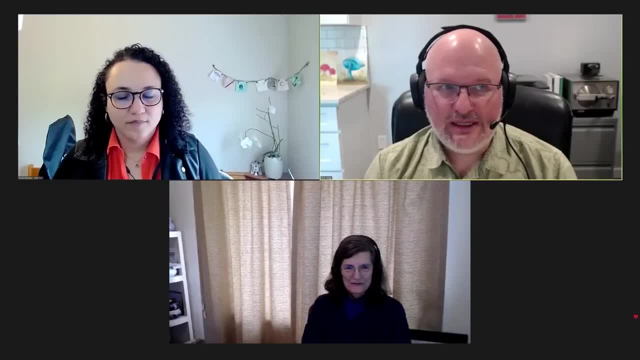 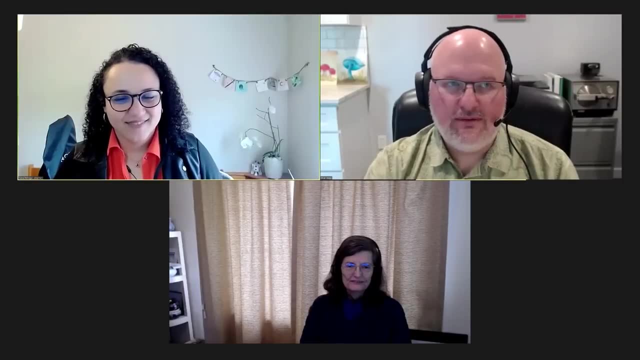 floors. You know, in farming it drives me crazy. I'll, you know, driving down in the Southern Valley of California, where it's a fair amount of moisture, And I'm like I'm going to have to look at that soil And it's very dry and everything is just completely denuded of everything but the 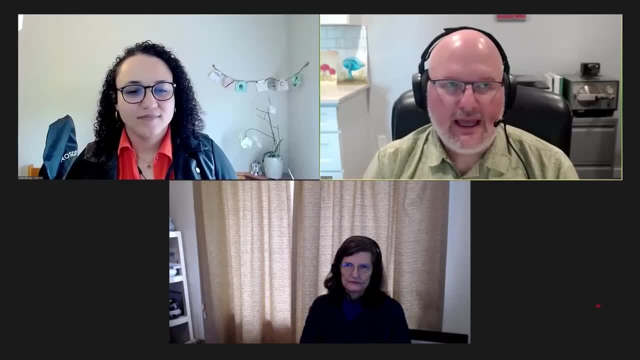 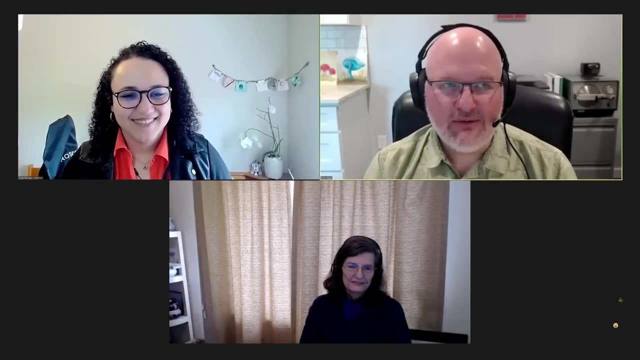 cash crop- Let's say it's almonds or whatever it's going to be- And we have water problems in California. I just look at that and go, wow, the amount of moisture that just evaporated out of that soil because we didn't put any kind of cover or protection on top of that soil. It's crazy. 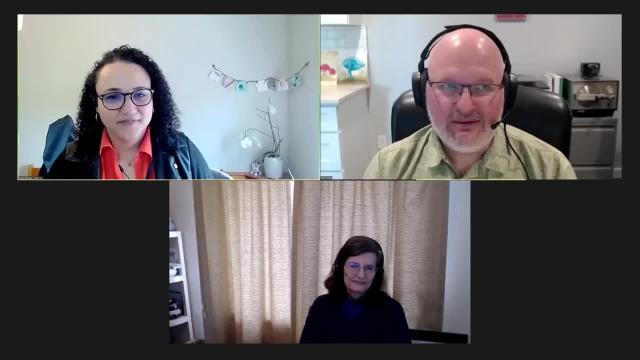 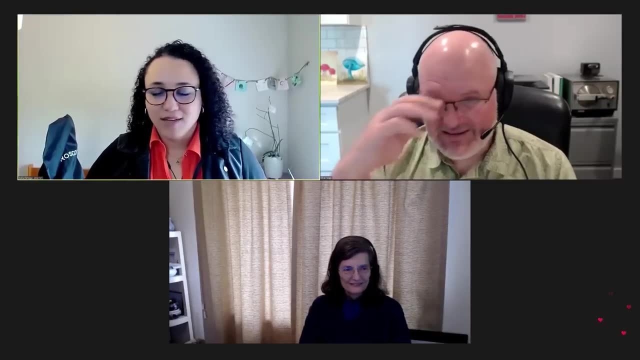 So I think as managers we got to look at both the doing, the mulching and whatever cover plants we can put in there, but then also get the biology that make aggregation. Sorry, Carla, go ahead. No, I'm sorry. It's about building up the soil structure again right And understanding that everything is. 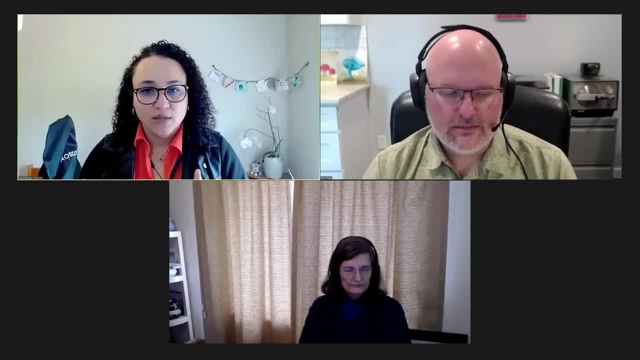 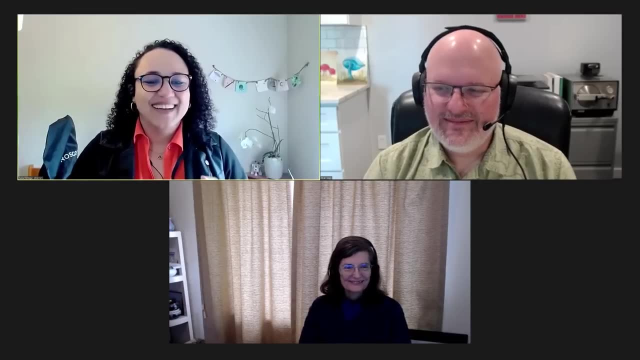 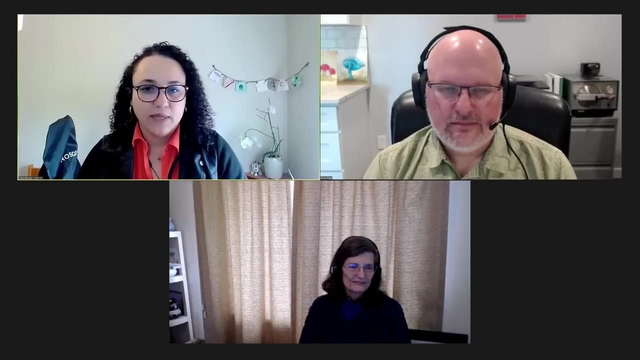 interconnected no matter the season of the year you are, So you have to have the best practice of management, like Adam's posting a lot of them in the chat- Thank you, Adam- And also thinking through the process of why I'm doing this, what I want to achieve with this step, And really sorry. 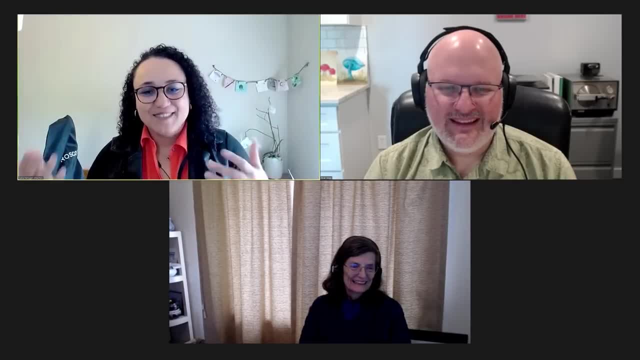 Dr Elaine, read what which message Modernator is telling you. Yeah, so the first thing is to have a very good soil. You can adapt and adjust as needed to promote a healthy soil, a structured soil, so the moisture naturally will be there And, like Brian said before, as long as you are using. 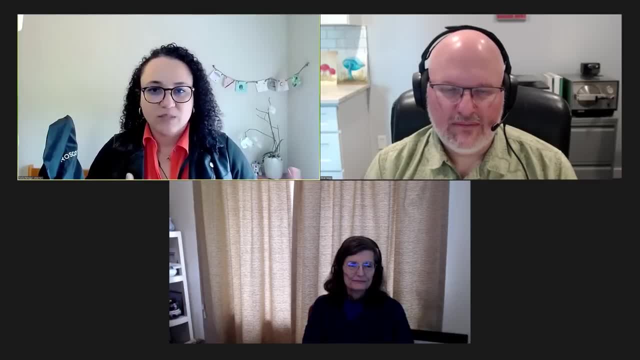 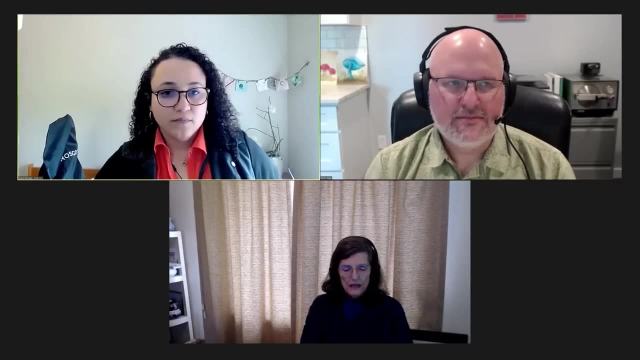 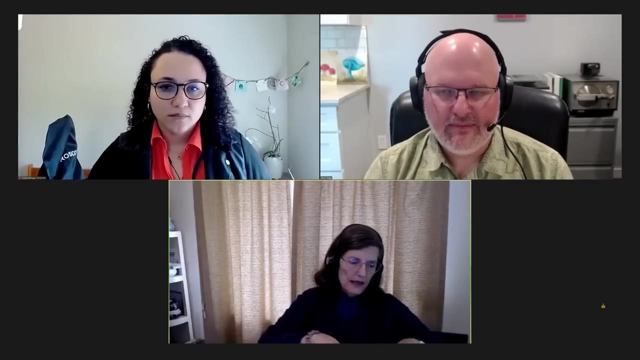 well-adapted biology. they will thrive because you're respecting their boundaries, their limits, You're promoting a successful space for all of them to thrive And we know that if we can be getting the organic matter down into the soil, so the microorganisms 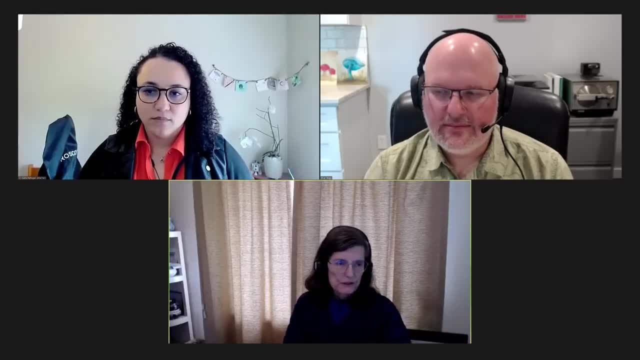 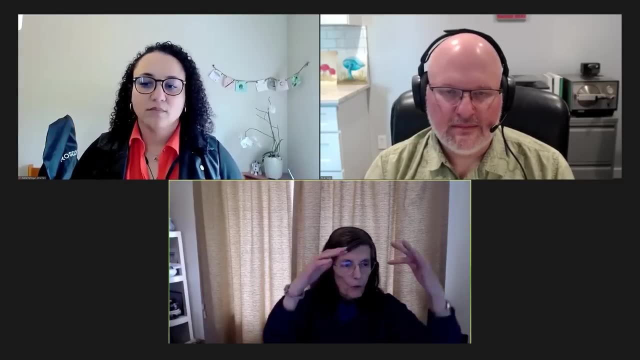 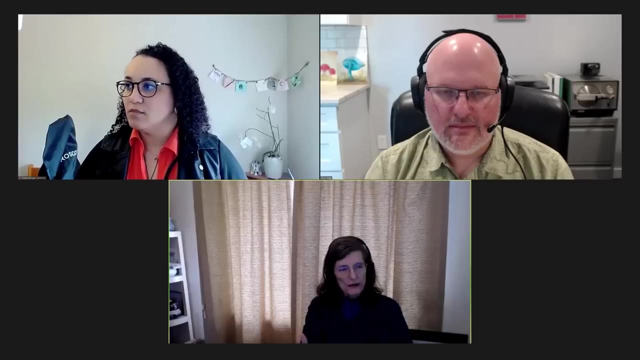 They go through the soil and build highways and passageways and hallways to move through, so that oxygen goes down deep into the soil, so that water goes down deep and can be held in those aggregates. So even though you're in a very dry climate, you still have adequate water stored away deep in the soil. How can you get your roots to grow down to that deep water and expend the energy sources? Well, it's going to go get the water it needs. If you had all of your water concentrated up here on the surface, that's going to evaporate very rapidly and you're left with no water. So we want to have these aggregates built way deep down into the soil. So if we're looking at Different kinds of trees and orchard systems or different vegetables, how far down do the root systems of your plants need to go to get to that stored water? 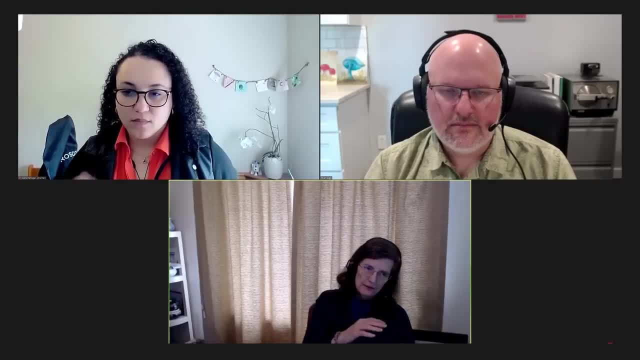 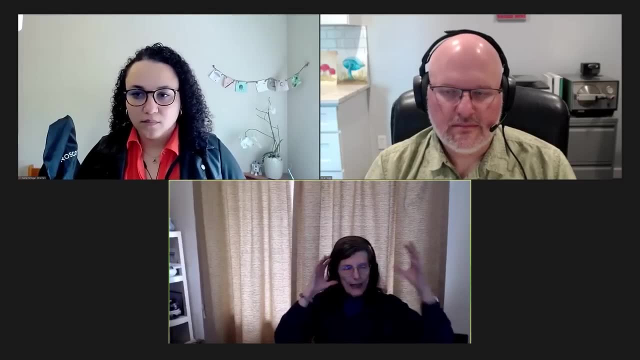 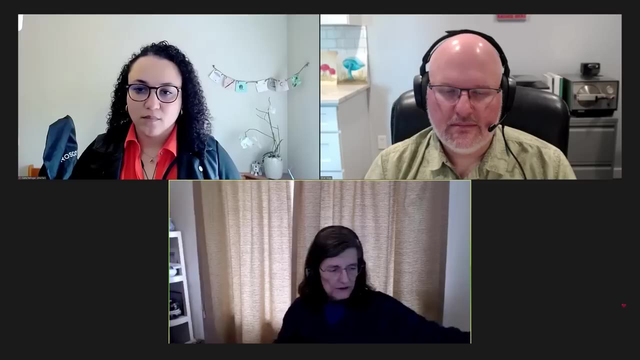 It has to be deep. It can't be three feet, It's got to be more like five feet, 10 feet, 20,, 30. So we have a really bad idea. The vision One was wrong, where, when human beings came in and they tilled the soil and they compressed the soil wherever they walked, wherever they had big machinery on that ground, they compacted the living daylights out of it. So the roots would only go that deep into the soil And then they have to go out sideways because, remember, if you compact you're going to be anaerobic. Oxygen's not moving in there. The organisms are growing in that compacted soil. Using all of the oxygen, And so now you've got anaerobic conditions. The roots of your plants cannot grow down into that anaerobic material, So it goes out sideways and fights with all its neighbors And it's not getting any extra water. You've got to water two times a day, at least once a day, And it's just a waste of water. It's just a huge waste of water. So we have to understand how nature has been doing this for the last. Well, the first rooted plants were observed on our planet a billion years ago. 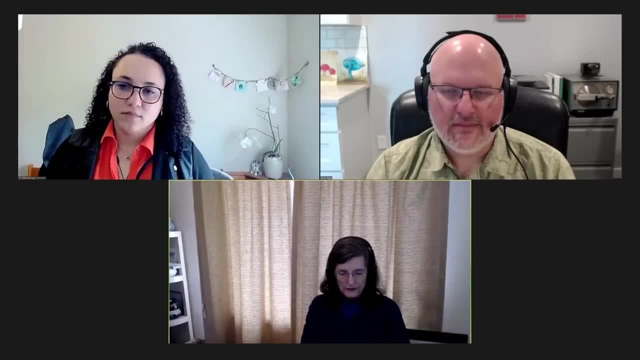 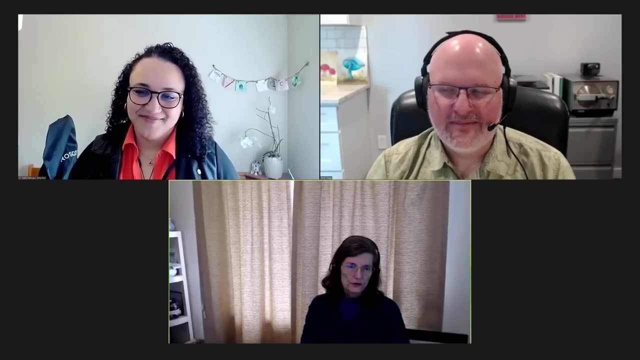 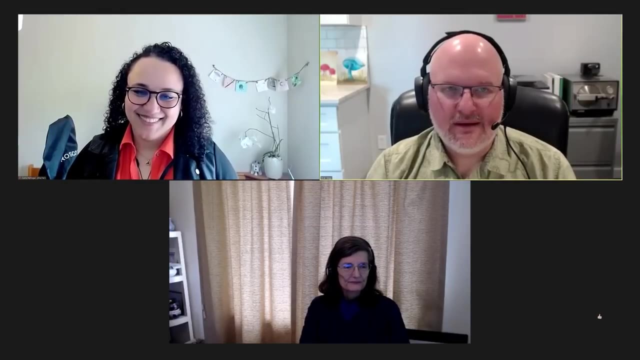 She's had a billion years to work on the system. Maybe we're very arrogant to think that we know better than Mother Nature. Yeah, exactly, Adam, anything you want to add. These two are rocking the casbah. All of you are rocking the casbah. 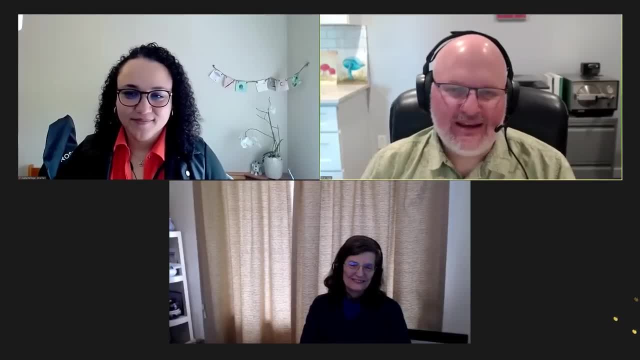 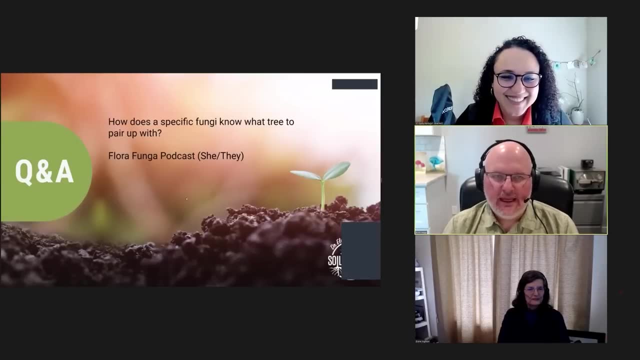 All right, let's move to the next question. Okay, next question. This question is from Flora Fungi Podcast And it is: how does a specific fungi know what tree to pair up with? How do these relationships occur? This one I can answer. 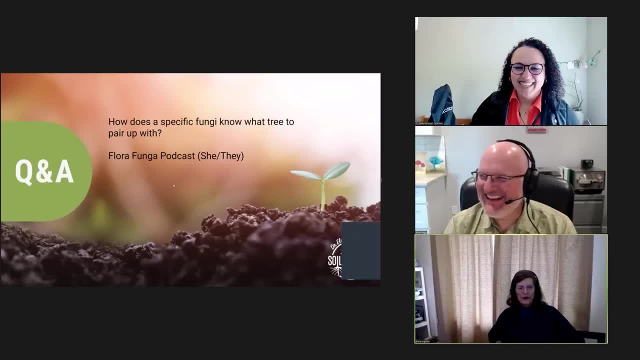 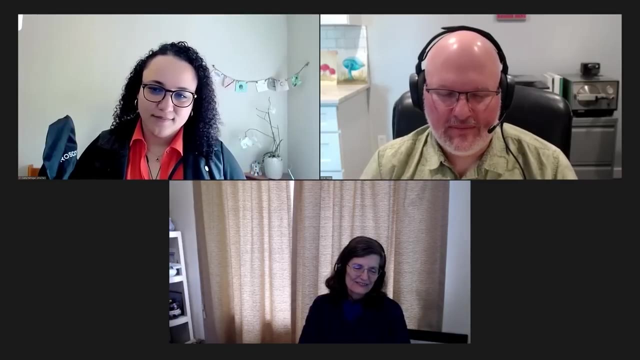 Go for it. Go for it, Adam. No, I've been grabbing the limelight. It's your turn now. Well, I mean, I talked a lot today, so I've been enjoying hearing y'all, So this is like a secret password. 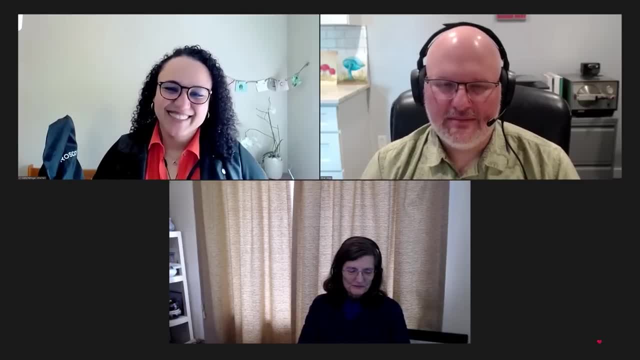 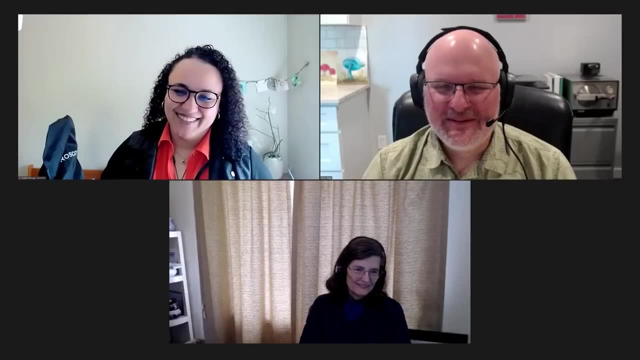 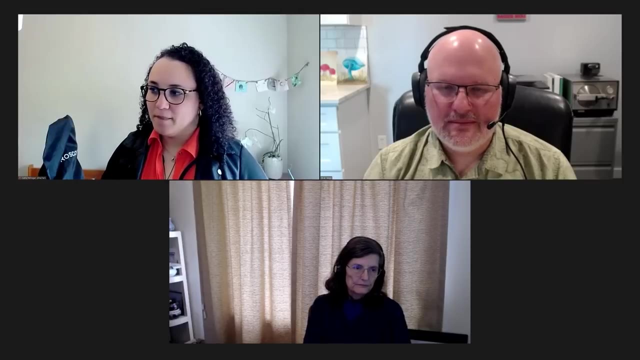 But instead of a verbal password, it's a chemical password. Biochemical, Yes, So the plant exudes some kind of hormones or other things. It depends on the plant, It depends on the fungi, But it's very complicated. We're talking about things that don't last long in the soil. but it's a chemical signal, a biochemical signal. 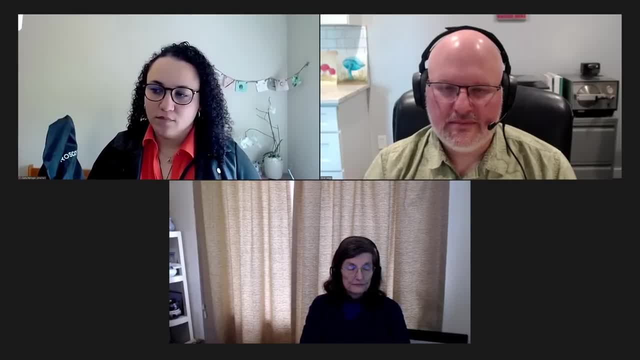 And the fungi go: oh, it's time to hatch. And I'll move towards where that signal is coming from and I'll get the nutrients I need Because, especially with arbuscular mycorrhizae, they can only get their food from a plant. 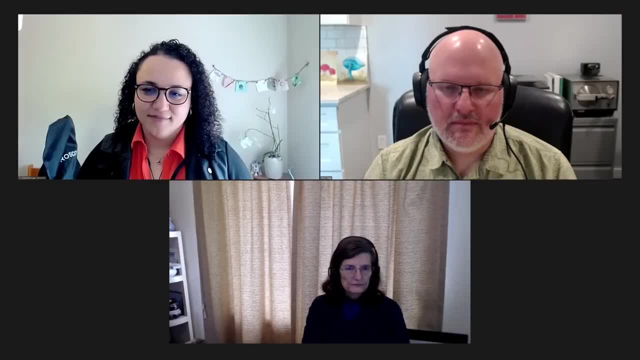 They have to form this symbiotic link. There's some fungi, like ectomycorrhizae, that can do what we call saprophytic lifestyle. They can feed off some organic matter. There's lots of saprophytic organisms fungi in the world. 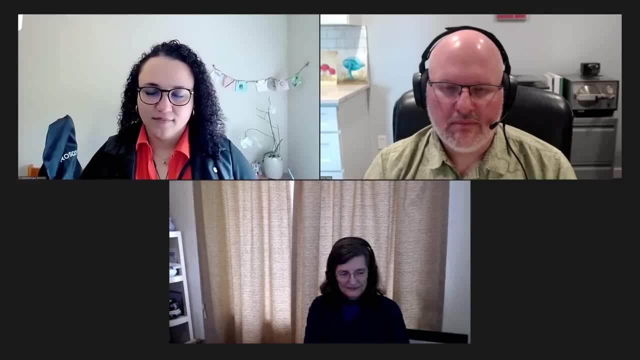 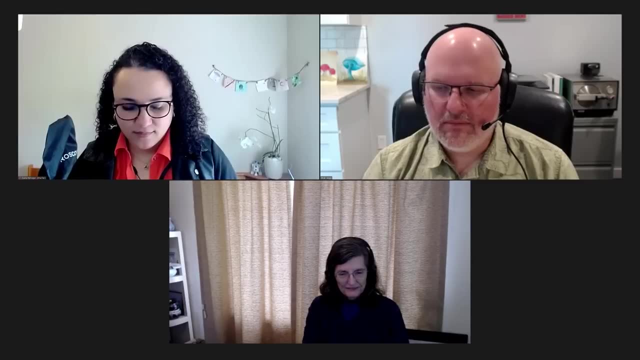 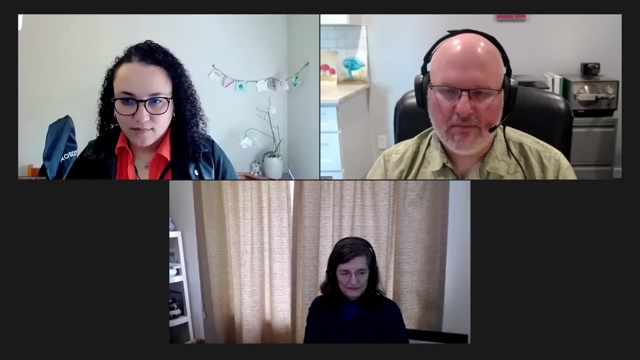 But in many cases, especially if there's this tight connection through time, through evolutionary time, then it's a lock and a key that's developed there, But we also. it's interesting to note that some other organisms, Organisms- have figured out how to hack that biology. And there is a devastating weed all across Africa. They call it the witchweed, Striga armonthica, And it's got teeny, tiny little seeds in the soil. And when the plants, especially corn or sorghum, start signaling to fungi that they need them, those little tiny weed seeds wake up and they stick their stinking roots into the roots of the vein plant. 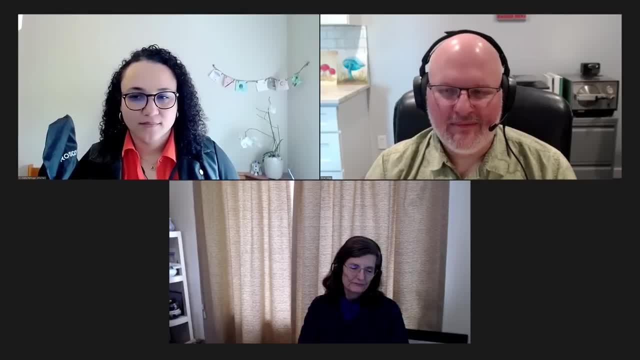 And they suck the life out of it so that it never produces a lot of food, And so that's the same system. It's the same mechanism. It's just reading the radio chatter and determining the cipher and jumping in there to do something nasty in that case. 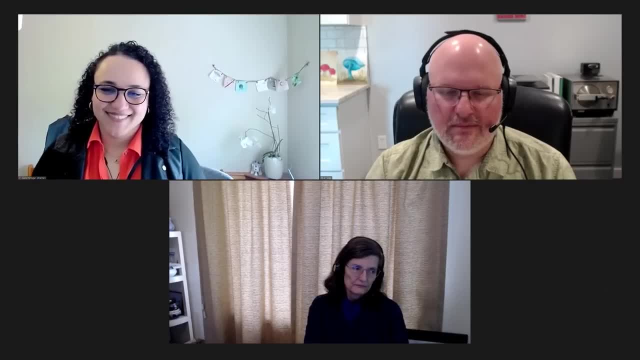 So, yeah, That's really how it works. It's pretty neat. Yeah, I need to go looking for some organism. That would be really cool, Really nice. Yeah, Thank you, It was a pleasure, Thank you, Thank you. 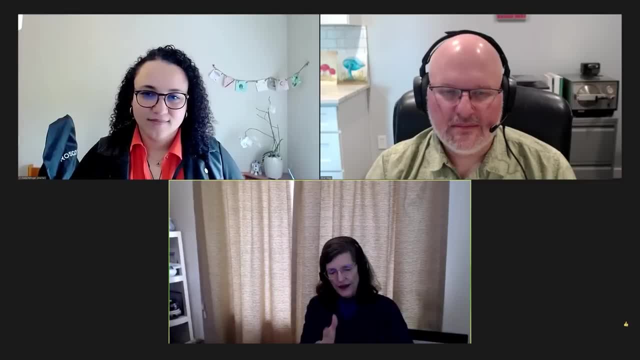 will adore the fact that that problem plant is present. And so you know, confrontation in the soil of this fungus with that fungus we've got to. we would need to find something like that, or it could be a bacterium, And you only seem to find these things. 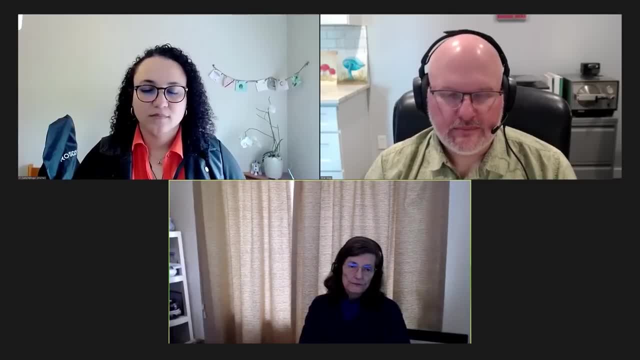 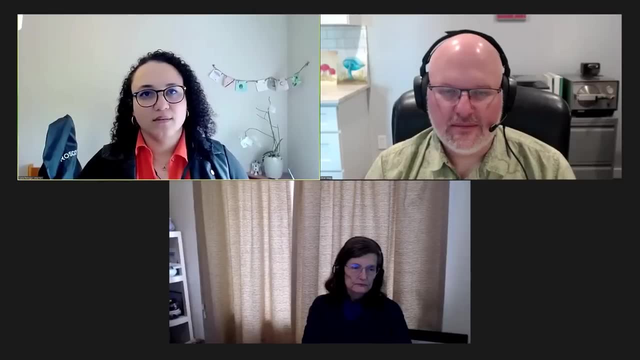 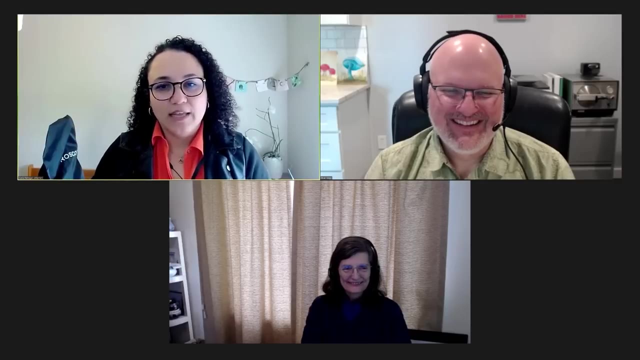 if you're working very carefully with your compost, Carly. anything else you want to add? Oh, it's just being a tiny bit nerd. Of course, I need to still learn a lot with Adam, But if you have a main question, 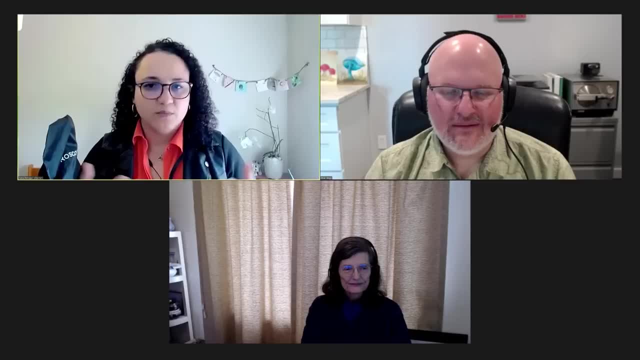 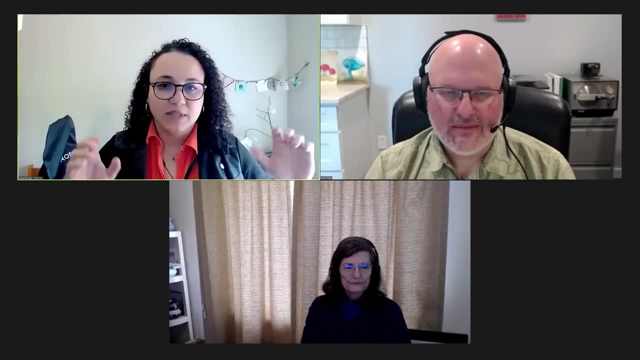 if you are not sure if your plant has one specific mycorrhizal species or everything, there is always one amazing source to go, which we recommend: Google Scholar. Just type the name of the plant in Mycorrhizal Association and probably going to find out a lot of tons of information. 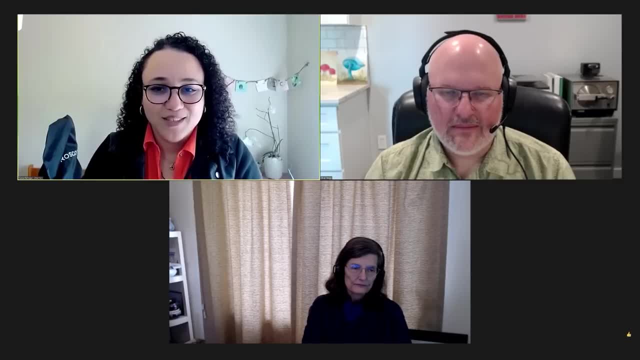 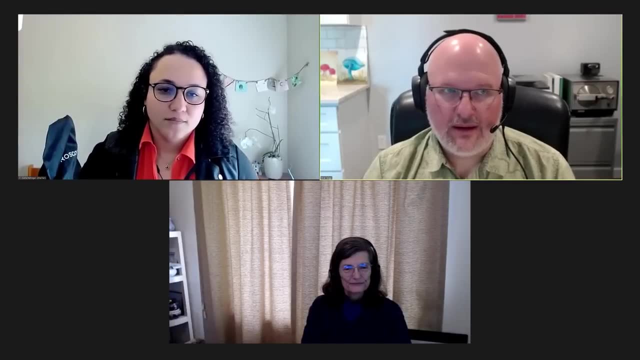 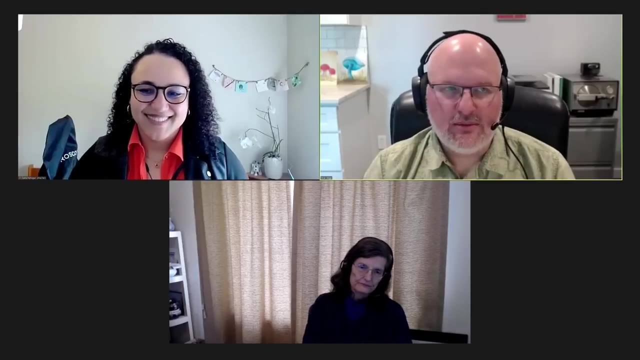 And also you can always reach out to the school for more support if you need it. You know this is interesting because it does broach a question that I get a lot working with my clients, which is what species of fungi or bacteria or you know, name your organism. 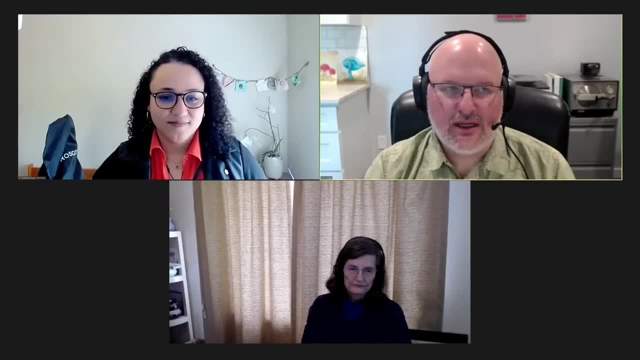 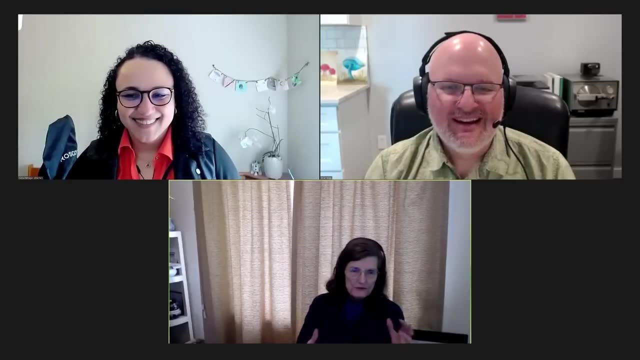 do I need to have for my particular cash crop, And is it present or not? And that's a difficult question to answer sometimes. And you need about a thousand different species, Right, exactly, You know a bunch of them, Right. 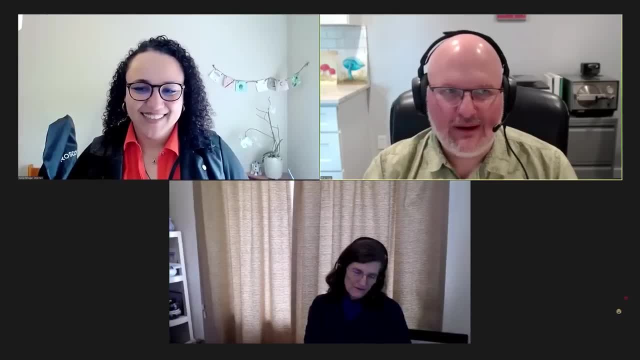 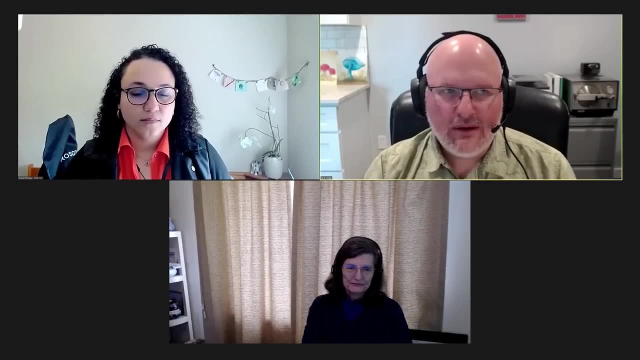 And they're so used to the more that reductionist. well, I only deal with these four fertilizers, so there's got to be four fungi that are going to be what's the ones I need to have in my soil. And this is where you know practically we look at saying: 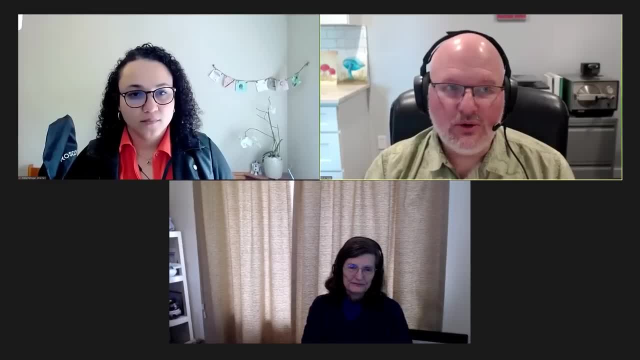 well, we want to create compost that is the most diverse that it possibly can be. Not knowing that I have, you know, species X, Y or Z that I can use. I'm trying to make a compost. that's going to be. 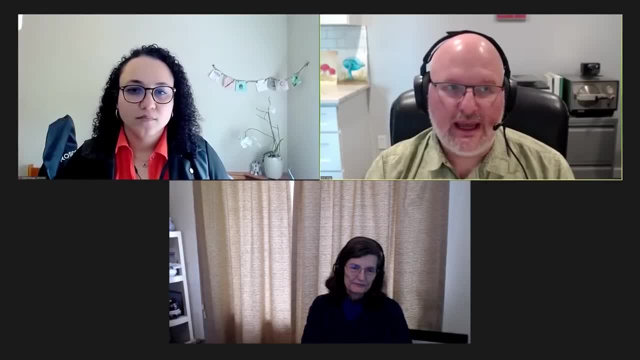 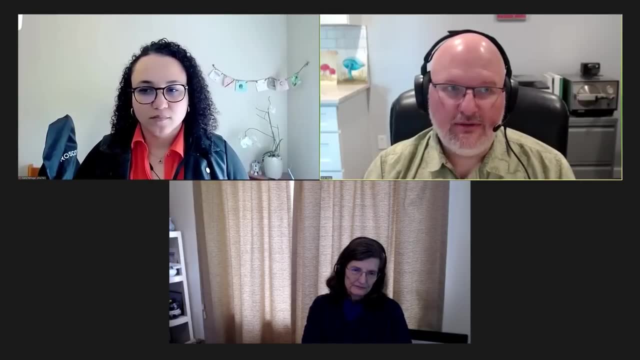 that is going to be really related to that particular plant. I'm trying to make a compost that's going to really have enough diversity to try to fulfill whatever niches that that plant needs. Now you know, there is the- you know- evolution of DNA analysis. 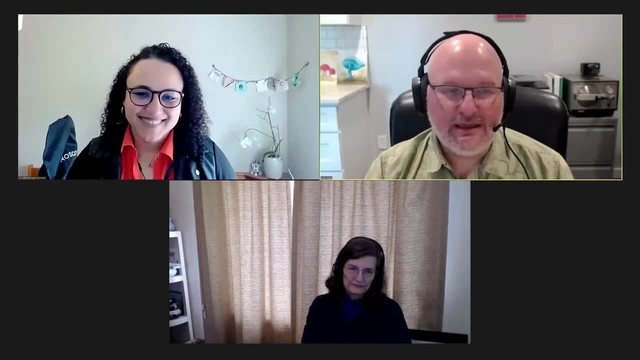 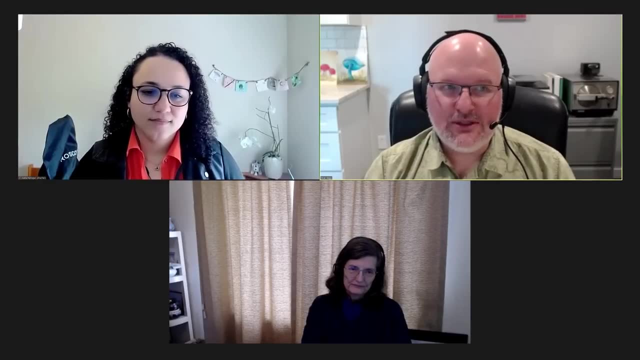 that's coming out and I'm sure we can probably become more specific with this. but you know, creating a compost that has specific types of fungi in them can be really challenging, especially a lot of these fungi aren't don't do well lab grown. It's not like I'm going to make beetroot dishes, so these fungi add them into my- you know- compost. So I think that's the key thing for us right now, practically is diversity, diversity, diversity. Make sure we've got as many of those bases as we possibly have covered. And again, try to find those indigenous microorganisms that are going to fit for your bioregion. Really, really important, Because on the long run it becomes like a cycle right, You're going to treat your area with good compost. 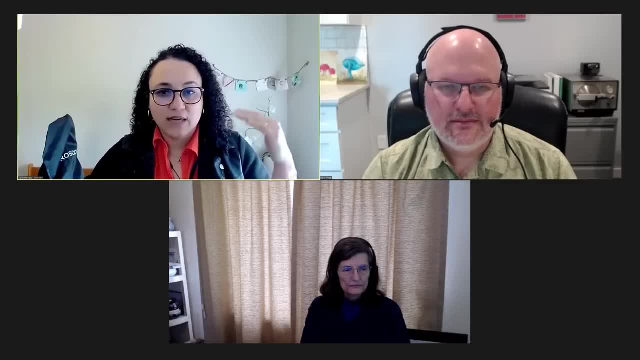 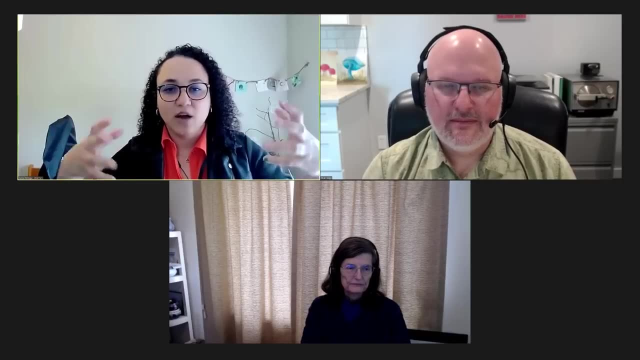 good extracts and good teas and all that material that you are not selling as your main resource. You can just put that in a new pile of compost. So you're tailoring all the biology for your specific area and your plant, because the plant association. 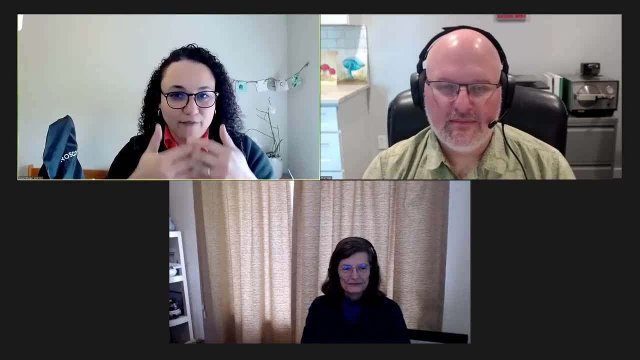 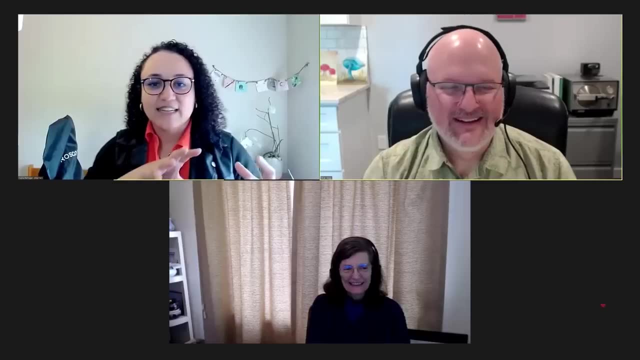 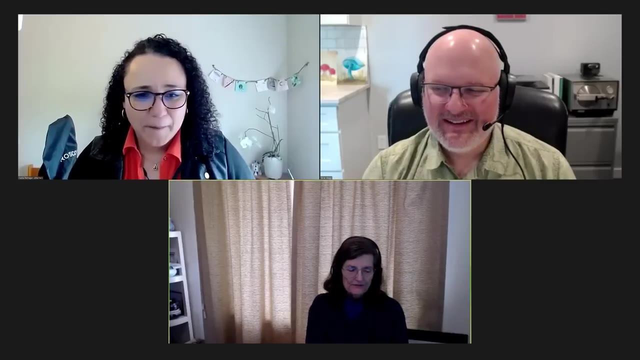 the root system and the biology will develop these partnerships, symbiosis- many names that you can put here- and then the system retroactive feed itself. So sorry, Elena, I interrupted you. Well, there is one more thing that we you know. 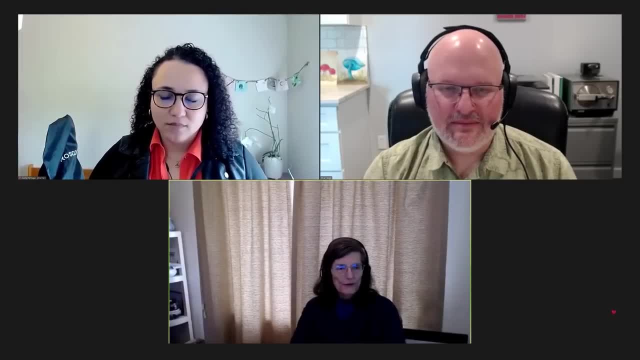 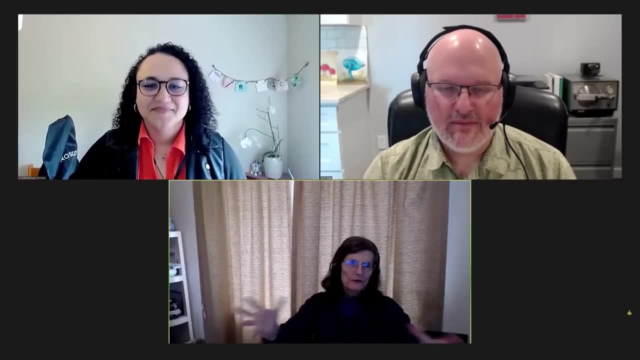 really need to consider, and that's the weather. It's not always going to be the same all the way through the growing season. I like to, you know, always put the question out to my students. you know, when is the last time that you've seen? spring or summer or fall, exactly like this one. And their answer is never. It's never been the same. But when we've got these, which species of bacteria, fungi, protozoa, nematodes, microarthropods, earthworms? and all of that, which ones should be in your soil? We just want to maximize diversity, because you're much more likely then to have the thousand different species of bacteria or fungi, et cetera, et cetera. We're much more likely to have things that will combat. 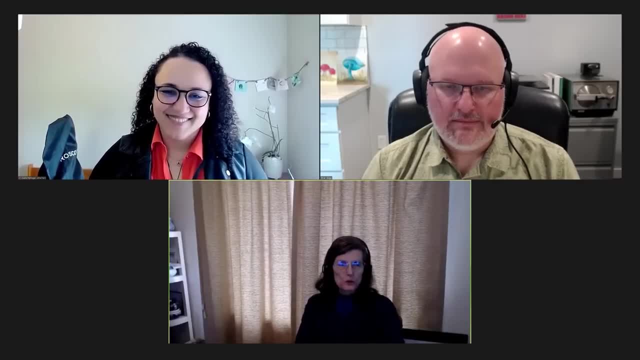 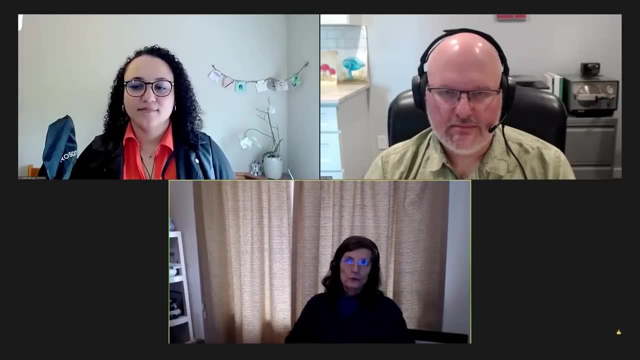 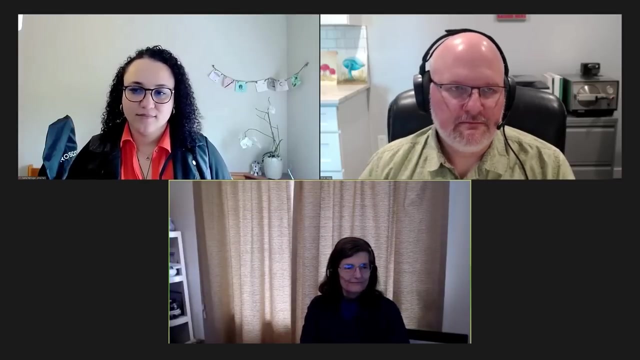 all the problems, that will improve the storage of water. that will, you know, make certain that your plant gets all the nutrients that it needs through whatever mechanism, where you want to be- And probably we want all of the mechanisms operating, so your plant is never limited for any nutrients. 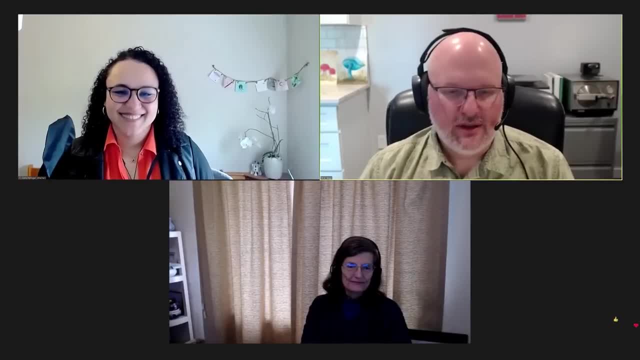 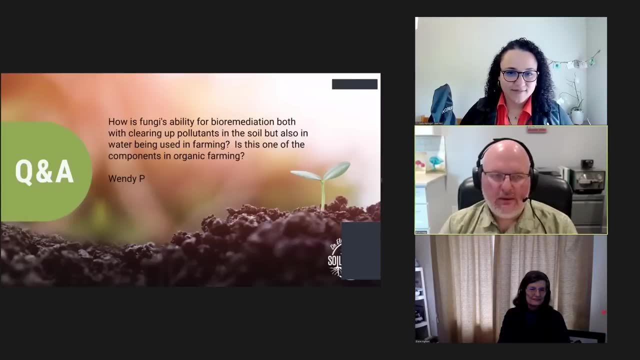 Okay, I think we did justice to that question for sure. Let's move on to our next question, And this question is from Wendy. And Wendy asks: how is fungi's ability for bioremediation, both with clearing up pollutants in the soil but also in the water being used in farming? 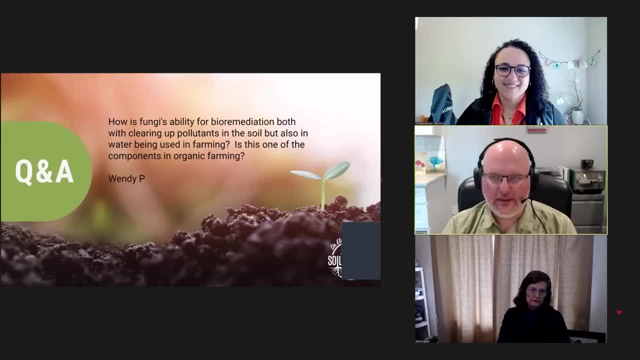 Is this one of the components in organic farming? Yeah, Fungi are really terrestrial systems. I think it was like somebody else had a question about you know, what do fungi do to help things in marine or aquatic systems? Well, the fungi don't really hang out in the water. 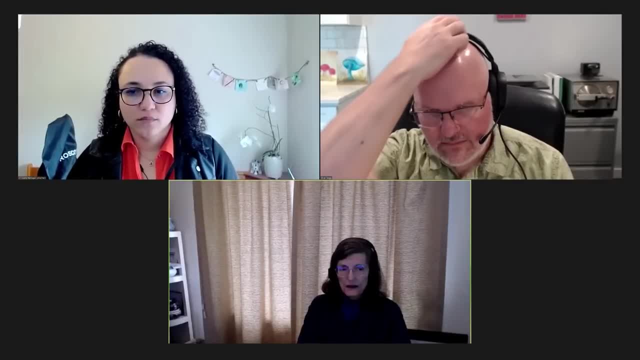 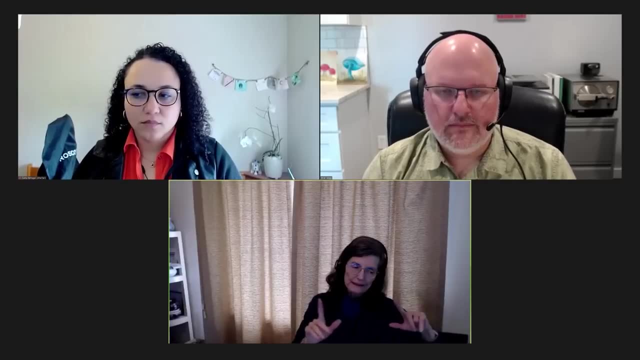 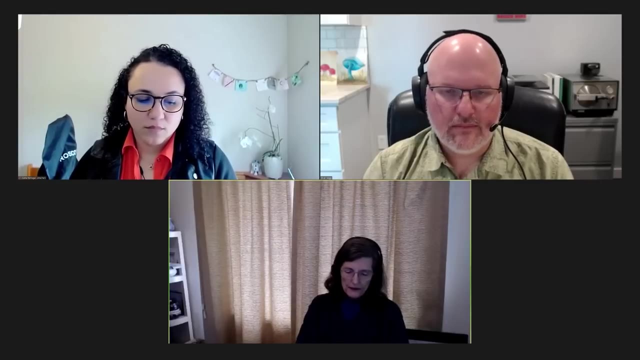 They hang out in the sediments. So sometimes you can find a pretty decent layer of fungi growing in the sediment, but it has to stay aerobic. That's a real limitation for the fungi. We do know that. you know, if we make a compost pile where we have. all of this diversity of different species of fungi, bacteria, protozoa, nematodes that we most likely have, all of those organisms that are needed to decompose whatever toxic material that might be in your water. pass your water through the compost pile so that you make certain. you deal with all of the toxic chemicals. You probably want to check and make sure that you know you're actually dealing with all of those problem chemicals. once it comes through the compost, Maybe you need to give it a longer shelf life. It takes longer to deal with the problem than you had. than just what a simple run through the compost would allow. So how long You've got to do some testing? How long Maybe it's just increasing the amount of fungal biomass so you get the effect faster? All kinds of questions. We don't know everything yet. 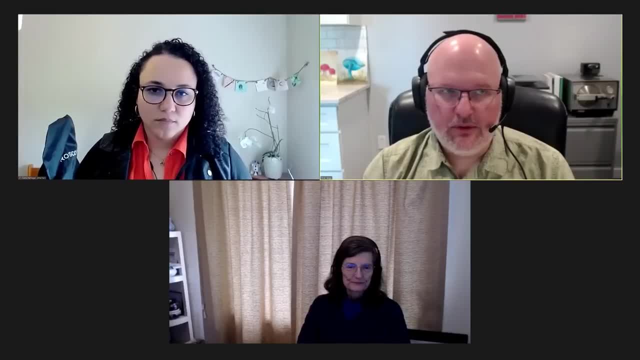 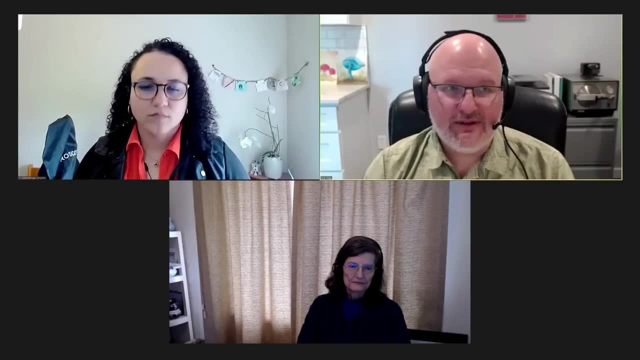 Right, You know, I think there are some people who are doing fantastic work, especially with bio-remediation. You know Paul Stamets. you know his work with fungi And developing fungi that are very specific towards certain toxic issues. 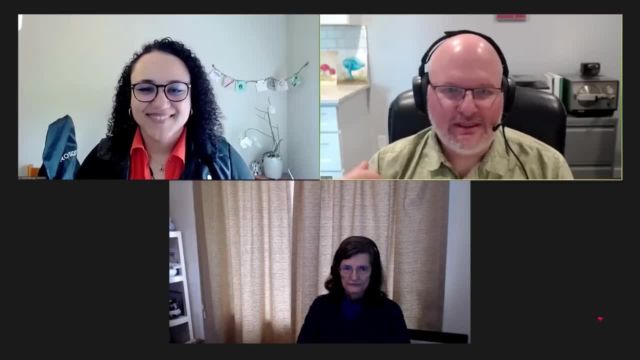 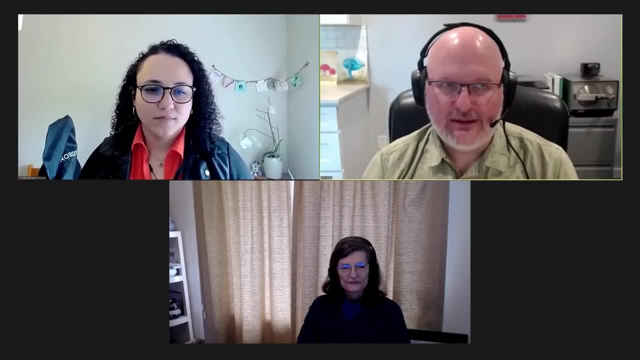 You know, I think he did a lot of research on like diesel fuel and was able to use, you know, fungi to absorb and to collect that material. I think it's fascinating. I think there's, like you said, there's going to be a lot more, you know. 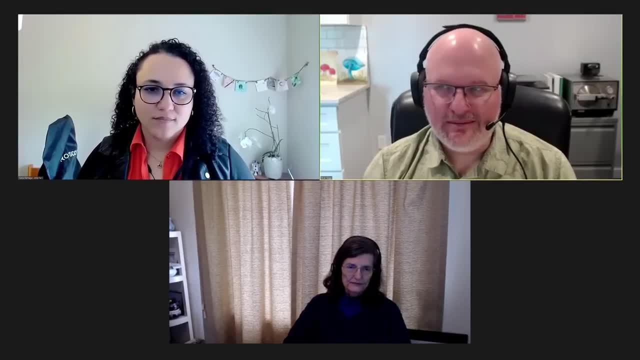 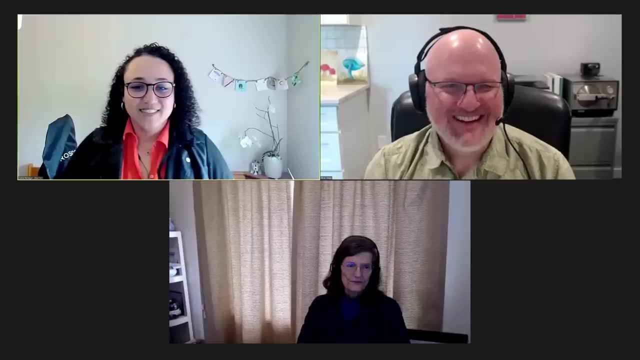 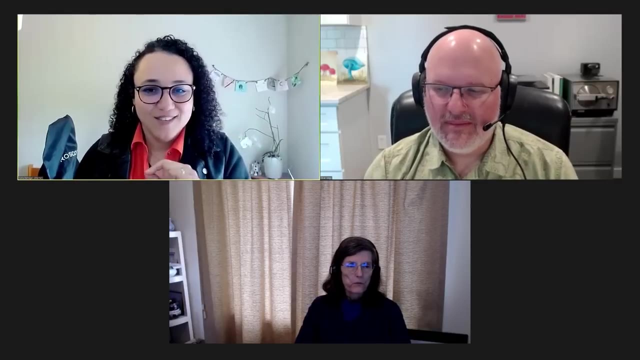 science going on in this space, In this space in particular, Because we have a lot of toxicity that we've got to clean up. You know we've made a mess of this. Like Adam said earlier, we are just touching base on how much we know about species. 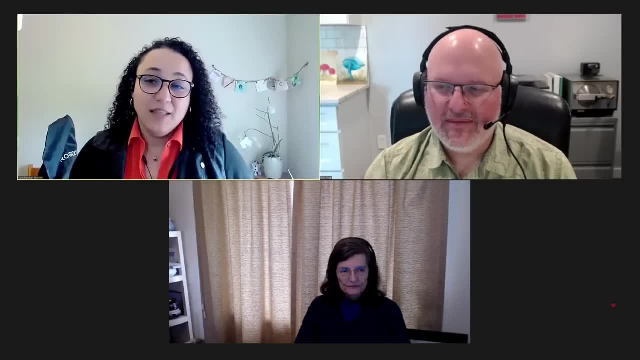 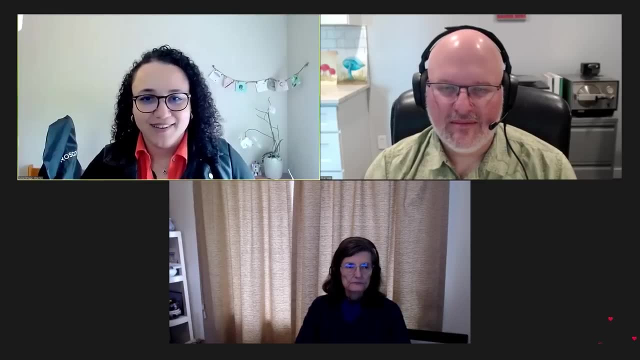 So how much more secrets are there for us to find out? So it's my opinion, It's just the beginning right. The solution is there, We just didn't find it yet. Yep, There are ways to take a thousand different species. 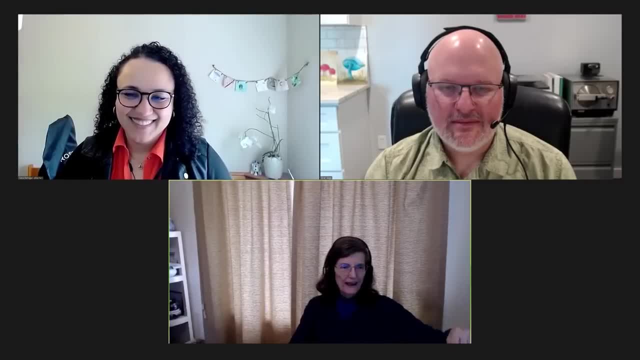 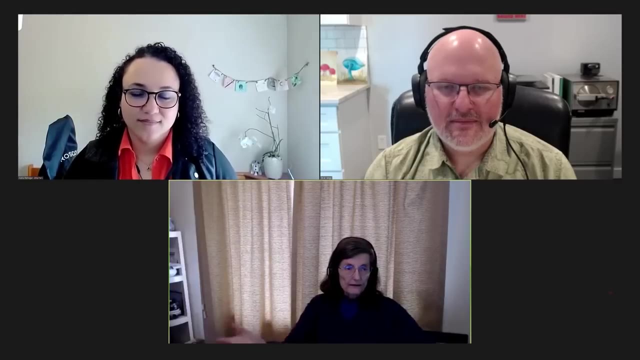 And instantaneously determine: does it have the ability to break down this bond or not? These guys break down this other part of the problem And this one breaks down this other part, And that's going to be really nice when we've got it. 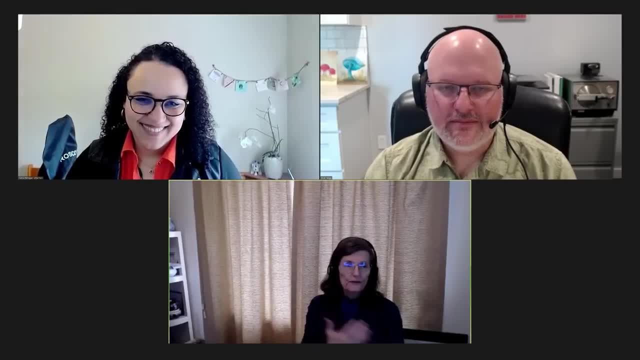 But we don't have it yet. So we're very practically oriented. These are the simple ways to deal with it. So we're going to have to pick up the machine And then we're going to have to deal with the. You know. 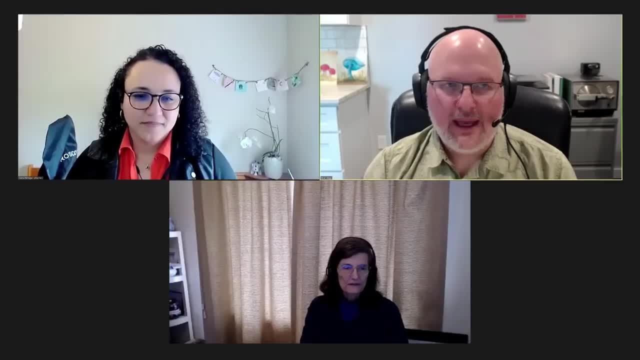 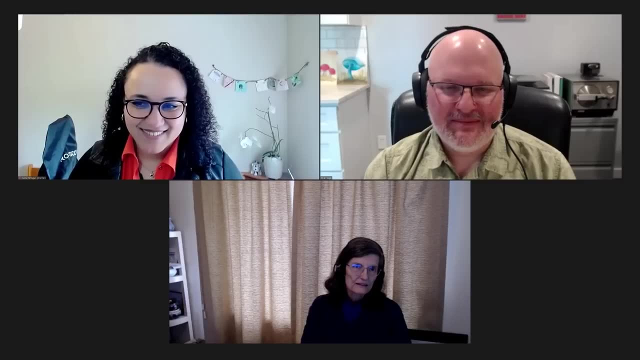 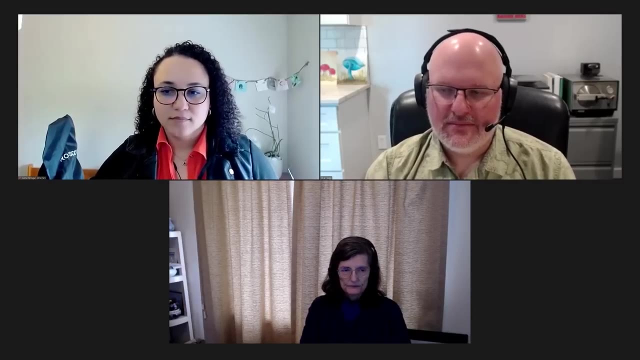 We're going to have to deal with the contamination or you know, disease or contaminated materials, Go ahead, There you go. Remember that Things that like commercial cultivation of mushrooms or things that have been like lab rats for a long time, It's like saying, Oh, I heard that wolves are good for ecosystem. right. They're just going to get eaten. They're just going to die. They're just going to cause more problems. potentially right. If anybody's been to the deep South of the US and seen kudzu, I don't want to see the below ground microorganism version of kudzu. that's an invasive species. 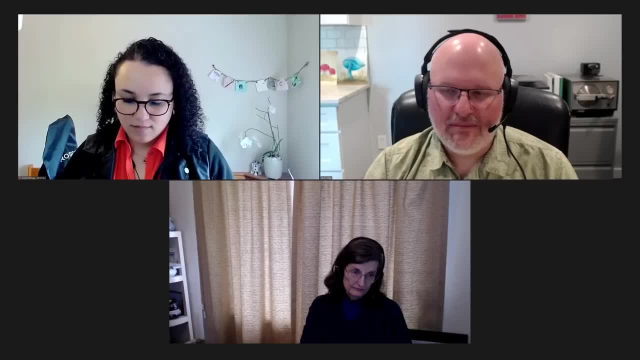 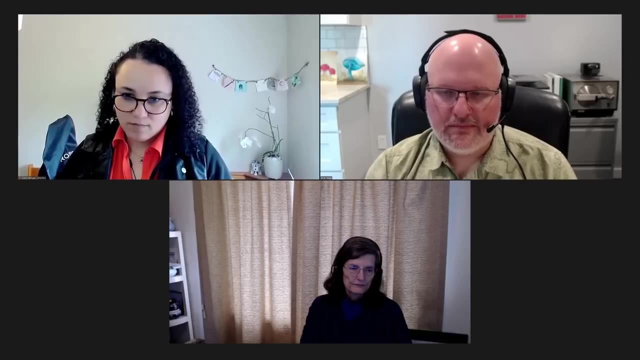 right, So we have to be. this is why we always default to diversity and local diversity with these microorganisms. And you know, Elaine has said it so well- that we create this sweet spot, this Goldilocks condition in our composting process And then we just get. 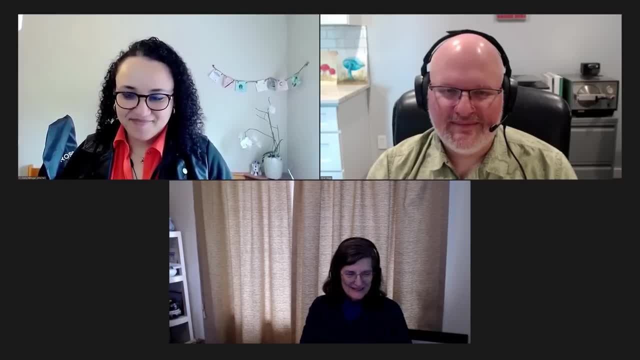 bajillions- that's the science term- bajillions of microorganisms in there, of all different kinds, And somebody asked if they'll compete. There is competition and that's also valuable, but there's more and more. you know science and technology that's going to be able to do that And I think that's going to be. 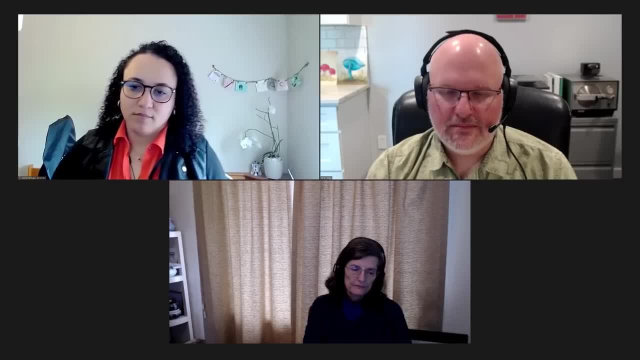 more and more. you know science and technology that's going to be able to do that And I think that's going to be more and more. you know scientific verification of things like quorum sensing, where, over time, these communities fill, they switch food sources or they switch some other. 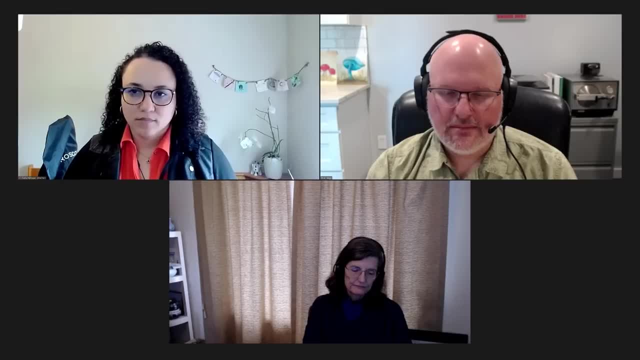 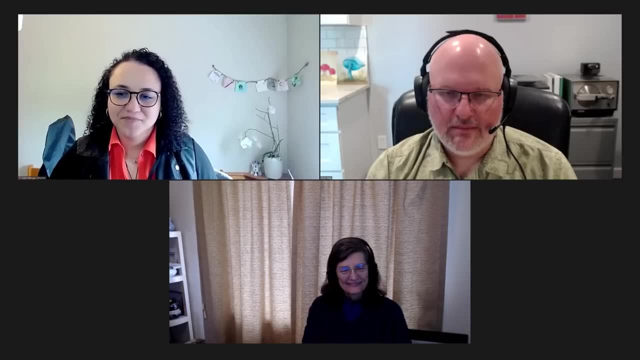 part of their behavior so that they can collaborate more. You know, this is like if you put together a brand new symphony, a brand new group of musicians, it might take them a while to learn how to play really beautifully together and to learn how to follow that conductor. 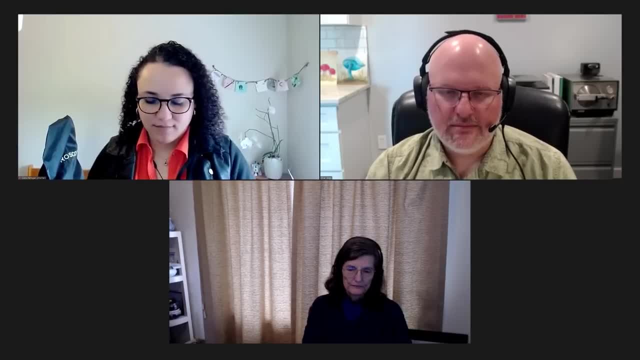 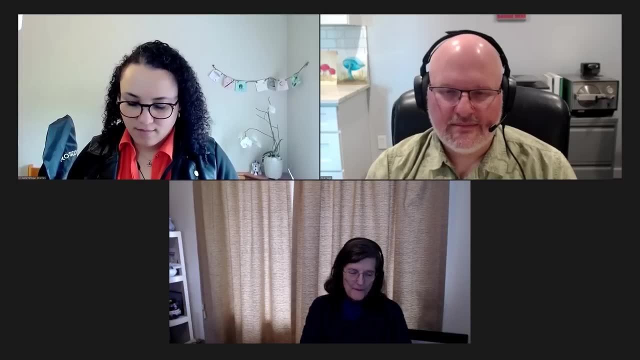 you know properly. so, going back to that metaphor, you know it's how many different instruments are in a beautiful orchestra. that's diversity. we want that that harmony in the soil comes from all the microorganisms contributing their unique functions and roles and, in many cases, doing. 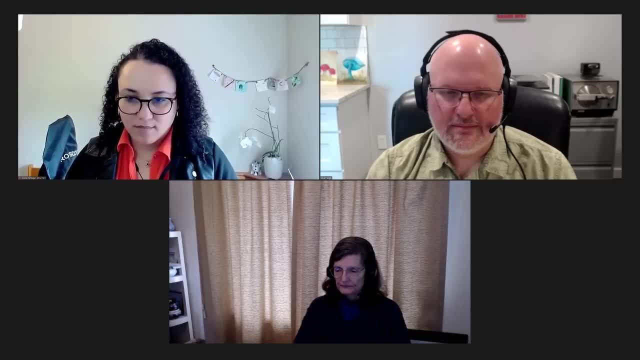 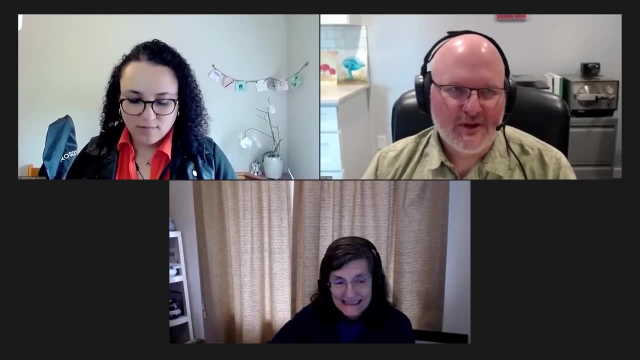 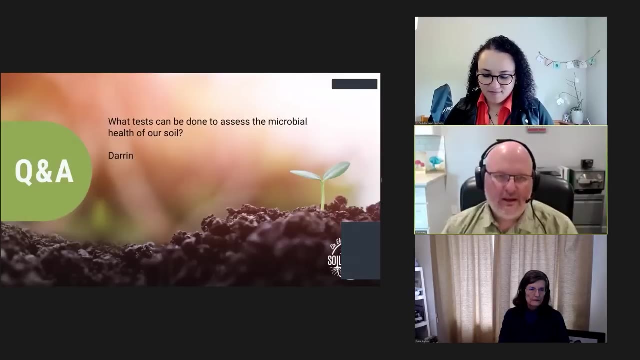 what they want to do, what they, what, what they, what's best for them, and then it all becomes this beautiful symphony. well said, all right. let's move to another question. um- and this question is from darren and darren's- asked what tests can be done to assess the microbial health of our soil. 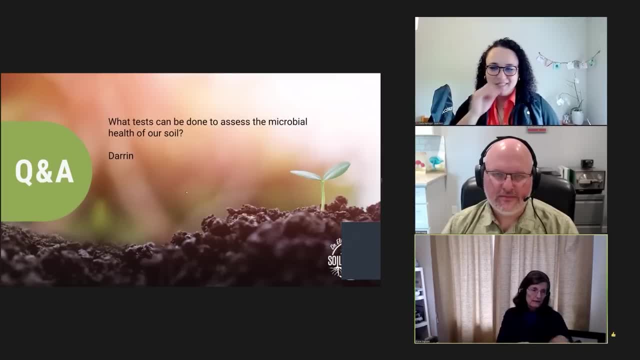 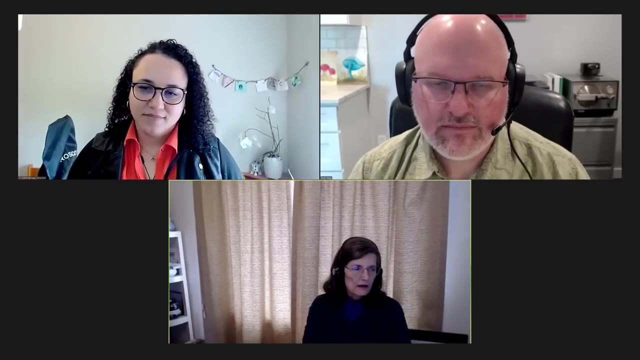 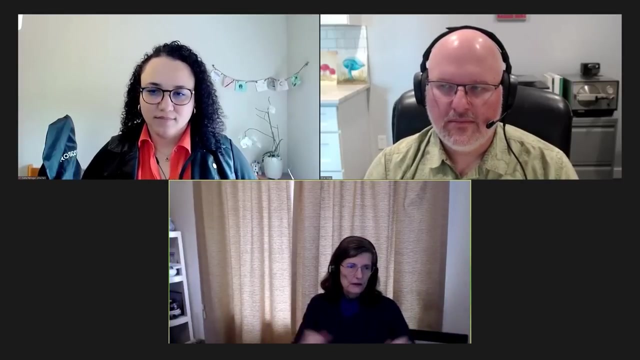 probably the easiest thing to do is to like: have a control. where you're going to not add anything to that soil, then you know, add to the next unit, um, put in, uh, add it, and make an addition of really good compost and then compare the growth of the two plants, measure the sap, do bricks, do you know? there's a huge. 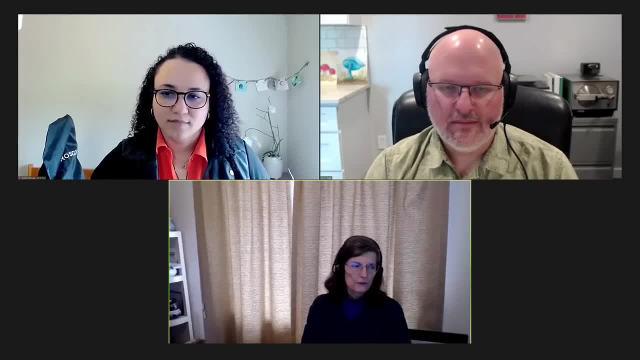 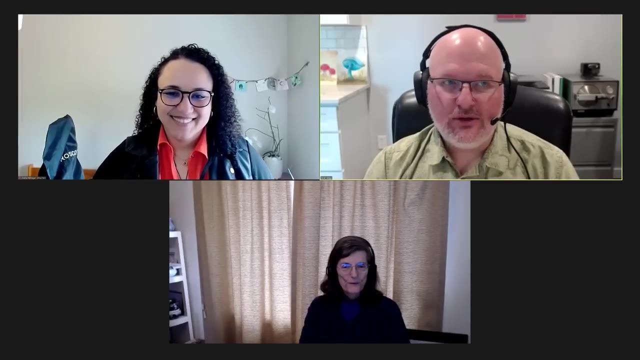 number of tests that people do to make certain that your plant is growing very, very well. the assumption is that if you've got a healthy plant, you got healthy soil, so that's one approach. you know, i'd love this question, um, because you know you get down to: is there one tool that rules? 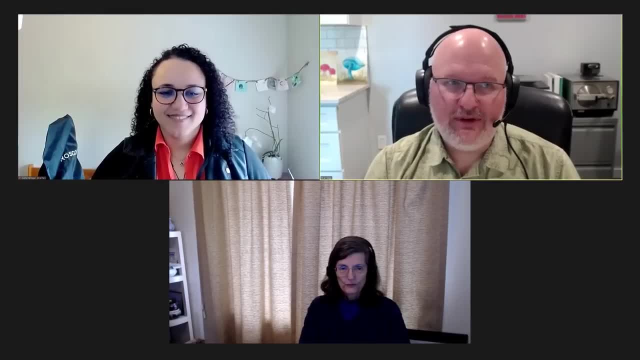 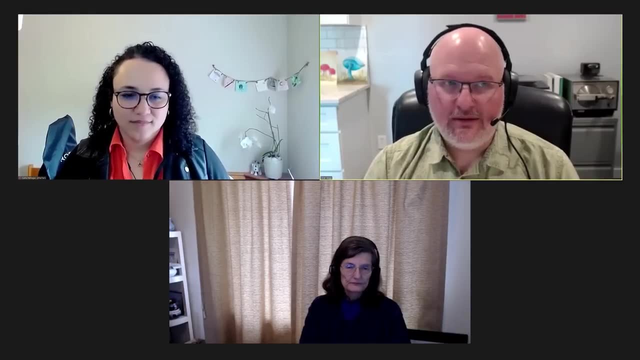 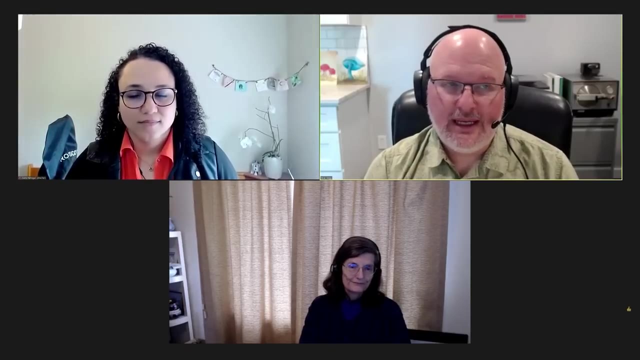 them all and i look at. no, there are some tools that provide you better insight than others, but i like to have a full, well-rounded set of different tools. you know, some people say, well, you know soil chemistry analysis. well, i can get some information from the soil chemistry test. i can also get it from a dna analysis, plus the microbial assessments that. 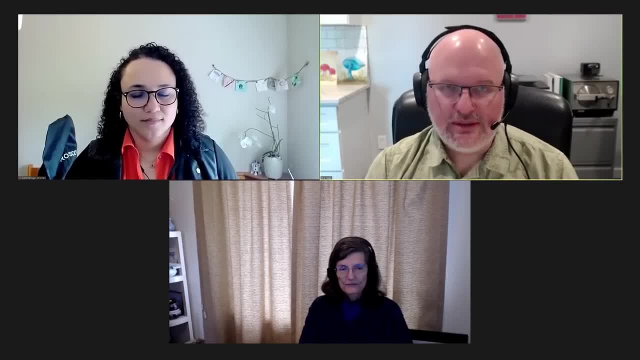 we do, you know. so it's the combination of all these different data points that come in that the help build a better or bigger picture. um, so i'm always an advocate for more. tests are better, but there's also a budgetary concern that my clients have to say: whoa, hold on a second, you can choose. 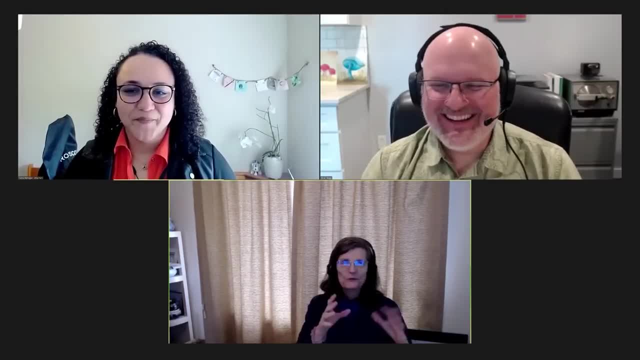 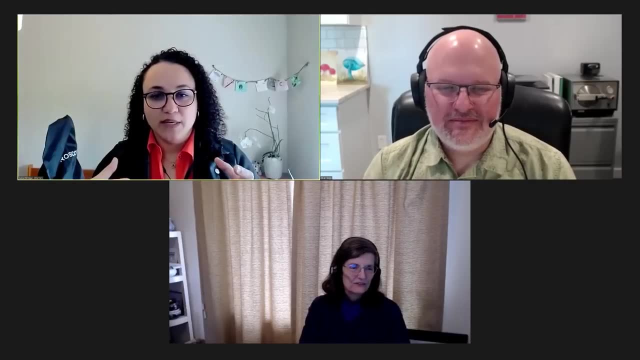 which one you want. all right, which you're going to tell you the most exactly? yeah, it's always about the question, right? you need to find that balance. what do you want to know on this moment? how, what's your budget and the timeline that you need? then you can tailor and and define the tests that 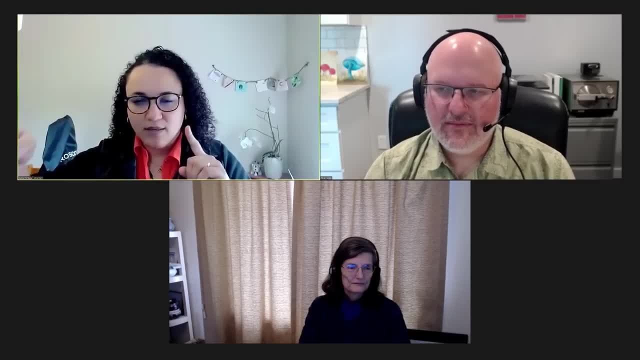 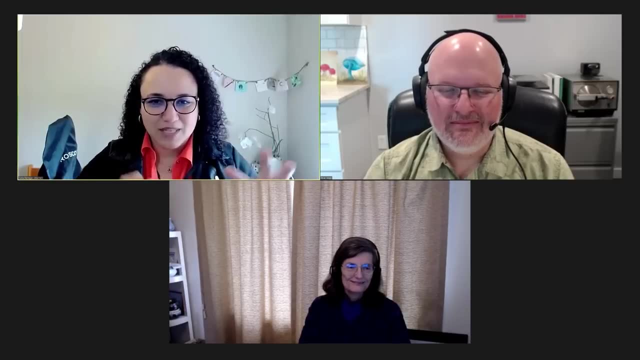 you're going to do, But, above all, always read the field which message is bringing back And, like Brian said- and I call it the toolbox- just keep expanding your toolbox, because more options you have, better results, not better results, sorry. better answers you're going to have and you're going to optimize your management. 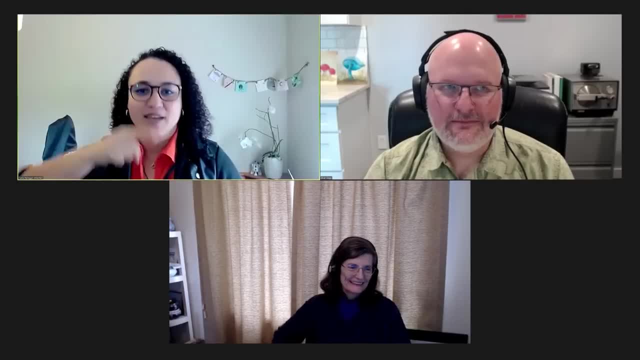 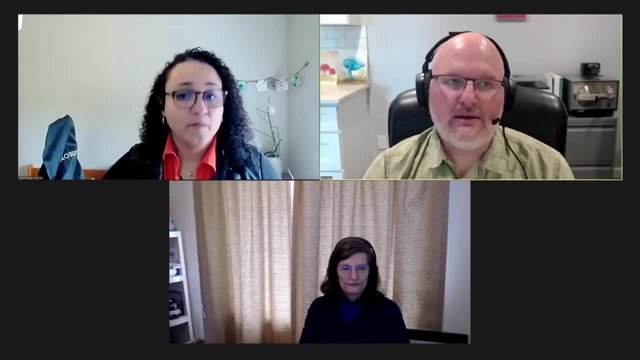 So then you'll go back to the cycle right, getting better every single time? Yeah, and having more tools in our toolbox is great, because then you can pick and choose which tools fit the narrative that I'm trying to really understand, And having more options is not a bad thing. 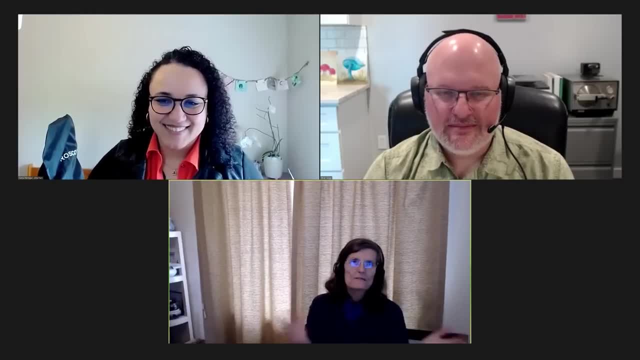 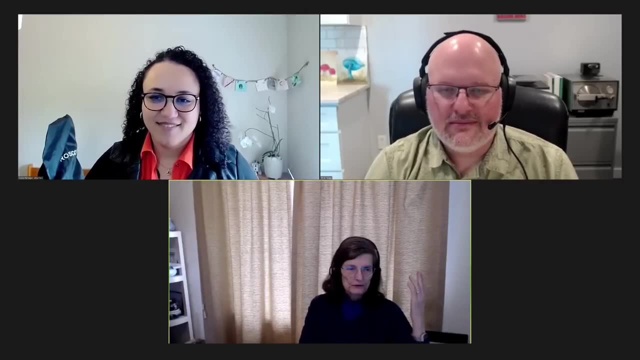 Yeah, there's probably there's one. you know, it's like a favorite thing that people in microbiology use- which is to measure the amount of CO2 that's coming from soil that's being incubated or something that's being incubated. 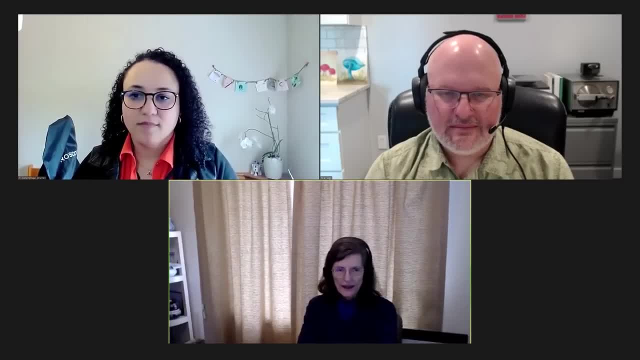 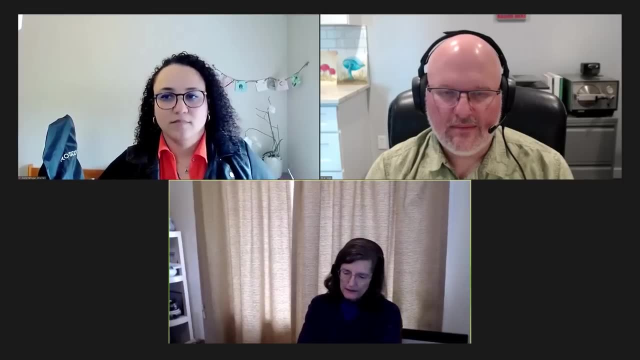 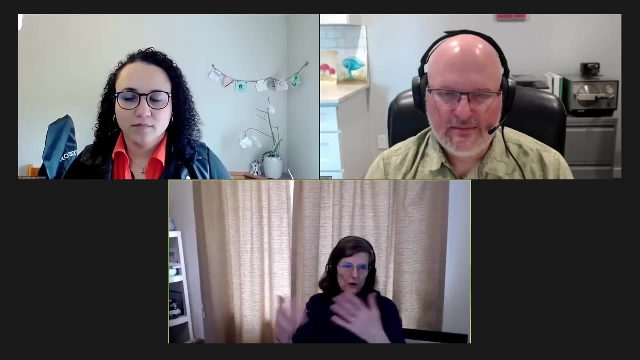 And Yeah, Yeah, Yeah, Especially when you know how important fungi and bacteria are. you need to know how much bacteria and how much fungi do you have. You can't glop them together. What does it mean if you've got 100 CO2 coming off of your soil? 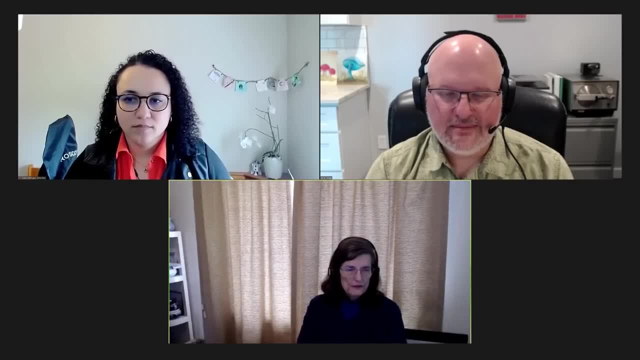 Who did the most work? Was it the bacteria? Was it the fungus? Was it the protozoa? Was it the nematodes? You know you can't. You can't split things out and indicate to your client what they should do next other than well, you should get more microorganisms going in there. 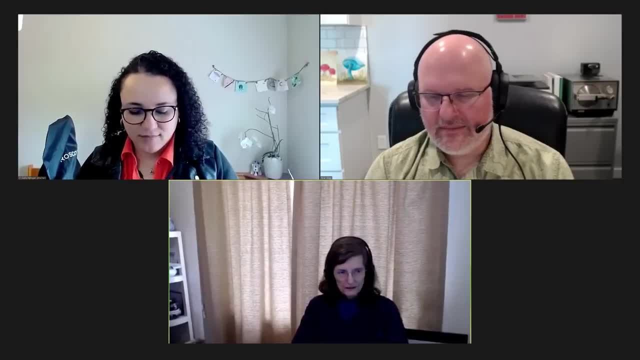 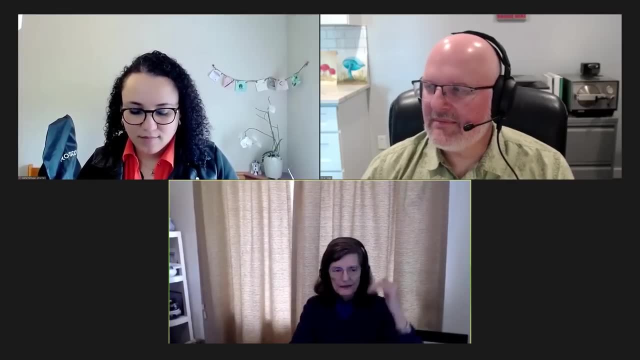 Well, okay, what's the inoculum? Well, you're going to have to use that microscope to answer those kinds of questions. So where we know that this plant needs this much fungi, that much bacteria, and what we have in there right now is like this: So what are you going to do to change this to that You're going to be putting in compost that has extremely high levels of fungi, extremely low levels of bacteria. So let's say you've got a normal, you know bacterial community in there of you know, 600 micrograms. You're going to put in a whole lot of protozoa, So most of those bacteria are going to get eaten And they'll And the fungi can establish and everything works together. hopefully You keep testing with the microscope And that's one of the joys of it being so inexpensive that you as a grower can afford to buy that the microscope. 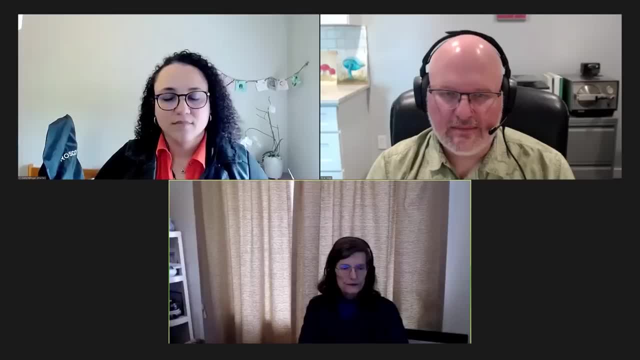 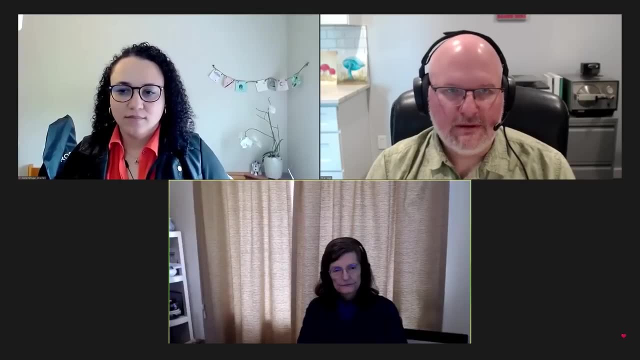 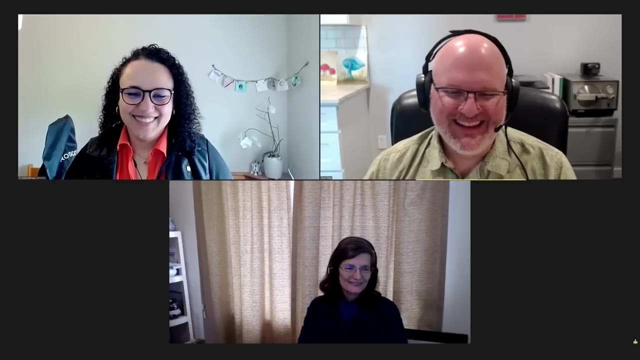 and be able to use it very rapidly to show what needs to be done in your soil so your plants grow better. Yep, Adam, anything else you want to add? I wouldn't be able to add anything to that. Okay, That sounds good. 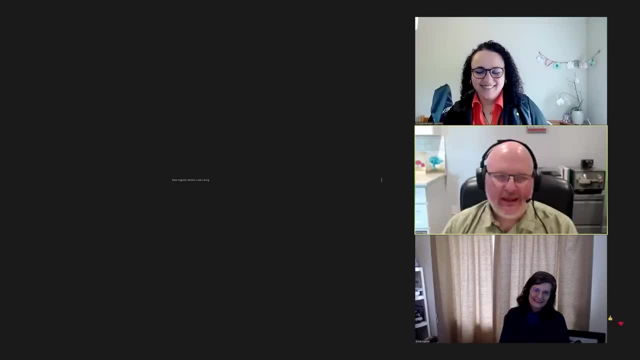 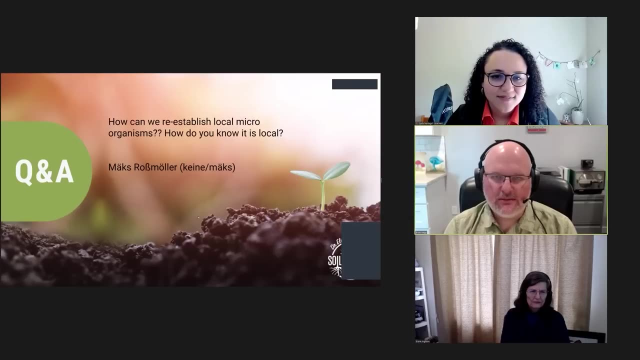 Let's move to the next question, And this question is from Mox, And the question is: how can we reestablish local microorganisms? How do you know it's local? And I think we kind of already answered part of the first question. 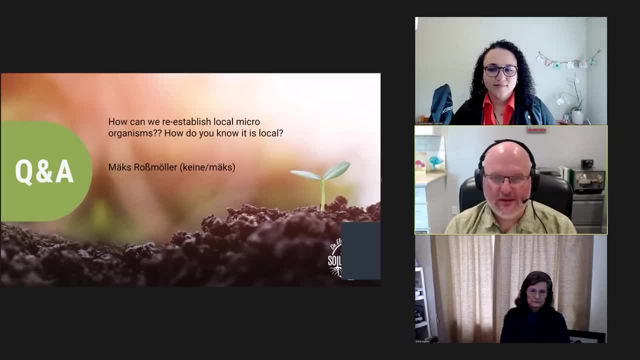 But the second question is interesting: How do you know it's local? All right, We'll take you Pellis. What is local? Yes, that's exactly it. Is it within 100 miles of your location? Is it within your bioregion? 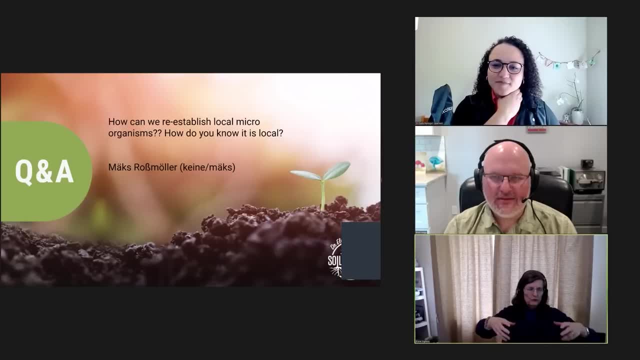 Well, but there are already written boundaries. Now, this is going to be the Yellowstone boundary, This is the biome, And then here's the next biome and the next, And you would go and get your organisms from the To the To the biome, where you want to apply, where you want to grow your plants better. So, and how do you know that it's local? Basically, what I would do is put together a mix of some soils with your compost and put it outside and come back in a couple weeks and find out. you know what happened to the nematodes or protozoa, or the You know what are the species that you have left. We can't. We need to do. It would be really nice if the DNA analysis could catch up to what we needed to do. We needed to do all 13,000 species of bacteria. 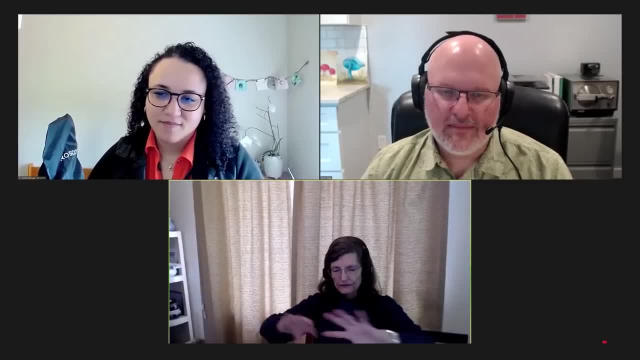 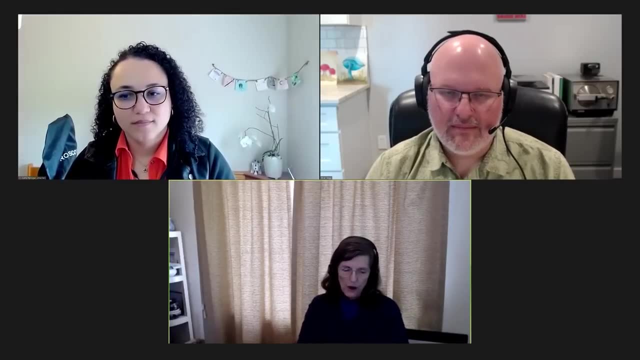 Fungi are a little bit. You can do a lot of splitting the fungi by just morphological characteristics. You can do a lot more that way Before you go on to the DNA analysis. So we need that little tricorder that Dr Bashir in what was the 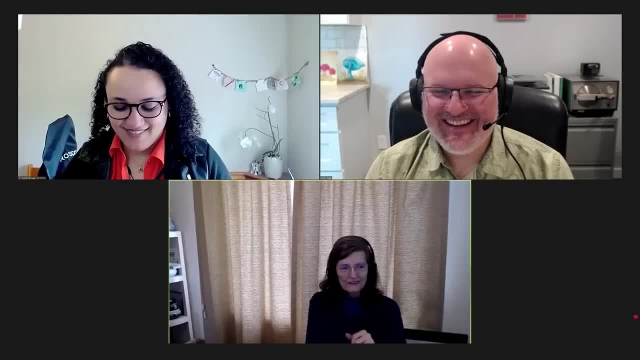 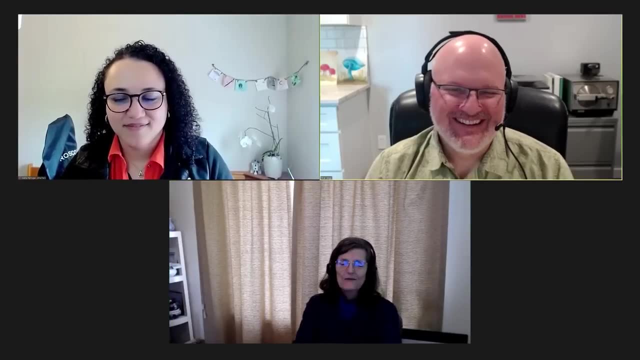 Star Trek. Star Trek would point it at the ground and he'd look at it and he'd say, yes, this has a good ratio of fungi to bacteria in it. Right, I want that piece of equipment. Come on, you engineers, we need this. 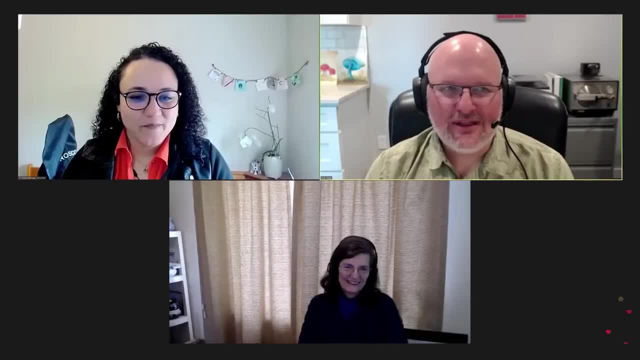 Yeah, There's One part of that question I actually like to just change a little bit as far as the thought thing for the panelists here. A question I get a lot of times is not just, is it local, but what is native? 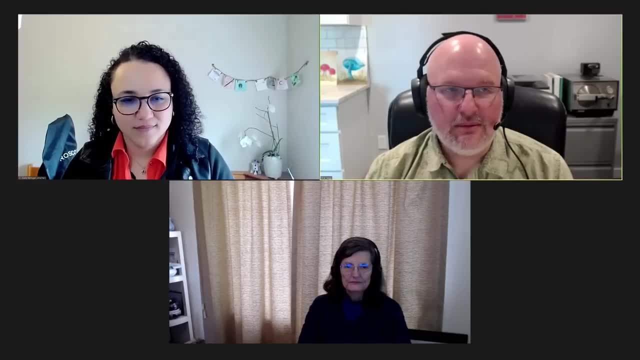 And that is a kind of a fully loaded question. What is your historical reference to what native actually means? Native to a hundred years ago, native to a thousand years ago? Things evolve and change, especially with this whole global kind of network that we have. 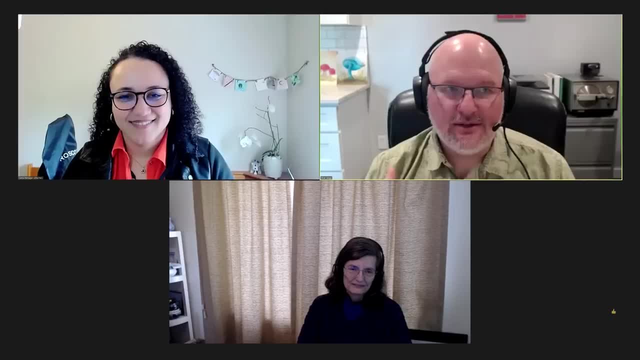 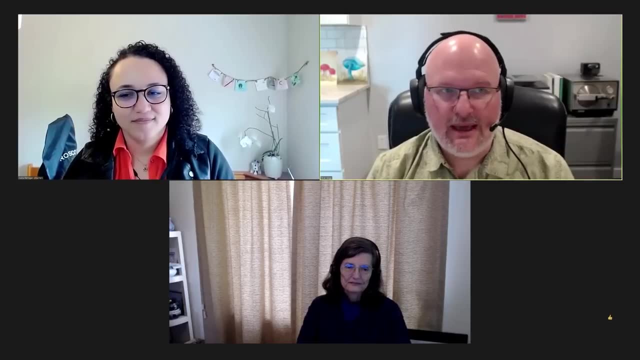 You know what Maybe was never native a hundred years ago, became native now or essentially native-ish, because of somebody moved those organisms into that particular area, And we see that with plants all the time. Yeah, Someone posted a question similar to that in the chat. 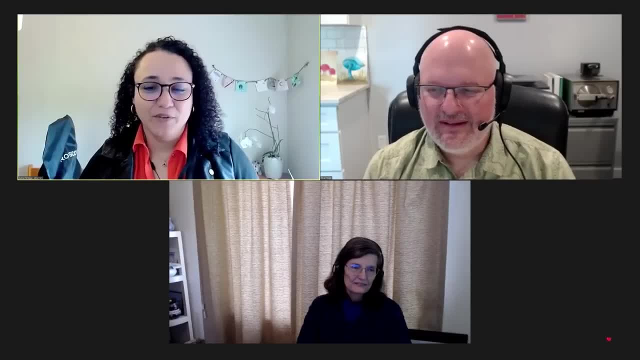 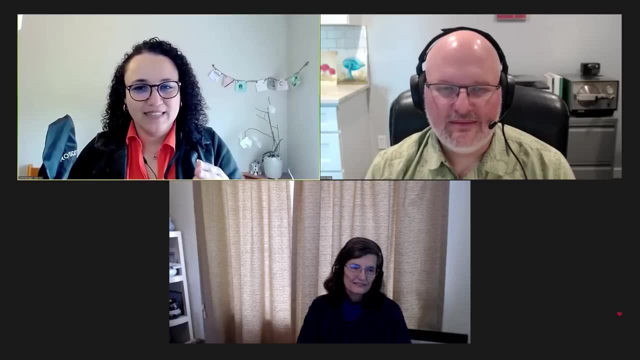 Sorry, I don't recall the name because I'm chatting with a lot of you, but it's exactly that. It's just like how, back in time, we need to go back to define this, because indigenous folks, they domesticated plants, They domesticated plants. 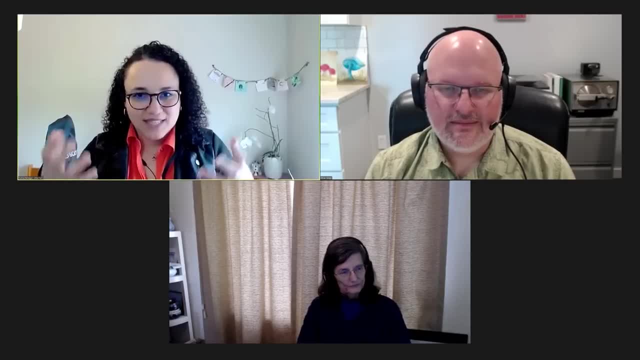 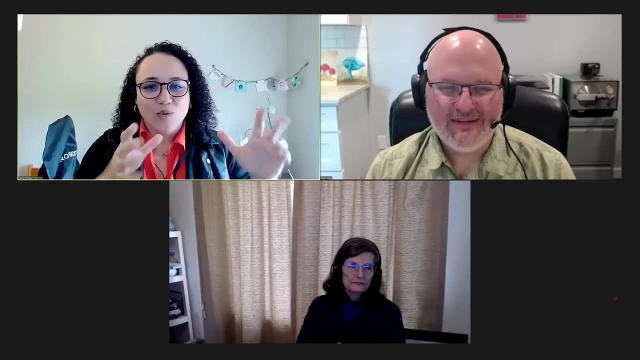 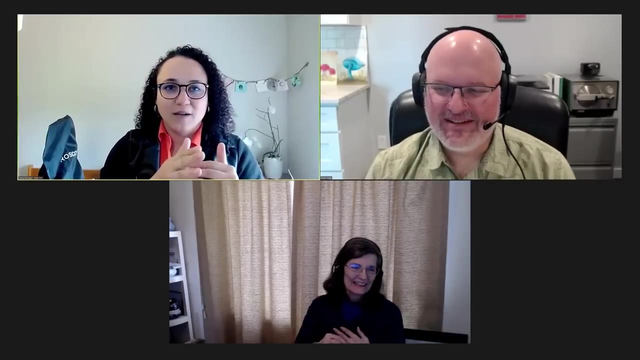 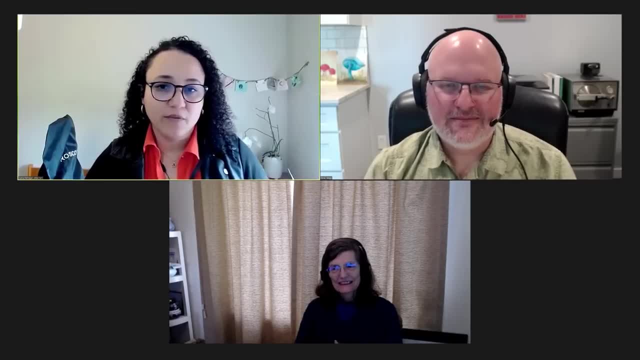 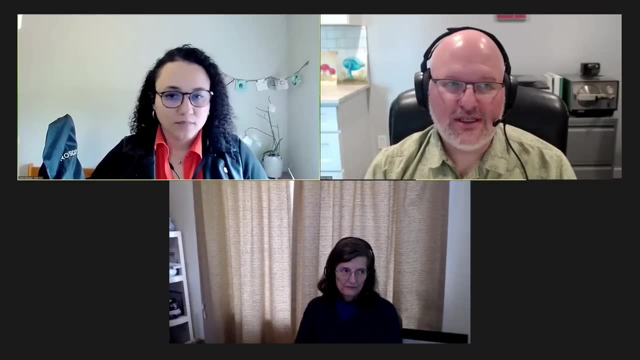 That is always my favorite place to start with. Sure, And it may not have native a hundred years ago, Mm-hmm, But it's now established itself and it's functioning in that ecosystem, I'm sure, And you're not going to get rid of it, right? 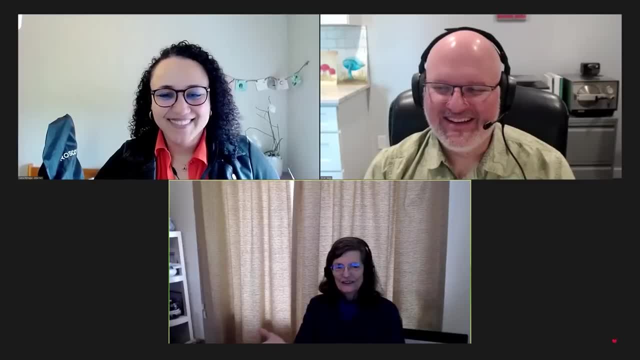 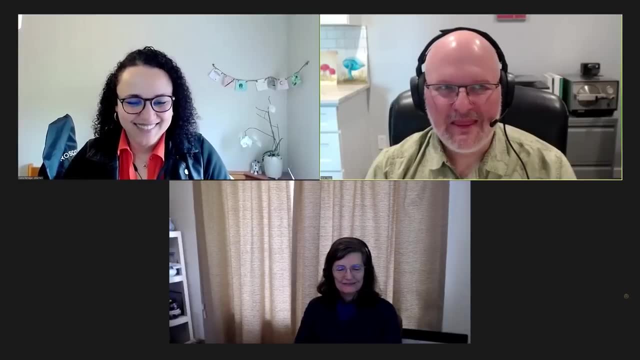 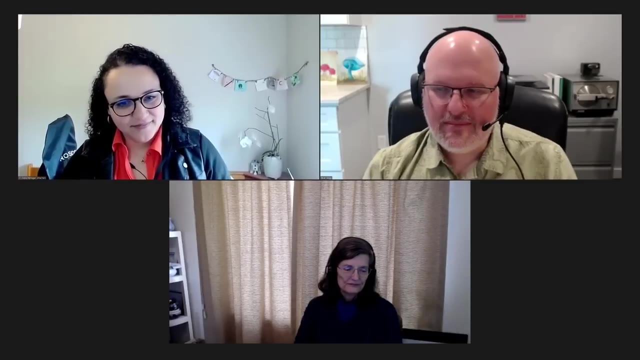 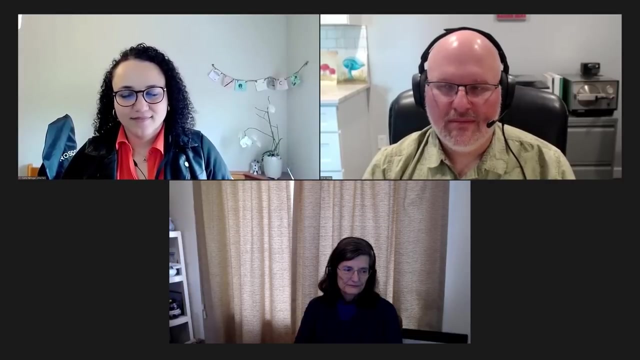 So of it by not you know any method and you just accept that is now indigenous, exactly. yep, i do add one thing about biogeography to that. um, i think about physical barriers between places- mountain ranges, oceans- as a pretty good indicator that organisms in one of those areas may not. 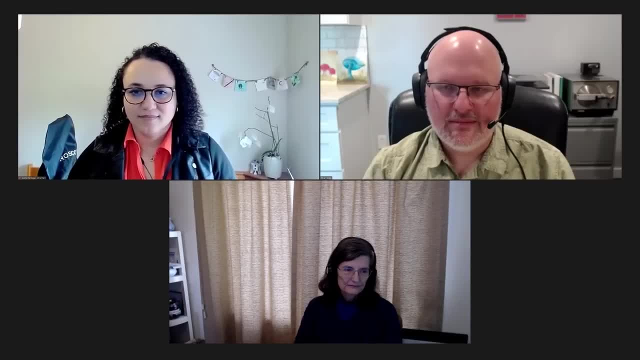 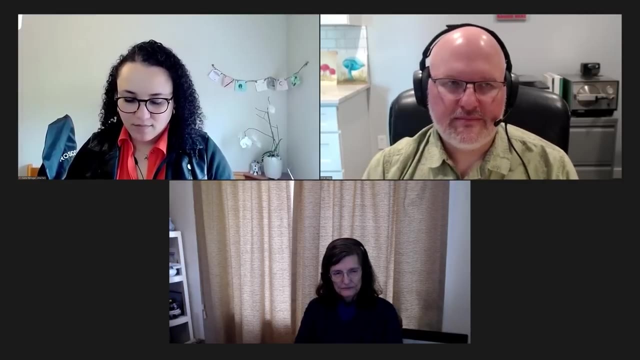 really be compatible with organisms in the other areas, you know, especially if those physical barriers lasted a long time. so many of the most devastating plants that have come over to north america from eurasia are eurasian grasses and they can be highly invasive and and they have. they can be released from the things that kept them in check in their home range. it's not that they're evil, it's that they don't. they, the the things here, did not co-evolve with them because of that big distance and or and that physical barrier, and so you can. 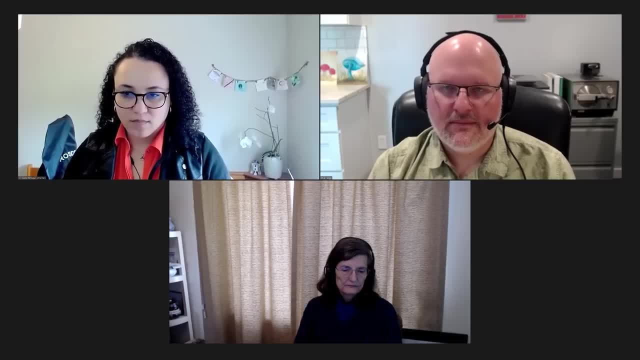 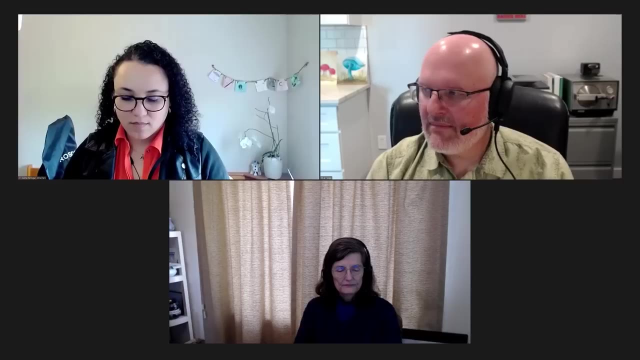 see mountain ranges and other things as potential indicators. um, but elaine has taught us to take a lot of inspiration from the successional stage as well. a lot of agriculture is sort of in a mid-successional stage and if we let it go too late successional, we can actually start to have 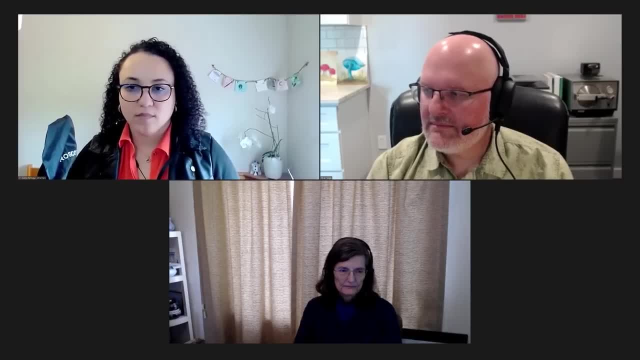 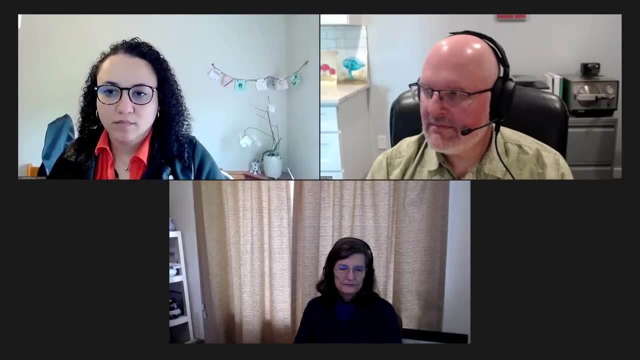 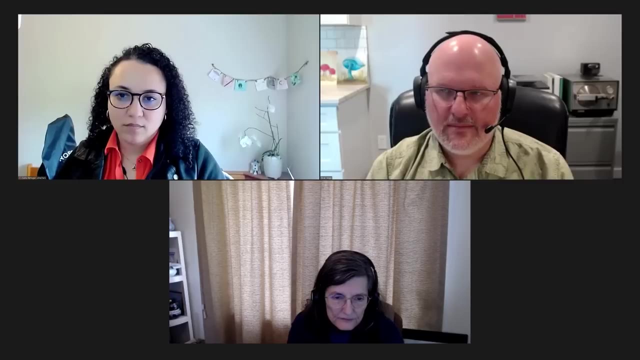 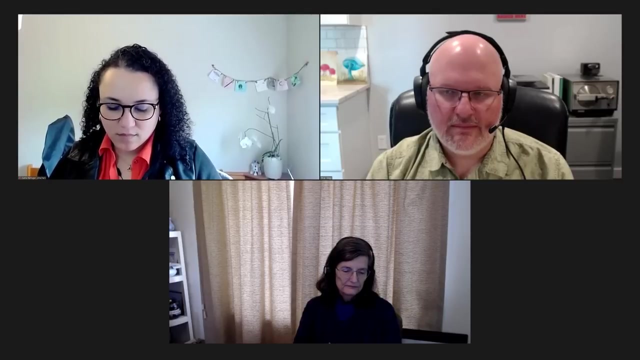 problems, and so it's about having the right. um, you know, even if i would say working in a pasture ecosystem, we think of disturbance as bad, but disturbance disturbances can be very beneficial to keep that fungal bacterial ratio the way it needs to be, or to introduce some diversity in the plant community, and so that's. 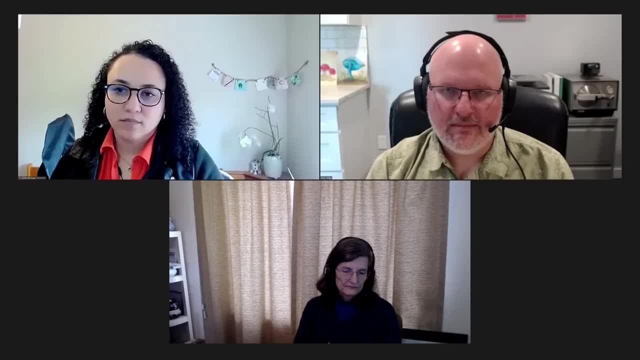 why we often look at fire and periodic drought and grazing as things that too much or in the wrong way can be a true biological disturbance, and so that's why we often look at fire and disturbance. but if managed properly, they can be great. so i think we need to be looking. 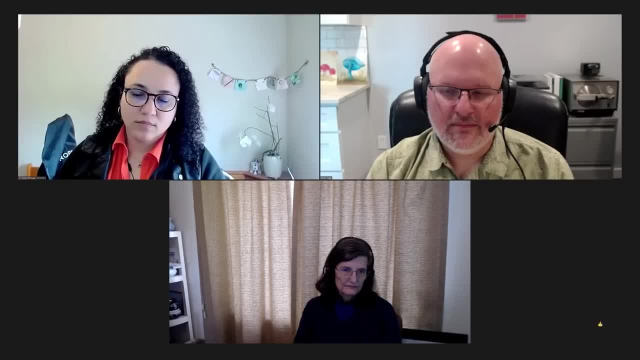 for what organisms are coming from, systems that match the system we are trying to make, and that's very different if you're growing apple trees or grasses or kale. yeah, i like that concept, adam, of you know, using potentially, sometimes like a disturbance, as a management practice. um to 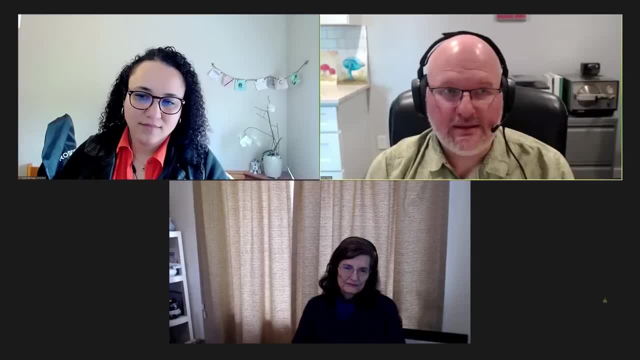 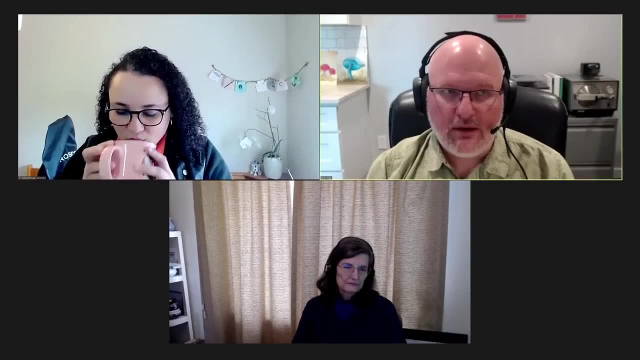 do some encouragement of you know growth, but it's. it's a fine line, and this is where we, as, as managers, have to look at our management practices and really evaluate. are they helpful to the soil biome, are they neutral, are they harmful? and the ones that are harmful we need. 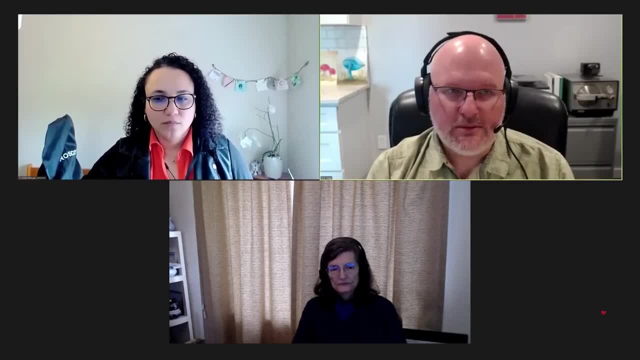 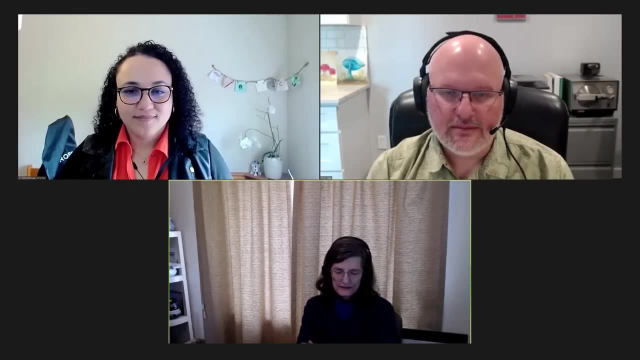 to change those, and then we work on our neutrals until we get our management practices to where we're really benefiting the soil biology, and that's where i i really want to see ground cover um as more accepted than it is right now. um put out seed for plants that are to the best of your. 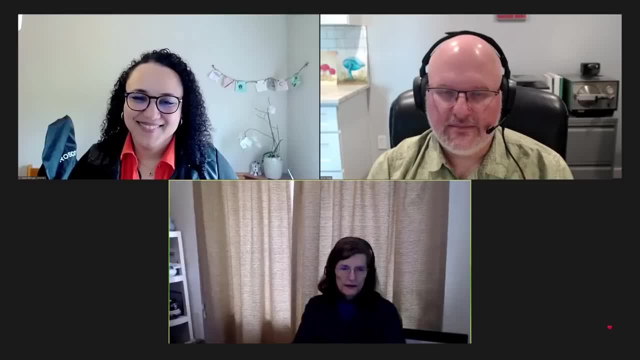 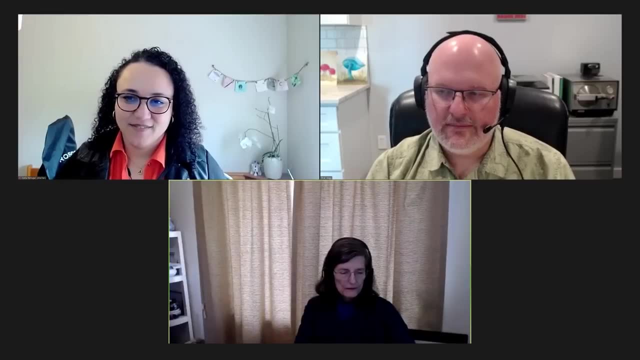 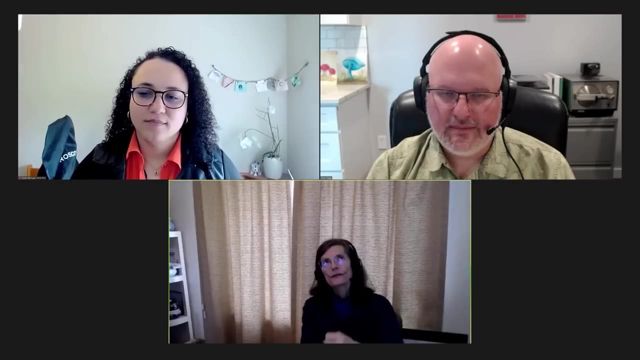 knowledge, indigenous, local- they're going to be able to use the weather patterns in a positive way and get that cover of the soil so that when a drop of water comes flying down, you know, think about how high that drop was when it left the cloud and you know. 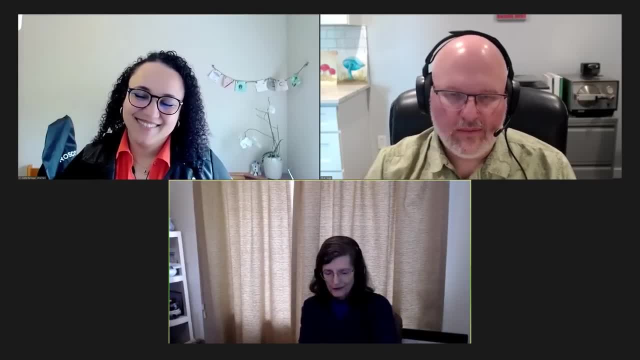 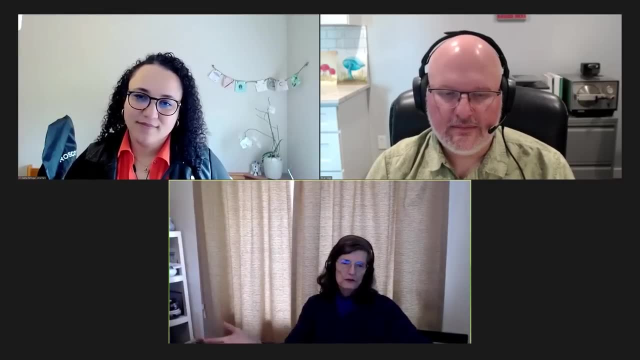 it's going to be significant and it can compact your soil, your um soil surface um, just by having those large range raindrops. you need to have that um soil covered so that when that drop drop of water with all that excess energy comes down, it hits a leaf of that plant and 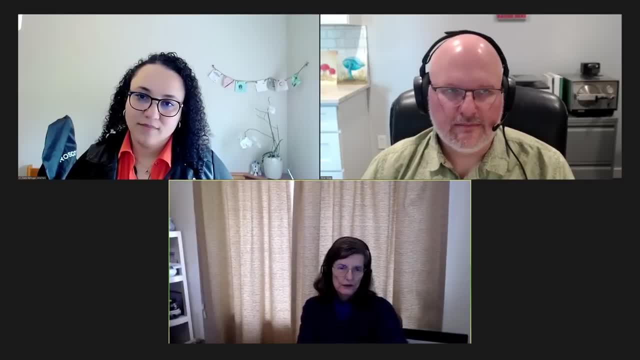